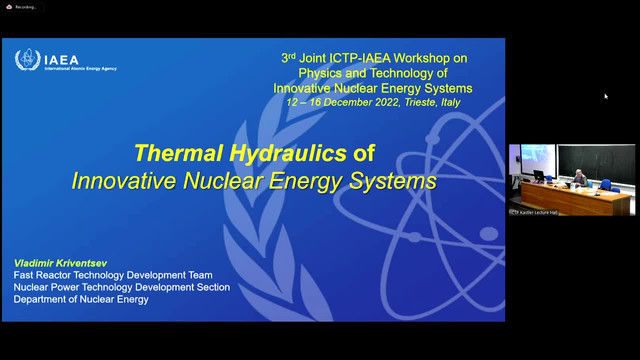 As you know, that we have the thermohydraulics- structural materials And the thermohydraulics- three main fields which should be simulated And of course, we want them to be coupled and work together. But I will focus on thermohydraulics today. 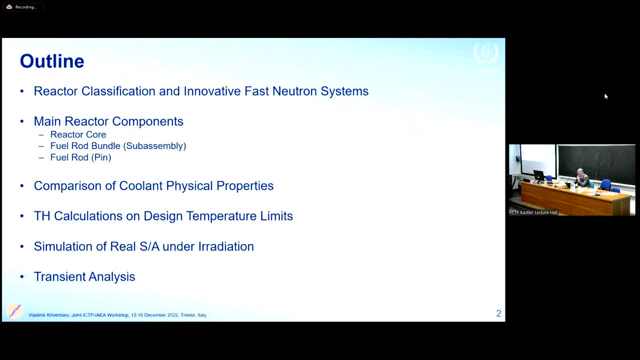 So again, I will remind you some more or less what is innovative fast neutron systems and where is the place of the liquid metal cooled fast reactors here? Then, how to simulate with thermohydraulics main reactor components such as reactor cores, fuel rotbundle. 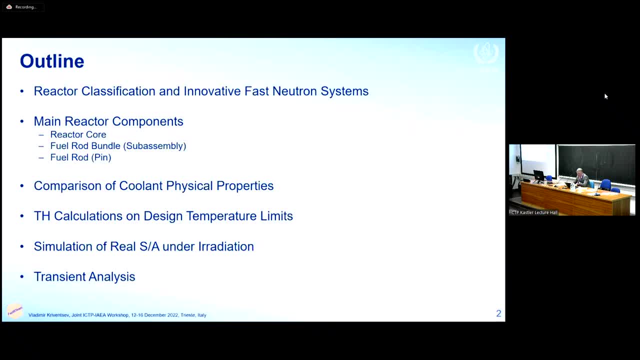 or sub assembly. we call for the fast reactors and also fuel. We'll compare the coolant physical properties, mainly also for the sodium and lead, And I'll give you several examples how to calculate, let's say, these basics of Handbook equations: thermohydraulics, depending on the temperature limits. 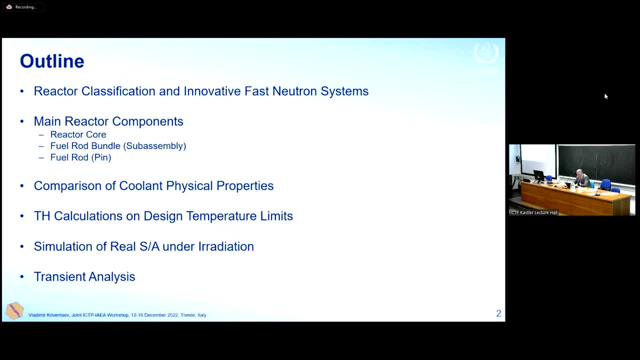 or you want to calculate power or you want to change the temperature limit. Actually, the real thermohydraulic simulations is much more complicated and you cannot cover it in one single lecture. but we will touch this method, which can be used for simulations here, And I will show what kind of difficulties 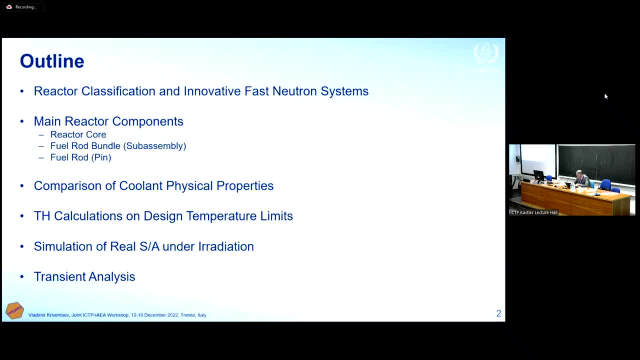 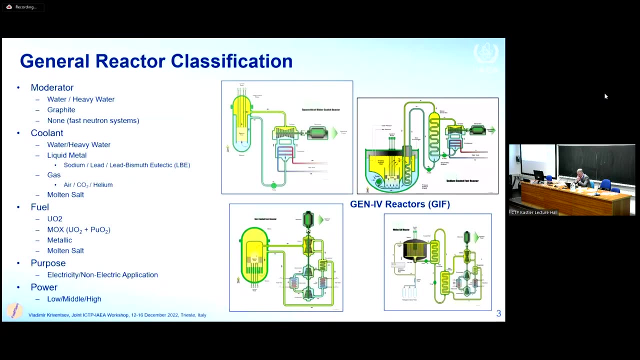 we can face, and especially for transient analysis and how to do also couple simulations, which couple thermohydraulics and neutronics cause simulations. Again, as I already shown it yesterday, it's we classify, just to remind you, reactors by moderator, which can be water. 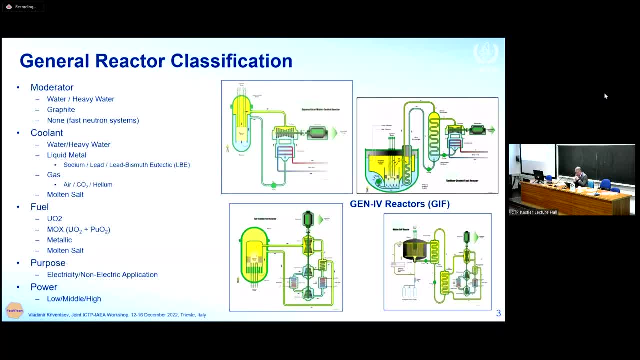 heavy water, graphite or no moderator for the first neutron systems By coolant. again it could be water or heavy water and liquid metals in the sodium or lead, or at least water protective. Also it can be gas like air, CO2, helium, molten salt. 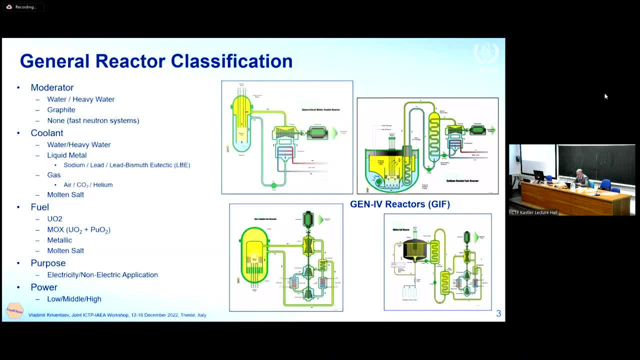 Sometimes we also classify the supercritical water as another, let's say coolant, which is different from normal water and because it has supercritical properties, By fuel. similarly, you can classify reactors like those which are fueled by uranium oxide, or uranium plus plutonium oxide, which is called MOX fuel. 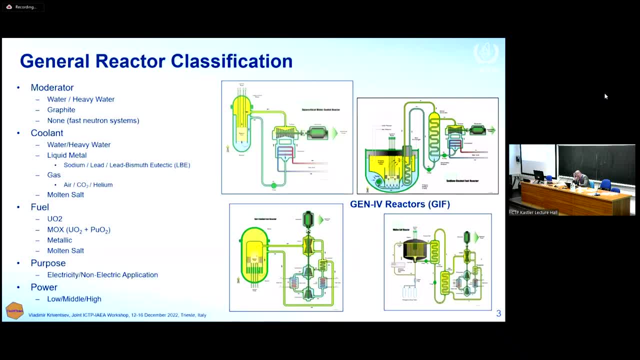 And metallic fuel is also possible, and molten salt also. There are several modern types of fuel like hybrid and nitride fuels of uranium Also. we don't touch here, but there are, Let's say, future or, for example, thorium cycle. 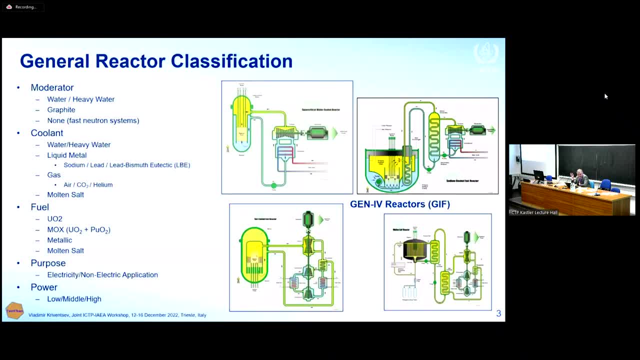 It's used thorium fuel, which is actually not fuel but breathing material, but we will not touch here. This is type of fuel which I used already in the reactors, existing reactors. By purpose, reactors can be classified for electrical and non-electric. for generation electricity: 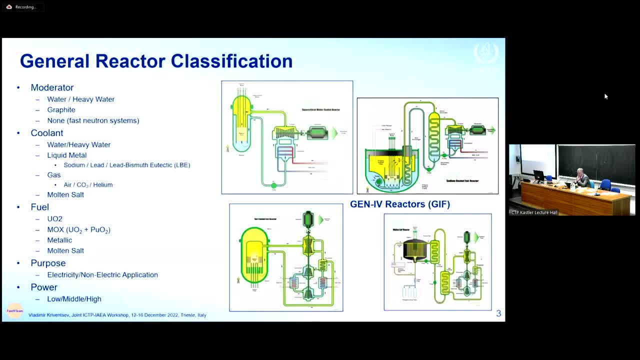 and for non-electrical applications: hydrogen production, desalination, heat heating, etc. This is the type of fuel that we use- district heating, et cetera, and also high temperature heat for the industrial applications as well. Power of the reactor can be low, medium or high. 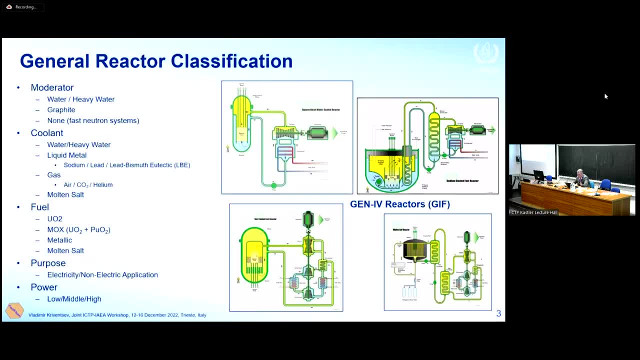 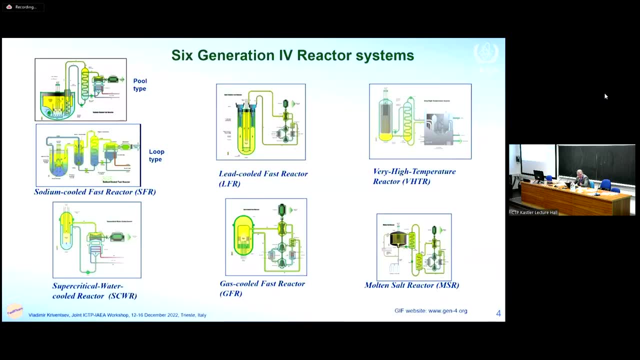 And for this we have classified also SMR small and medium sizes on all modular reactors. Already I touched this, but maybe you'll give more extended explanation about the six generation four reactor systems, which includes sodium-cooled fast reactors, both pool and loop types. 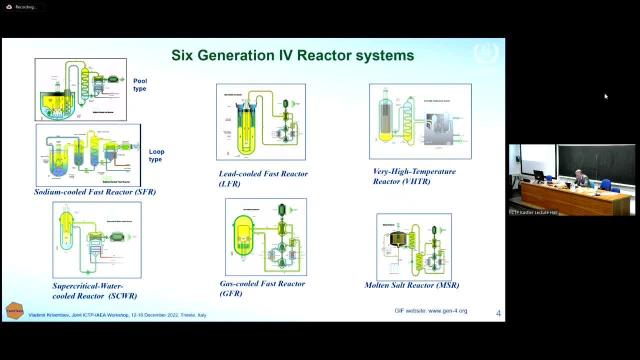 lead-cooled fast reactors, very high temperature reactor, supercritical water-cooled reactor, gas-cooled fast reactor and molten-solar reactor. Of all of these six, only very high temperature reactor, VHTR, cannot work. It can work in a fast neutron spectrum. 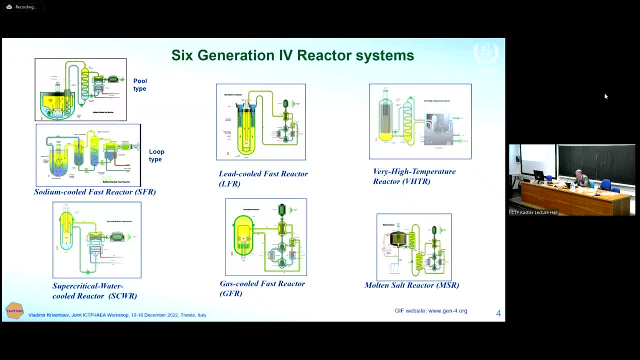 while all others, including molten-solar, can work both in thermal and fast spectrum, And supercritical water-cooled reactor can also work in the fast spectrum, both in thermal and also intermediate. So just to give you an idea, most of the generation. 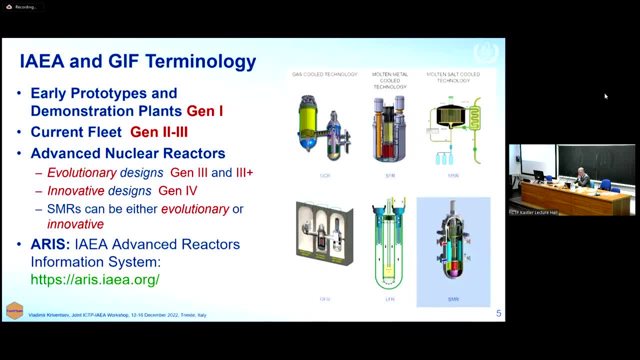 four systems are fast reactors. Again, there is usually confusion with terminology when We say generation. why GIFs say it's generation four? because we had they classified actually three previous generation. First generation was early prototype and demonstration plants. Current flint is the second wave and the third wave. 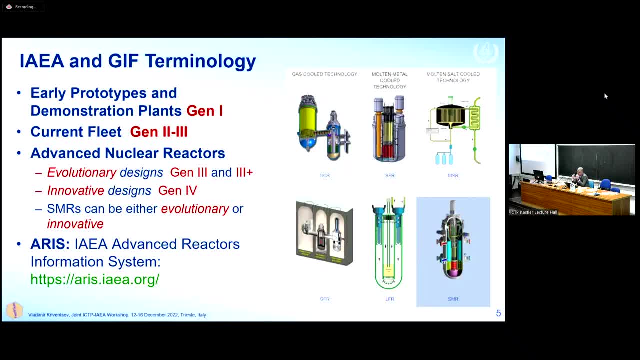 More or less or half of them. approximately half of the modern reactors are generation three And another half is old Flint is generation two, so-called. There are several advanced reactors, both, I mean especially water, what we call evolutionary and innovative. 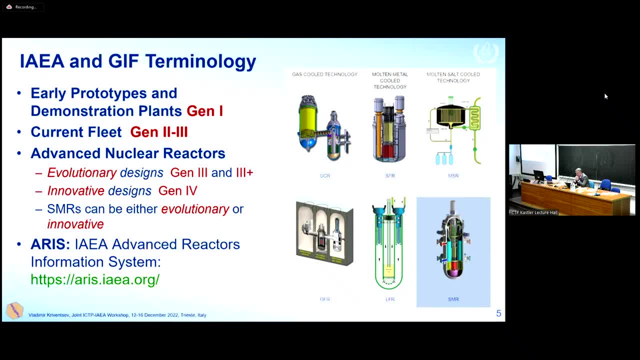 So evolutionary is more or less generation three, and generation three plus designs, according to the GIF terminology, And innovative design are generation four. just notice it there. So again, just notice that these generations are static classification, While in the IAEA we use this evolutionary and innovative. 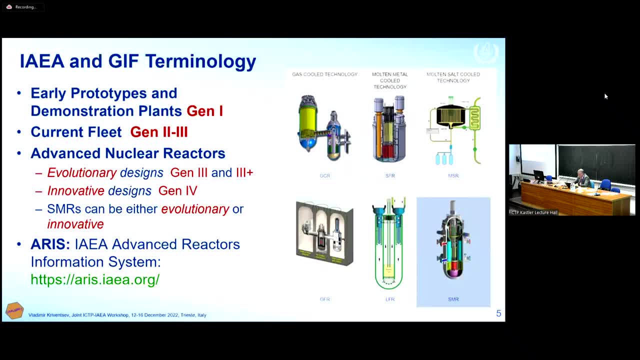 for all advanced reactors, which are relative classification. So what is innovative today could become evolutionary or old technology tomorrow and the day after tomorrow. SMRs, which are very popular and attracts a lot of attention nowadays, can be also either evolutionary or innovative. 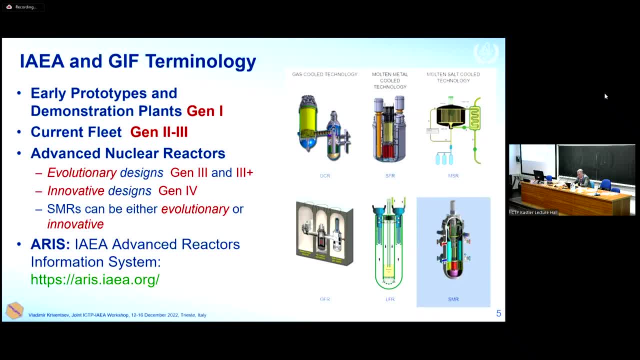 means either generation three or three plus or generation four, So we can say that these are the two most advanced reactors. Here there is something missed, but this is terminology which is developing and you don't have to. We have this IAEA- Advanced Reactor Information System, ARIS. 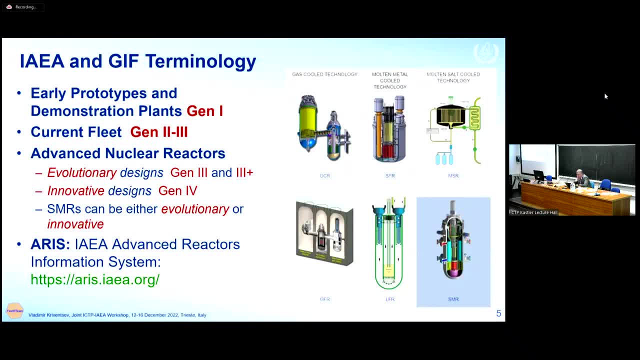 which collects all possible reactors, advanced reactors, both evolutionary and innovative, And we can find all information about these advanced reactors as they are provided by IAEA. We don't check, We don't, of course, evaluate or assess what the designs. 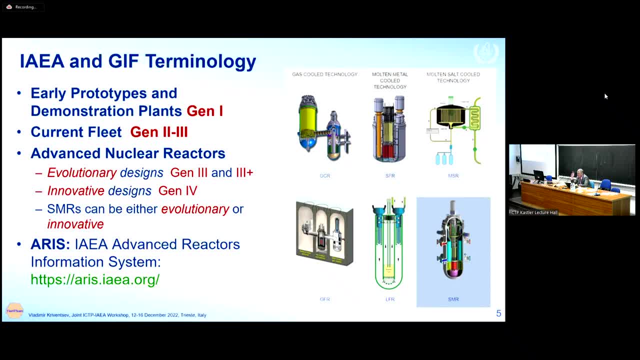 We try to just to remove if they use this commercial or advertising the designs. It's not allowed. But from the other points, all information provided are provided by the designers and vendors And of course there are many. I know how many it's maybe. 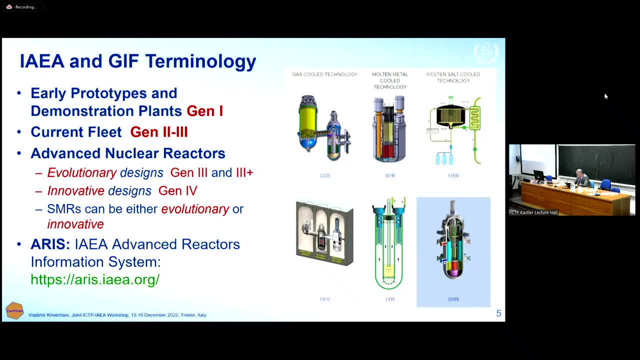 about 80 or even more designs. I don't I forget now In this data, But of course we don't expect that all of them will become a reality. As Akira explained it yesterday, that of many things like, if you look at the markets, the car makers we have OK. 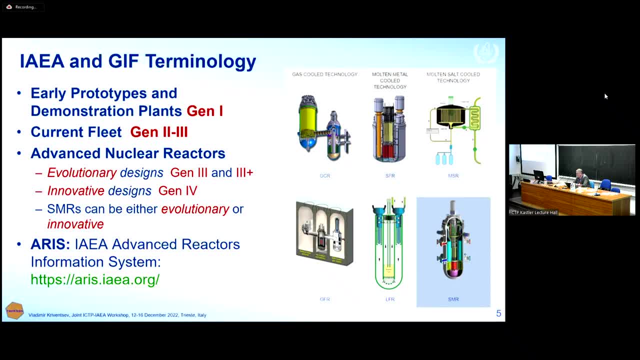 For car makers, we have like maybe 20 at least who are producing. But if you look at the plane aircraft makers, it's for the civilian fleet. it's only now The big one as a Boeing and Airbus. this only two. 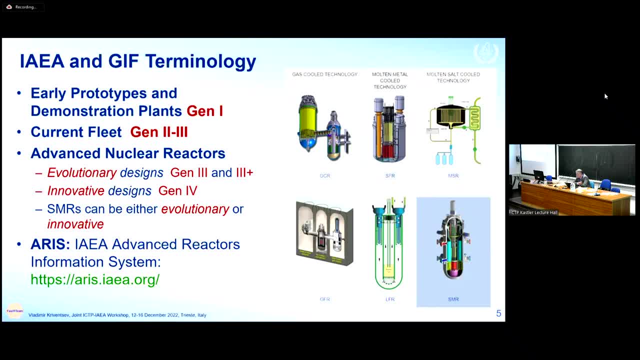 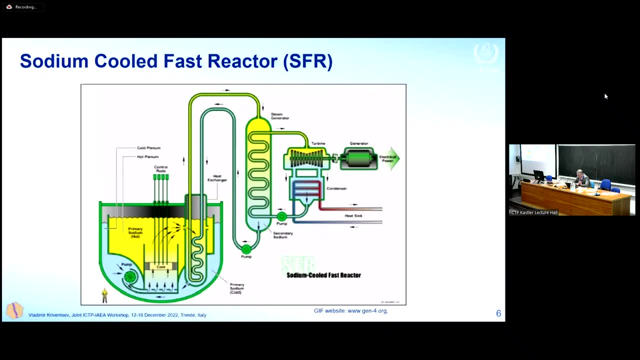 So don't expect that we will have all 80 designs there, But some of them, I hope, will be. Which one? you never know, It's future will decide. OK, So sodium-cooled fast reactor: is technology that this is has already very mature, because it's we don't know. 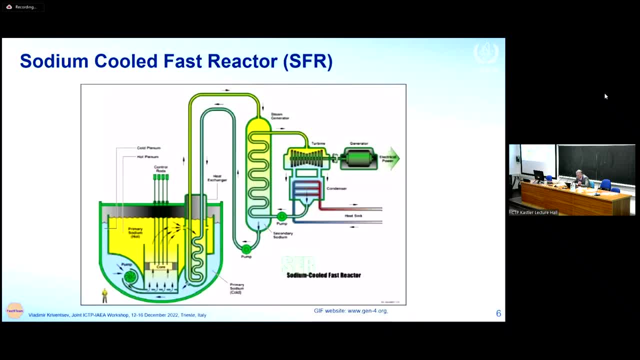 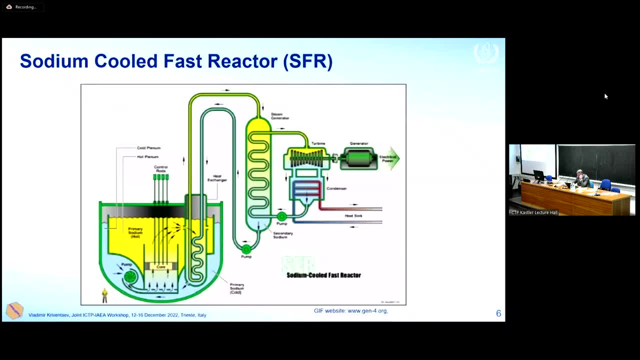 Because of this, sodium is a perfect- I would say would be perfect- coolant, But there is a disadvantages very important. Sodium reacts aggressively with water, as you know, and also with air. It starts burning in the air without any ignition. 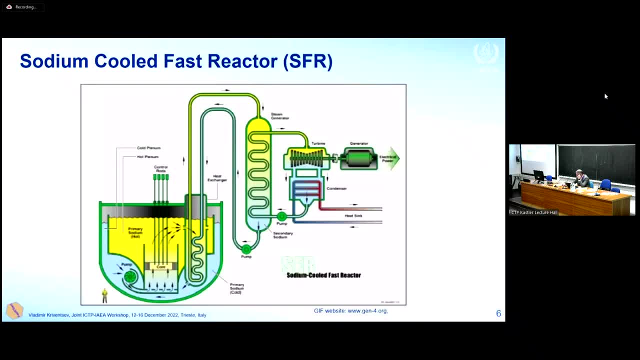 For these features of sodium coolant. Dr Laje will explain us in his lecture and he knows much better and he has great experience with sodium. but I think, Christian, you can agree that sodium is the best coolant you can imagine. 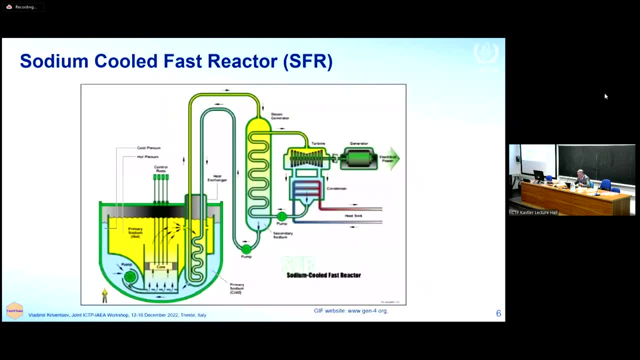 Thank you for confirming, But for this the system becomes more complicated because we need intermediate circuit between the primary and secondary circuit, which goes to separate radioactive sodium from water to exclude this direct contact. Of course it also could be included in the secondary circuit. 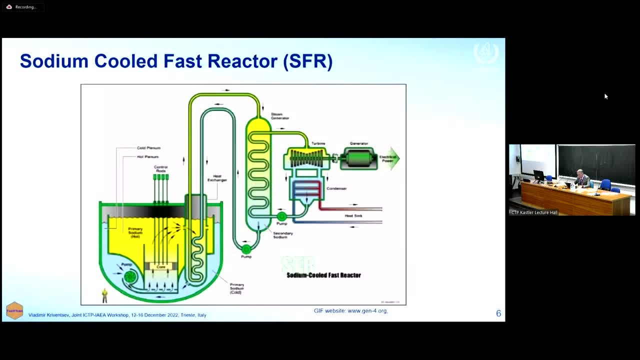 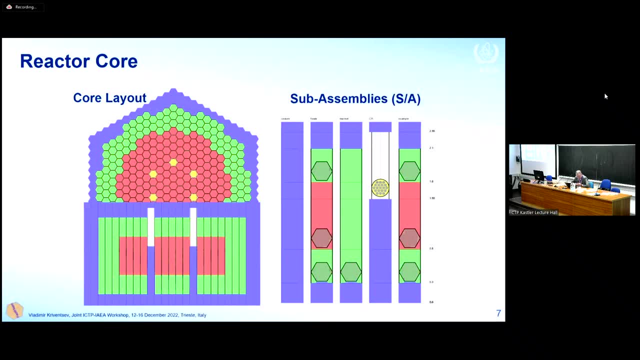 but we want to exclude and then make the system more expensive. This is the thing. Okay, this slide shows the typical. Now let's go to the thermohydraulic simulations of the reactor. Okay, reactor core consists of the several sub-assemblies. 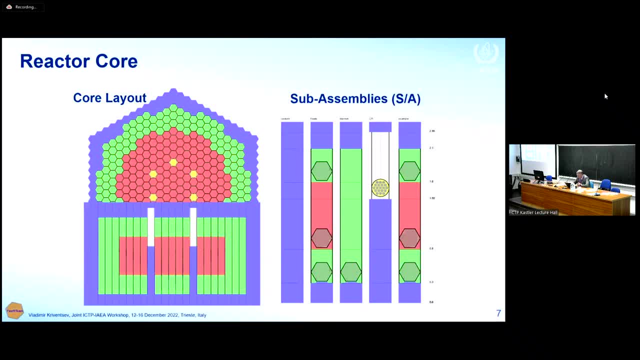 which maybe you, I guess I will show you. Maybe let's start from and this is the- if it works, okay, This is the core layout from the plane cross-section and this is the cross-section in the axial direction. 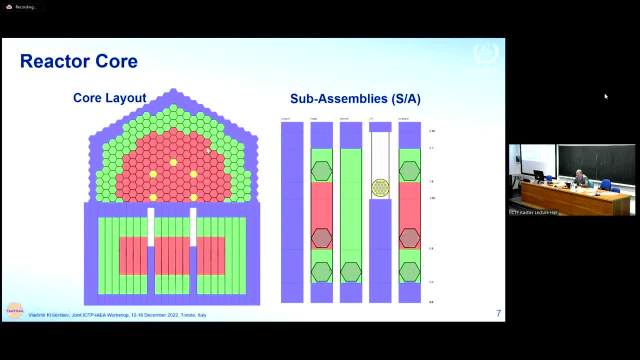 and this is red, yellow, blue and green. so things we call blocks we call sub-assemblies. In case of the traditionally for the fast reactors- sodium-cooled fast reactors- we call it sub-assemblies, while for the water reactors 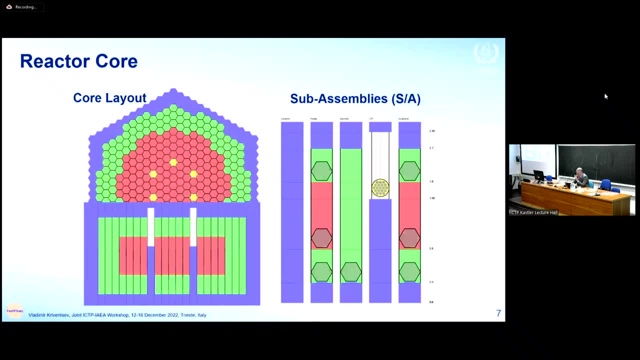 those elements are called rod bundles also. So sub-assemblies construct the reactor core which you have when you have critical mass and then you have a reaction and then the heat is released in the fuel and removed with coolant from this reactor core. 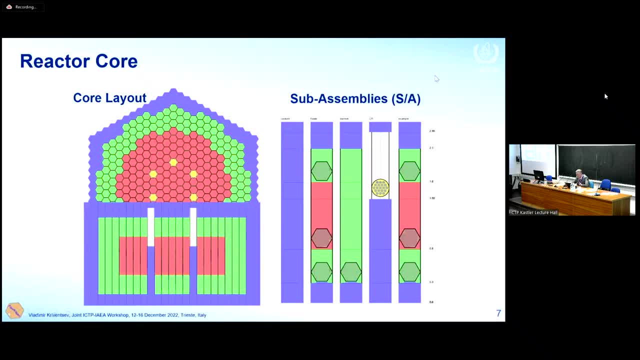 Sub-assemblies can be different types Here. example of traditional example of the hexagonal sub-assemblies which are usually for the all fast reactors are hexagonal shape. For water reactors it could be also hexagonal or also square shape typically. 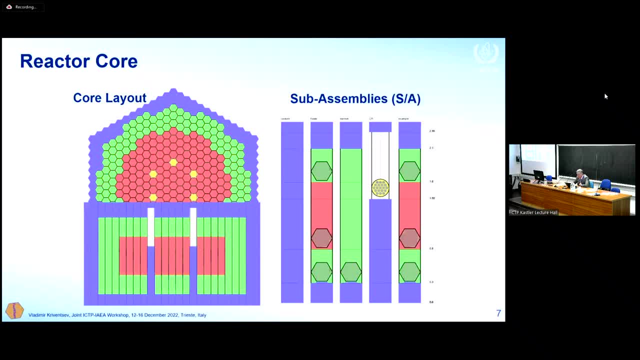 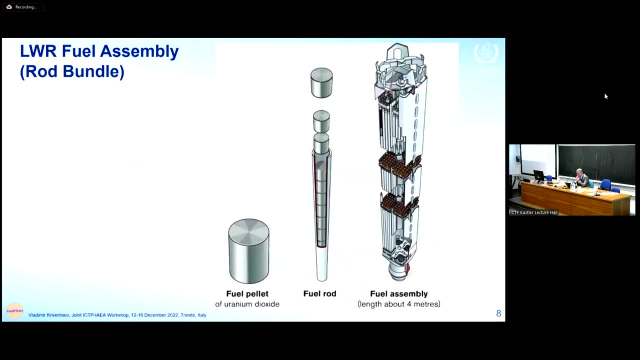 and inside you could see array of the rods, or pings, again for the water reactors. it's called rods, for the fast reactors, Somehow these fuel elements are called pings. just to show you one example of the fuel assembly: 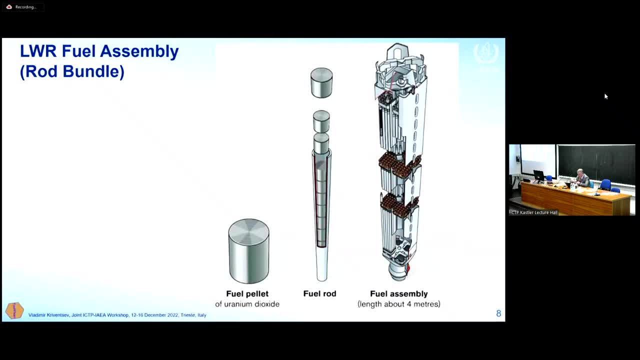 of the light water cooled reactor. So these pellets are collected and inserted inside the fuel fuel rod, and fuel rods are inserted in the fuel assembly which is length several meters, four meters for example in this case, and this is one of the possible design, as I said, it not necessarily hexagonal but can be also. 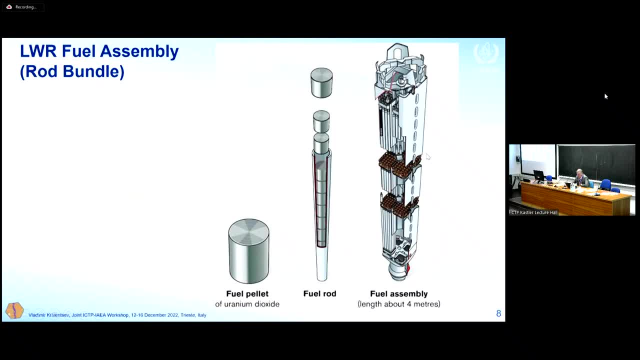 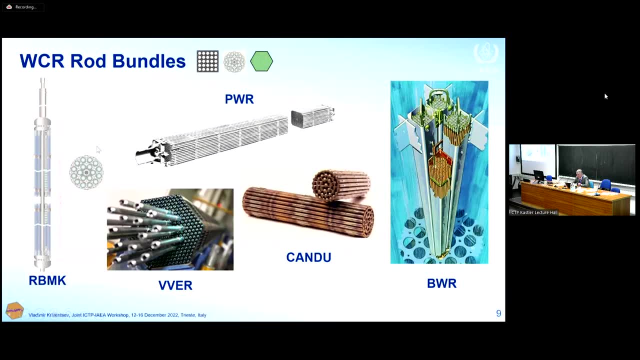 square. if you, let's say compare, is this: this for the boiling water reactor is square, for the pressure is right. for tractor it can be square. for the Russian river it's already hexagonal- not square, but hexagonal. also shape, but still it's a big rods or we call it in this case, field, in this palace, inside, for the. 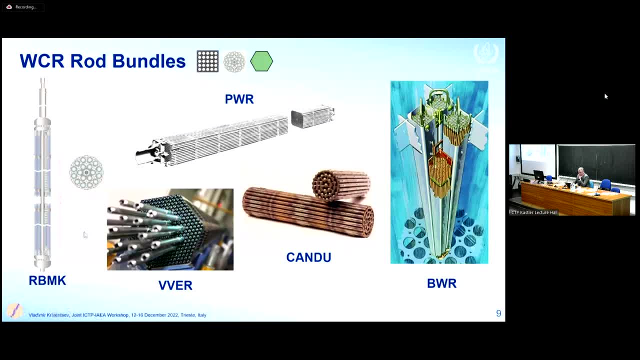 graphite moderated reactor, Airbnb, also the Russian Soviet Union's and Russian design- you have some assemble is of this system size and it's not, let's say, hexagonal, not square, but cylindrical. cylindrical shape which is inserted inside the channels we graphite inside the graphite moderator for the can do reactor which is in the horizontal, the sub assemblies. 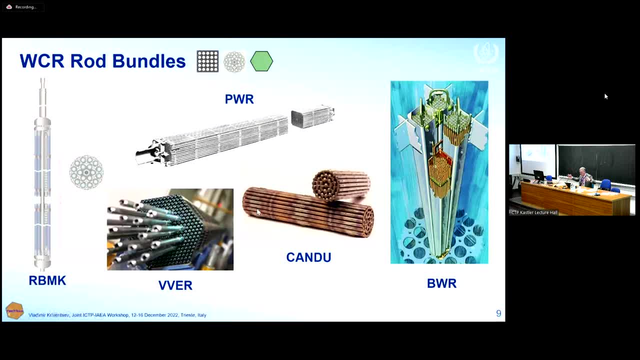 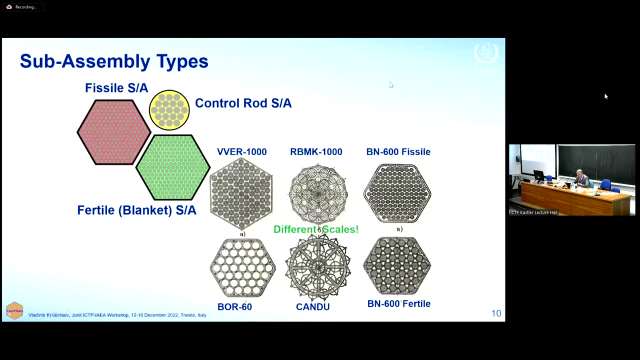 this. of this I know one meter or one meter size blocks that are collected in horizontal, horizontal layer. so what we can see, we can have here as a square road bundles, cylindrical on bundles and hexagon on bundles as well. all they are used for the designs. again, it's also this sub assembly types and bundles which can be. 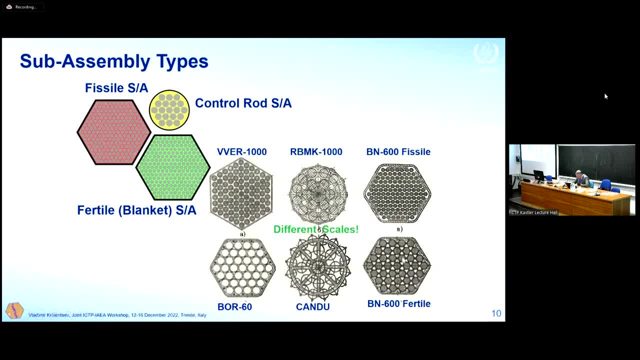 of different shapes here. it also compared several hexagonal design for the VVR-1000,, RBMK-1000, and then with sodium-cooled fast-reactor BN-600,, let's say with fissile and fertile material. Fertile means breathing material. 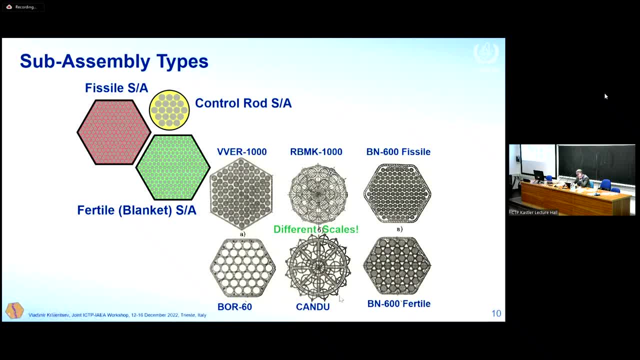 in this case uranium-238.. This also shows the cylindrical shape of the CANDU reactor and also hexagonal of BOR-60.. Actually they are different scales so you shouldn't compare it directly, as it is The different scales at just this slide. 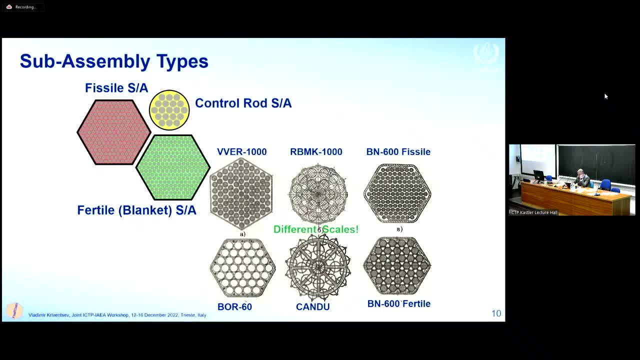 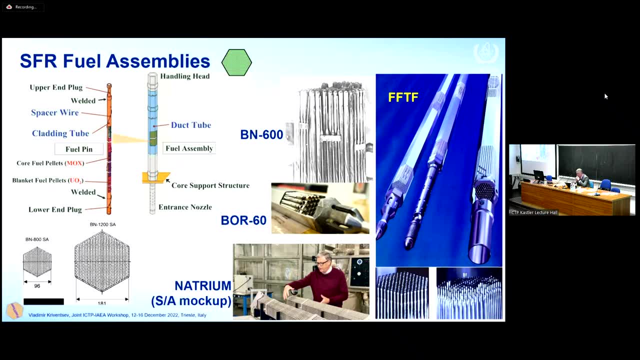 shows you the possible geometries. possible geometries: Okay for the SFR fuel assemblies. now let's go to the fast-reactors and sodium and heavy liquid metal-cooled fast-reactors. We have this fuel assembly, which is typically hexagonal shape. 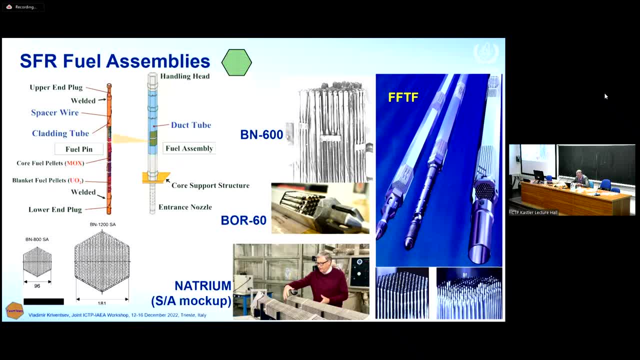 but, frankly saying also, square shapes were also considered for the lead-cooled reactors one time, but usually the typical shape is hexagonal And because of this tight allocation of the pins usually we cannot use grid spacers, like which is typical, to separate pins. 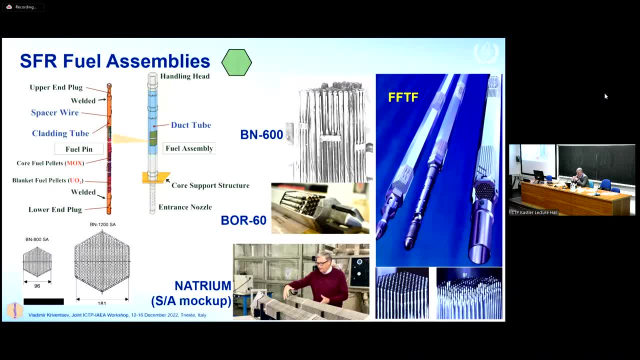 as is typical for the water-cooled reactors, but we use wires- tin wires, which is rotated around the pins, and then this wire separate pins to be touched and to overheat and to increase the temperature. So we need to provide the best cooling possibilities also. 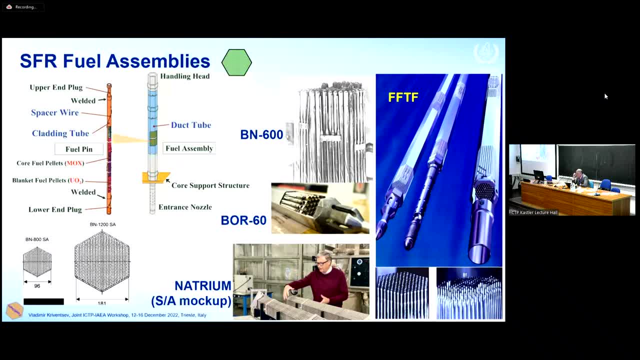 However, in principle, also for the lead reactors, where it has a bigger volume fraction of lead, you can also use grid spacers. Okay, So you can see that the tin and brass 300, it's grid spacers are used instead of the wires. 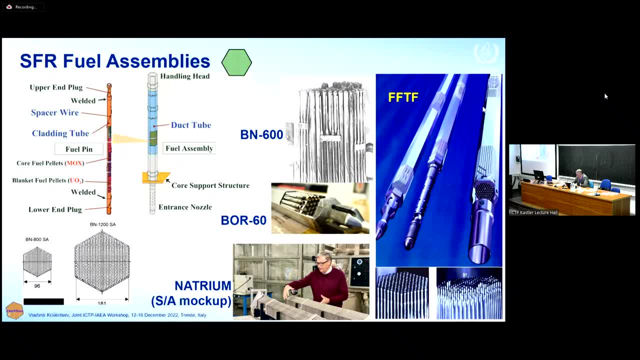 You see here that just I tried to find out in the open literature the photos of the possible fuel assemblies which look very similar. Hexagonal collection of the pins You see is the newest, let's say, natrium reactor presented by Bill Gates. 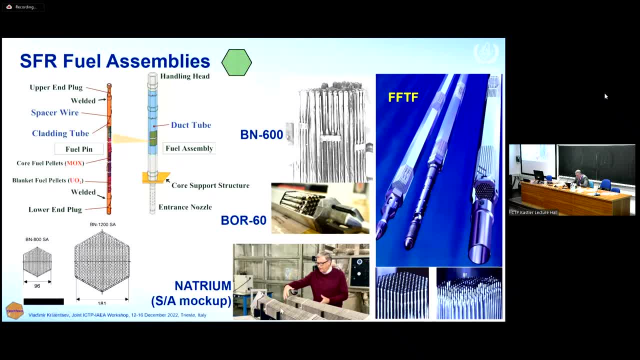 actually by TerraPower, but he's also standing here. This is actually experimental mock-ups of the fuel assemblies, but you can see, compared with Mr Gates, the size of this sub-assembly and how does it work. They could be different, of course, sizes. 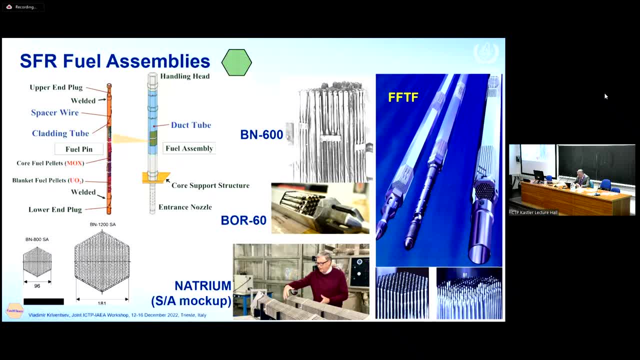 It can be smaller, like 96 millimeters, or even like 18 centimeters or so. Different different sub-assemblies for different types. Sometimes they are not covered, so there are gaps in here In hex scan, what we call hex scan walls. 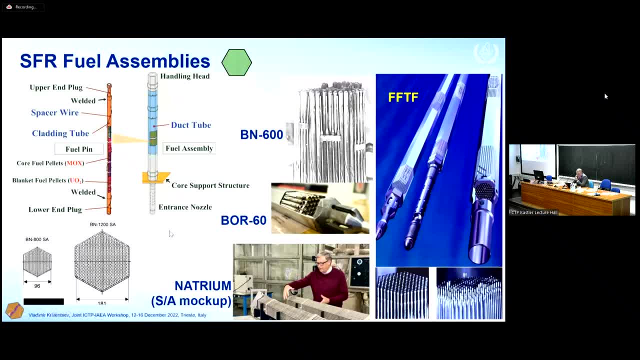 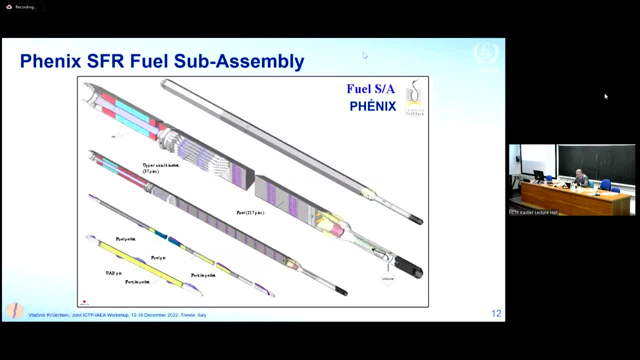 or without wrapper also, it's also possible. This is the sub-assembly of the Phoenix sodium pool fast reactor, which was long in operation and provided a lot of experimental data in France, And Christian was actively participated in this work and I will leave also for him to explain the details. 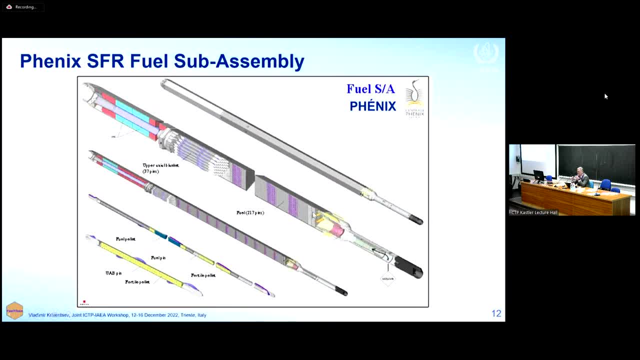 It can be very complicated. Basically, this is a sub-assembly hex scan channel with inserted fuel pins, but also other elements. For example, here you can see the so-called blanket where this could be uranium-238,, which is breathing material. 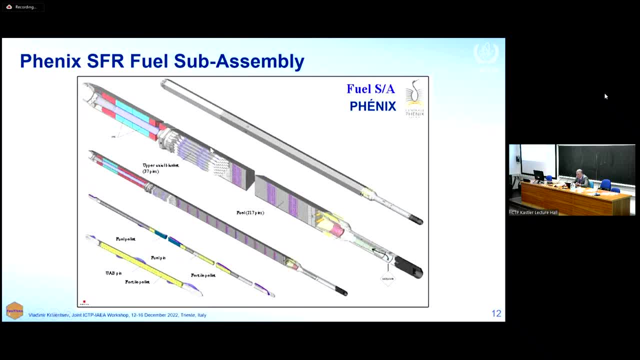 which is converted to plutonium-239 during the breathing in the reactor. So you have those pins are thicker the diameter compared to the normal, normal for, let's say, small 6.9.. Here we have 217 fuel pins and 37 only pins. 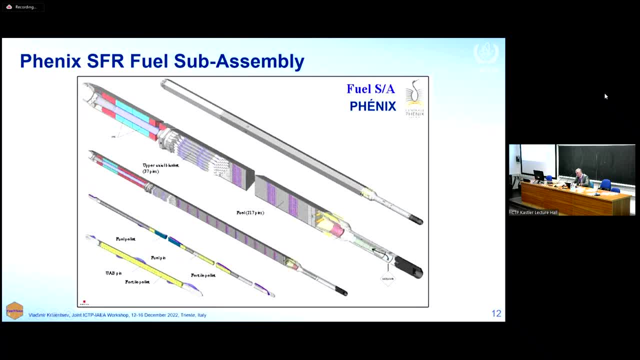 in the breathing area, but this is connected in the wall- one sub-assembly, And that okay. all these elements release heat and coolant flowing through all the system removes this heat. And the purpose of the sodium-hydrolysis system- the sodium-hydrolysis calculations. 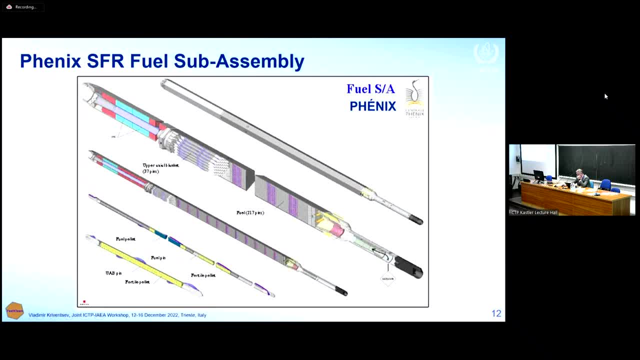 it is to calculate how this heat is removed, what is the temperatures, what is maximum temperatures of all coolant cladding fuel and how to optimize this, how to reduce the maximum temperature or, from the other side, how much we can increase the power. 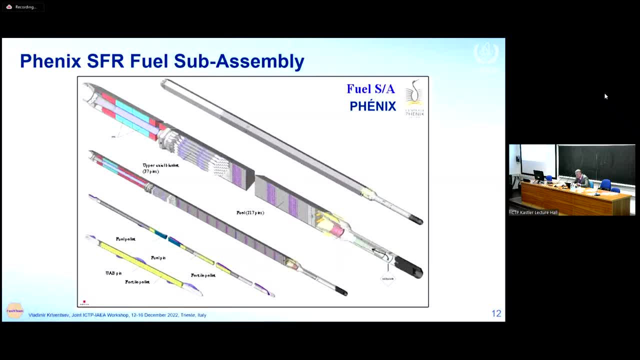 of this sub-assembly to not to exceed the temperature limits which are given actually by the people from Structure and Materials. They provide us upper limits. Let's say, temperature of fuel should not exceed the melting point, but it's okay extreme. 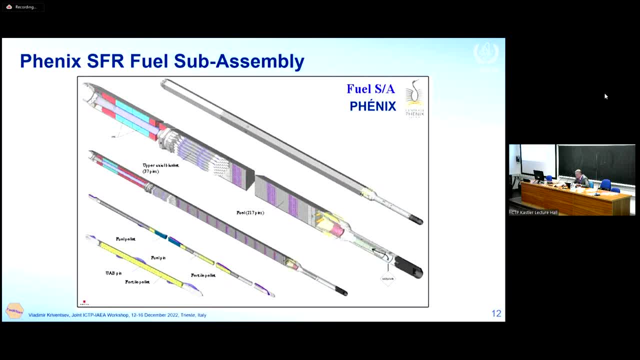 For the coolant temperature should not in principle exceed the boiling point of sodium- never, let's say, But of course we should not be close to this limit, We should have some gap to be on the safe side. And also for the cladding temperature should not exceed 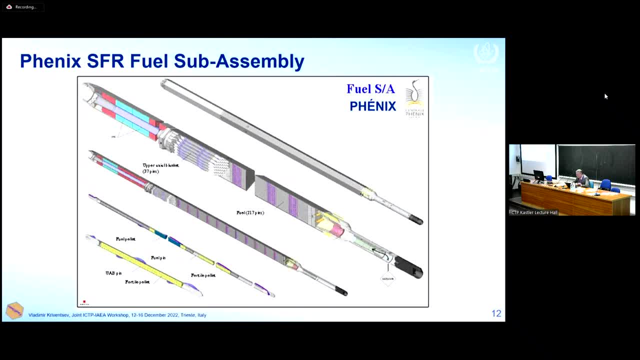 of course, the melting point of steel, but also should not exceed, I know, 1,000, temporary, even 1,000 degree Celsius, because steel can not survive even in temporary of this, Or in the long term. should not exceed 700 degree C. 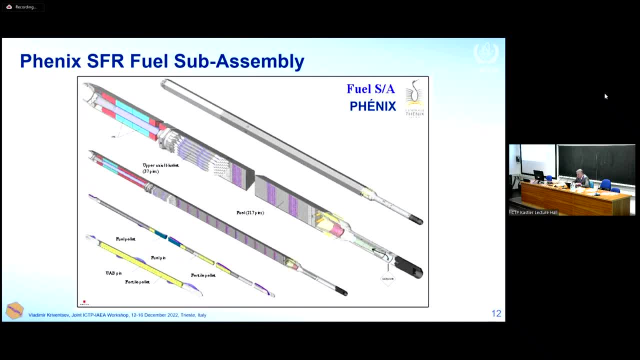 for the steels because of, in case of irradiation, steels are not. I mean for this case. they are not, I mean for these conditions. it's a problem. We can have a problem with steel, with swelling. 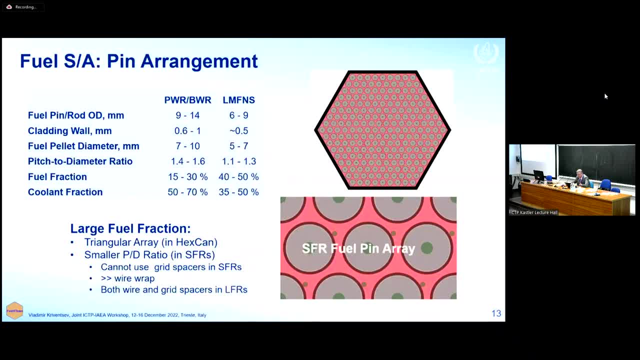 and other things with steel as well. Okay, so if you compare as a pin arrangement- and this is defined, of course, geometry, by this pin arrangement, If you compare here the between pin arrangement between pressurized water reactors, boiling water reactors, 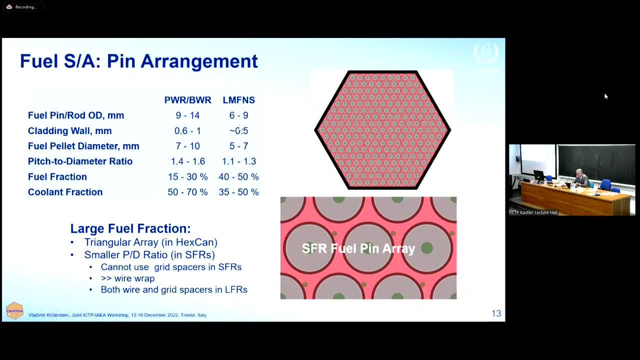 and liquid metal fast neutron system. you can see okay, liquid metal- here is more or less sodium- cooled faster. So the fuel pin or rod is much bigger for the water reactors Cladding. also, wall thickness is smaller for the because we want to keep it as the materials. 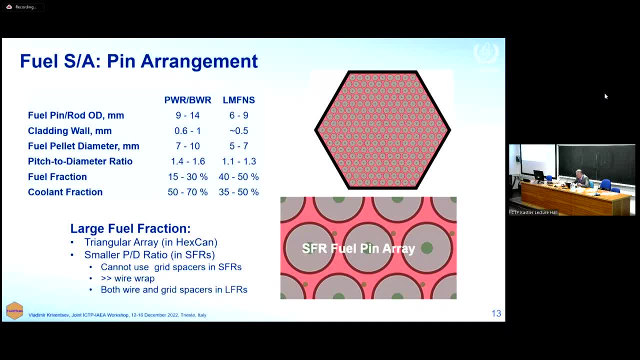 as little as possible steel to be in the reactor, but also it should withstand, it should serve its purpose to hold and do also as a barrier for the radioactive materials, to keep the pellets and keep the radiative fuel inside this pin. For this reason, of course. okay, why generally? 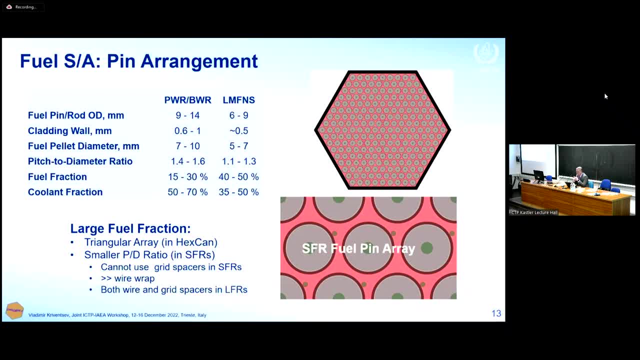 why usually fill pin rod for the sodium cooled faster at the smaller? because the energy per volume released, energy density, power density in the sodium cold fast reactor traditionally, at least from the very beginning, was much higher, like three times or higher volumetrically, than in water reactors. however, now this is like and it was considered as a benefit. 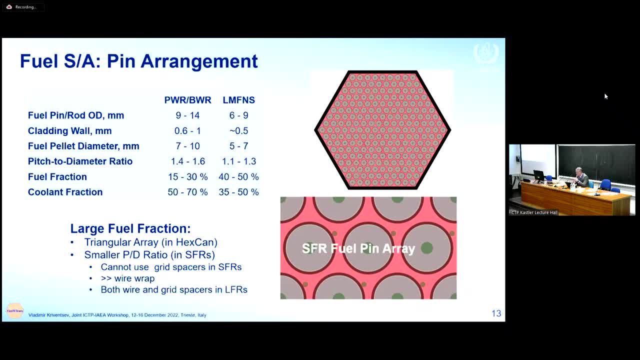 because, okay, smaller volume you can release and more power, but now, since, in general, director vessel is still much, it's much bigger than the reactor core. so and to avoid, let's say, some effects, especially during the transients and a potential accidents to that could lead to the severe accidents it is a new 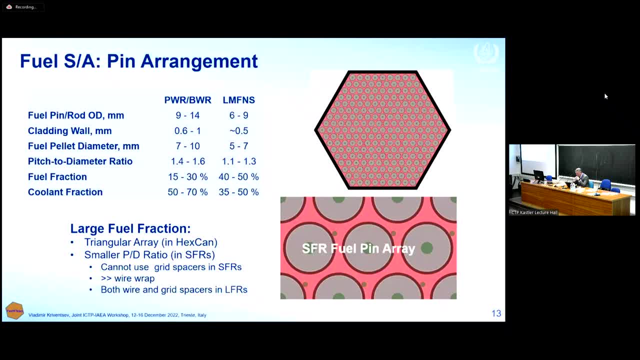 trend in the design of the reactor is to reduce the power density. now it's still higher than for the traditional water reactor. but let's say, if you compare it being a breast 300 or being 1200, the power density is like more or less than half. 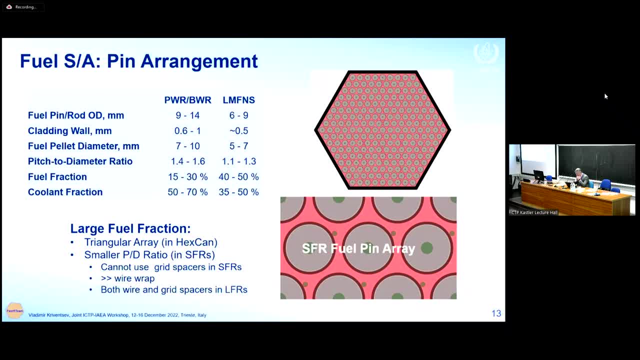 of those in the band 800. okay, and obviously once you have higher power density, you need to have smaller pin to to avoid them. the maximum temperature of the fuel, because the bigger cht diameter is larger than you thought. zuem sure this. of course you have higher temperature in the middle of this of the fuel pellet and to avoid this you. 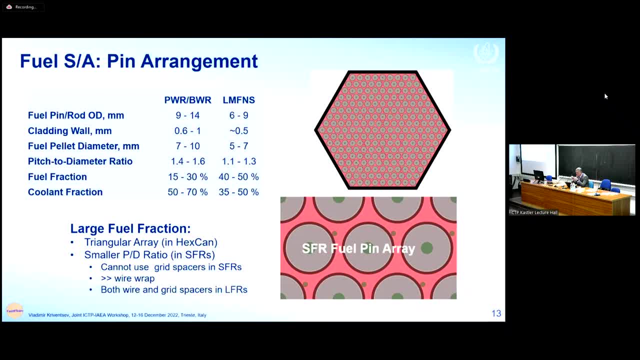 simply reduce. if, if you want to increase the power, you have to reduce the size of the pellet and then you avoid this. ideally it has to have zero diameter and which can be realized. then it's only uniform. that can be realized in the molten salt reactors, where the fuel is also coolant, so heat is released exactly in the 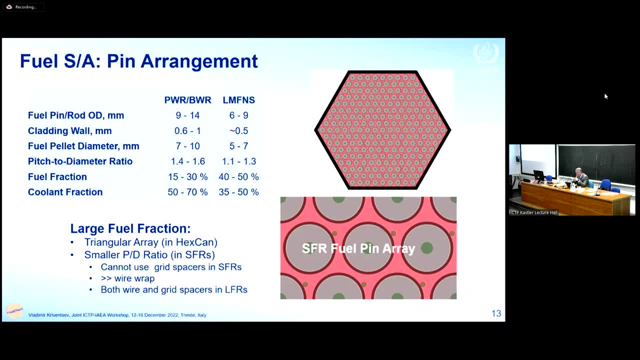 coolant itself. so you don't need these pins. on this geometry more or less, you can consider the zero diameter fuel pins also, but just to give you idea. and then smaller pin diameter, you can decrease the maximum temperature of the fuel. that's why we have smaller, because we have higher power density. we have to make 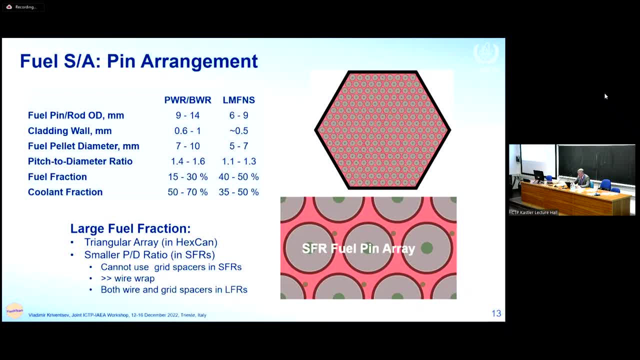 this pin smaller, because if you do is the same size as a water reactor, temperature will exceed all limits possible range. okay again, for traditionally those pin are allocated in the triangle road array, but there are also designs where they are located in square root arrays. for that, let one of 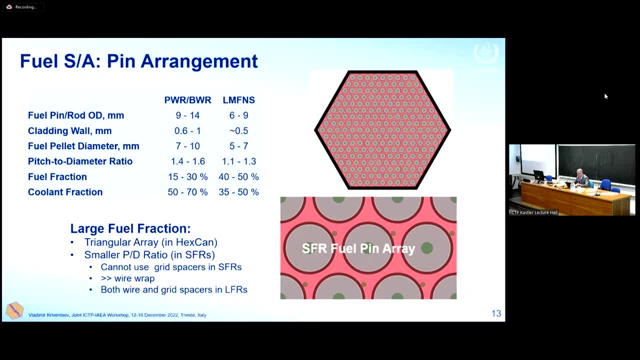 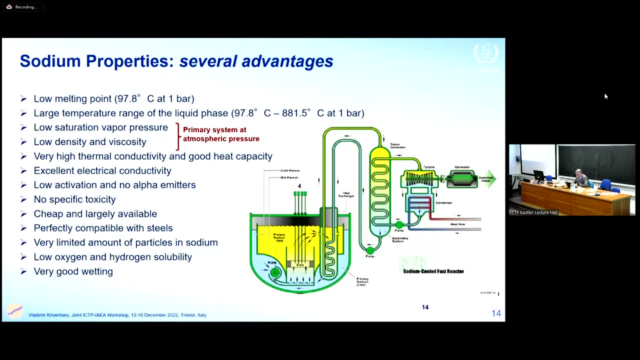 the designs of breast 300, but maybe 20, 15 years ago, was to allocate them in a square array because you need more coolant for in case of the lead cold fast reactor. okay, this I already told yesterday's the statute little bit and I believe that Christian will also explain. 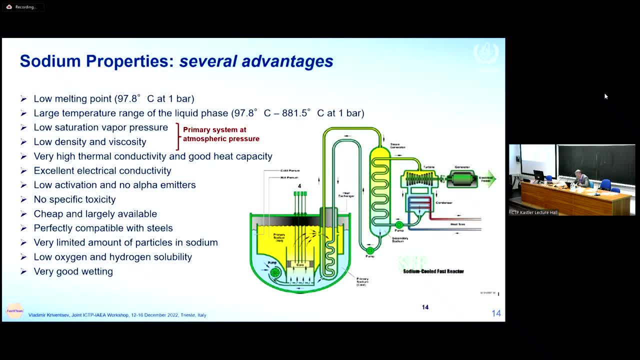 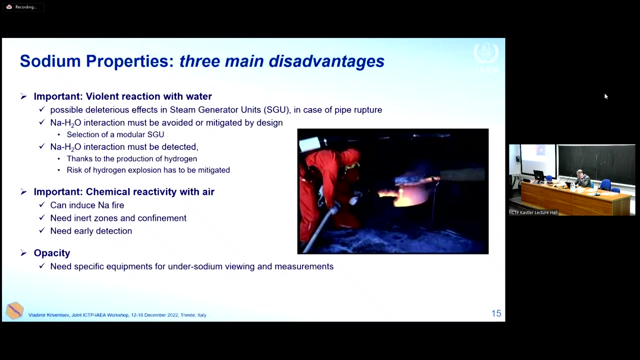 the sodium properties, advantages and disadvantages of the sodium in his lecture. again, what is important, just to repeat briefly, what is important is a perfect thermal conductivity, excellent but aggressive reaction with water and with air. also zero opacity. so we cannot do vision, you cannot visualize the insolvent inspections which can be easy. 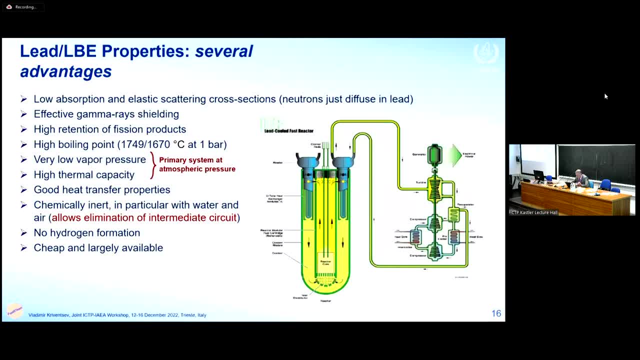 change for the lead compared to sodium. what do we have? we have this: there is no violent reaction, reaction with air and all and with water. then we can eliminate intermediate loop, which is very, very important improvement here. However, since it's has much heavier 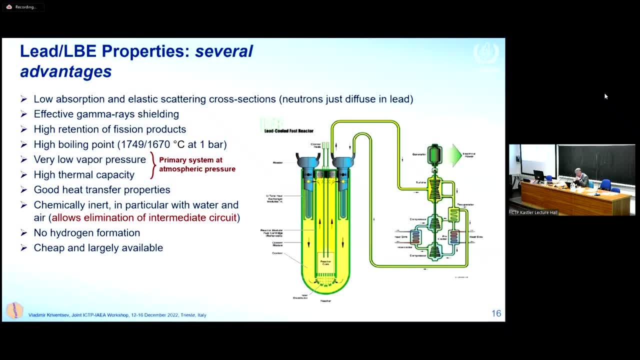 let this much heavier. it's both okay. Benefit and you know the challenge in fact. for example, we need to. we need to erosion problem. We cannot sell. velocity of of a flat should not exceed two meters per second, Otherwise. 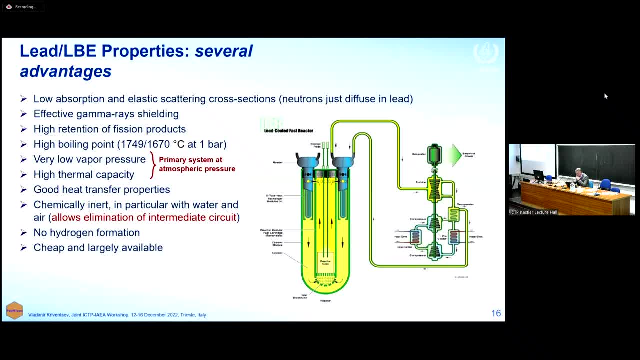 it will be affect the erosion for for for the walls. And another thing is that for the lead you have to control oxygen very carefully, Otherwise if you have very little oxygen then you will not have this oxide layer on the cladding. 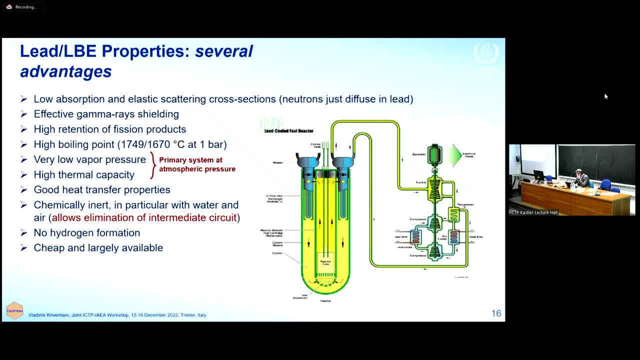 And you do this direct contact between. in steel, iron will dissolve in lead, because lead dissolves iron, And that I mean then you will. it will eliminate your wall and destroy the peak. Okay, Then you still you need to to to have oxygen in some oxygen inlet. 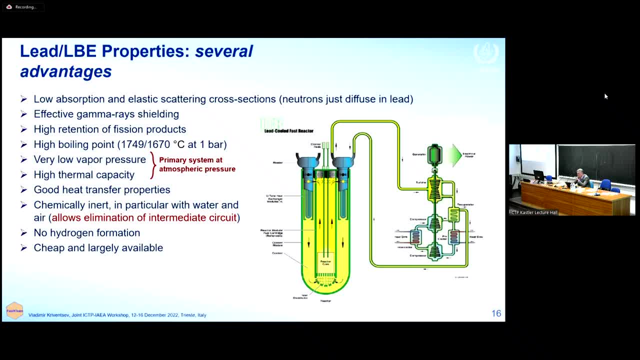 but if you have a lot of oxygen, this oxide layer will become very sick and then it's a problem for the blockage It's- let's say it's broken. This, this pieces of oxide materials. they can block and the flow passes in the system. 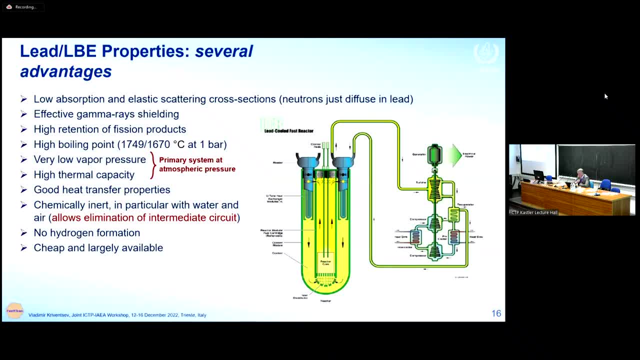 which is potentially dangerous. Okay, And it's. it's probably, it's confirmed by the experiments or uh, or an experience also, not only the experiment, but also experience. So for this you have to control oxygen always in the system on the certain level. 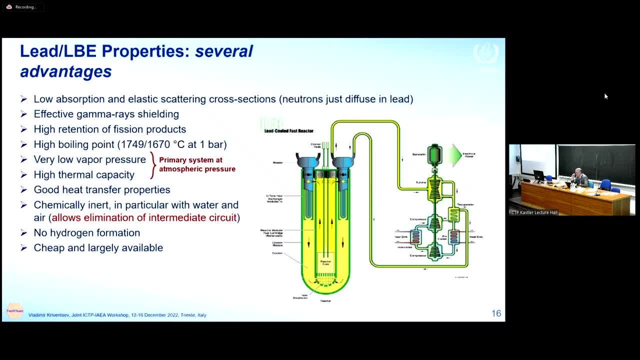 And this concentration of oxygen also depends on the, the temperature. Let's say, for the low temperatures you should have, keep the oxygen level is lower, for the high temperatures You should increase, or maybe vice versa, I don't remember, but it should be controlled always. 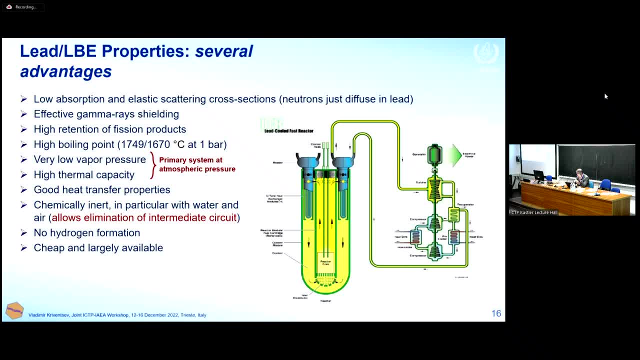 And you can imagine that in your system you have some zones with low temperature, with high temperature, and this is become a challenge: controlling the oxygen. This is one of the challenge for the lead. However, from the other side, it's uh. 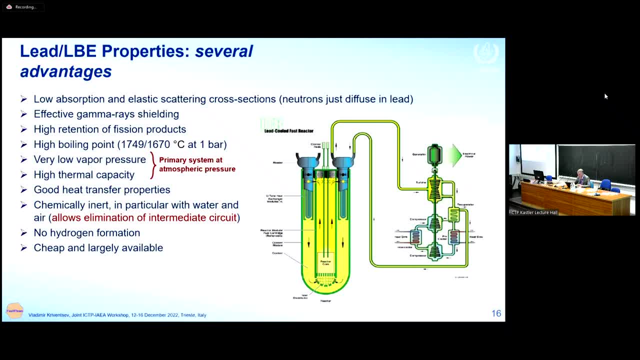 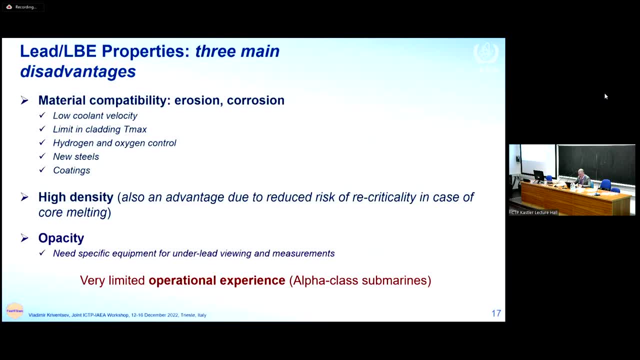 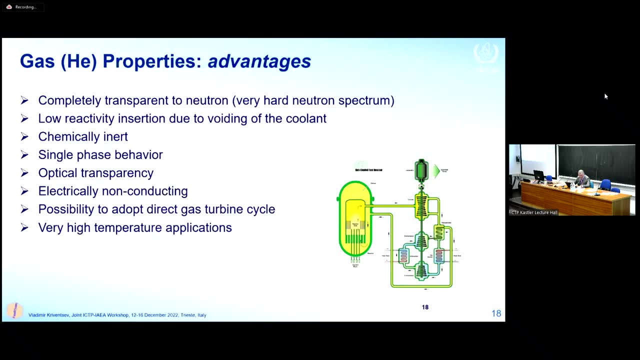 especially allowing elimination of the intermediate circuit, intermediate loop. It's very, very big. And let's say, the benefit for this material. Again, I will skip this, probably because also I want you to talk, to talk about the uh as well as for the lead. cool, Oh sorry. 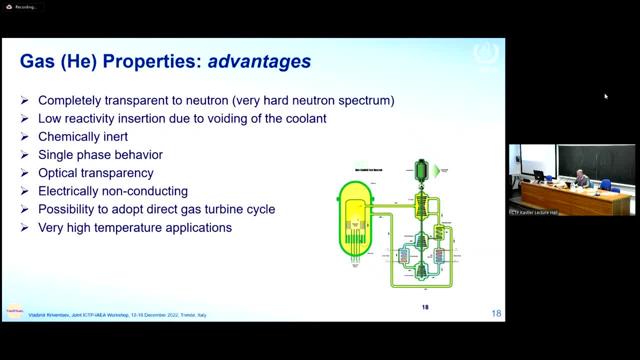 So the liquid metal cooled reactor. So we have for the gas, we have an uh. for example, gas helium is considered as a one uh potential coolant for for the gas cool fast letters in generation in GF generation for systems. 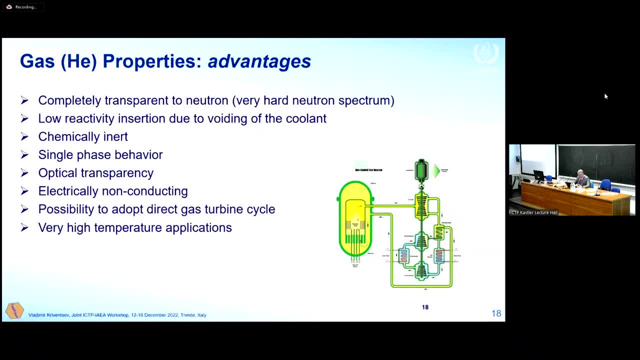 So it actually has very perfect properties: transparency, uh, chemically in that, So you don't have to make any measures. no transport to new trans, no reactivity insertion to remove, so it doesn't affect the activity of the reactor, for example, the sodium. the problem is if 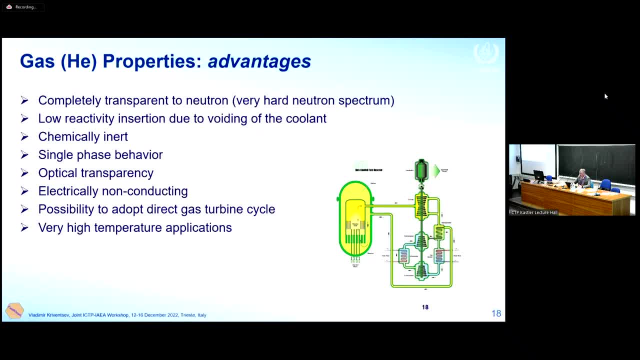 for whatever reason, sodium is boiled. or leaves the core region and core becomes because we say void but it's not void, but it's just sodium is evaporate. or, for whatever reason, leaves the core. it gives, because sodium still absorbs neutron and when you remove the absorber the criticality becomes. 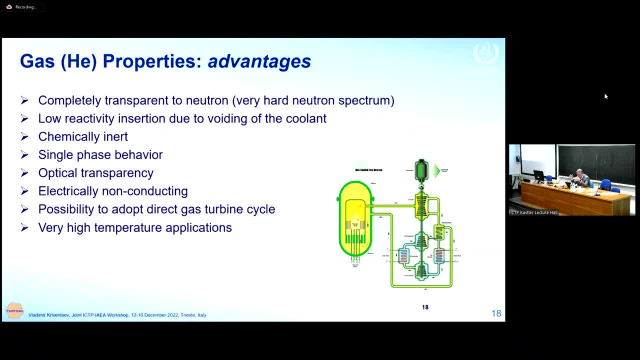 becomes higher, what you call the in sodium cooled fast reactor, and also let the the corner is not configured is most critical configuration. so by compaction or by removing sodium you can increase criticality and that is potentially can lead to the cv accidents also in this case with gas it's not a problem at all. the only problem is you need very hyper because 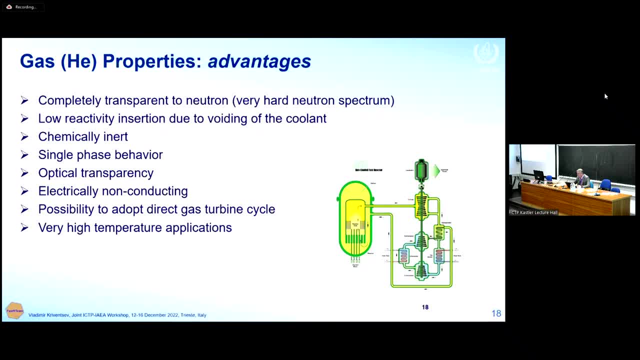 to remove the heat you need really heat cup. in heat capacity of helium atmospheric pressure is. it's very, very small, so you you can remove heat with helium, so you need pressure like 20 mega pascal and this is also can pose some danger. still can be solved and their projects i again skip. 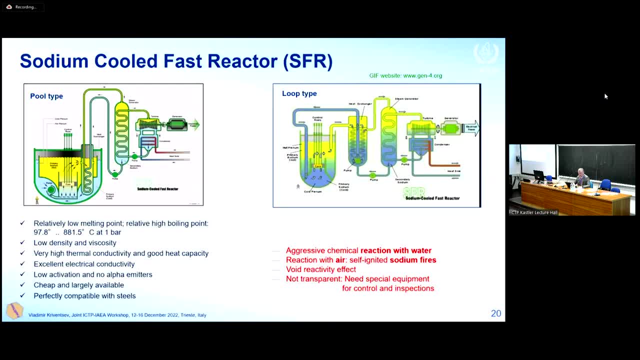 let us. that was example how to how coolant i influence the thermal controllers. here again for the sodium cooled fast reactors, we have two types, both with intermediate circuit, by the way. one is the so-called pull type, when you have this intermediate heat exchanger inserted in the primary pool with huge pool. 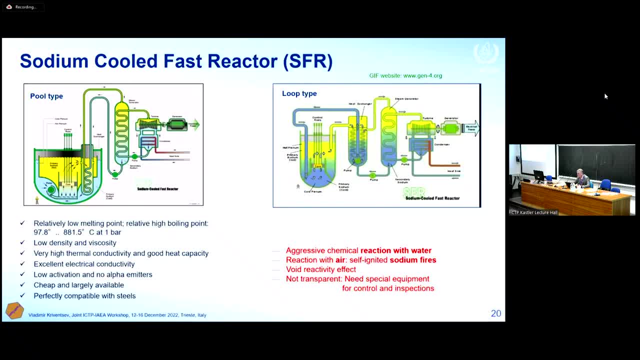 which is has huge inertia, which is okay because it could help during transit. could help sodium is with its allocated heat or cold in this case, could survive transit, many transients and for. but for the countries with seismic activity, such as in japan, they require the pull types. 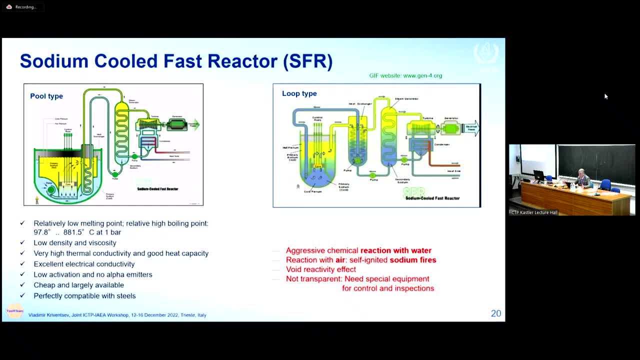 uh reactors are impossible because it's a huge mass of the sodium in one volume and in in case of earthquake it's very difficult it should destroy the vessel. i guess for this reason, for example, japan is considering loop types reactor which are smaller core, but for this you need the intermediate loop separately, so it makes the total amount of the structural 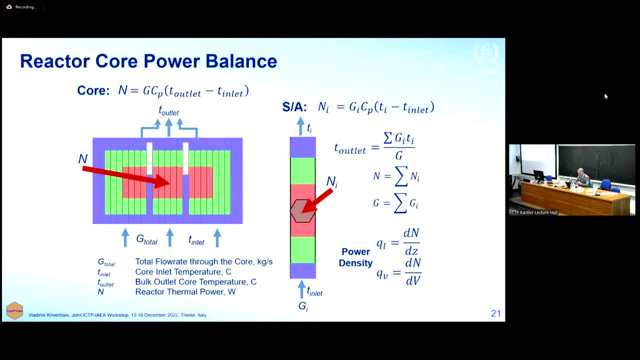 materials higher and increasingly. okay, now let's also talk. how do we calculate very simply thermal hydraulic? and we start with the reactor core power balance. it's related to this exercise that you received yesterday evening. Maybe try to calculate So generally you have, the heat is released in the reactor core. 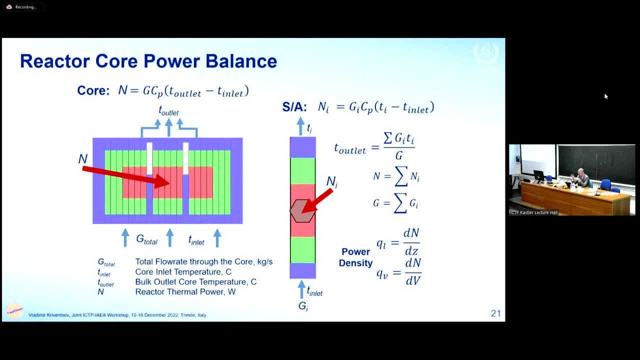 and should be removed by coolant and transferred to the outside of the reactor. Then it can, of course, be converted. This heat can be transferred to the water, evaporate water, finally, and the steam will go to the turbine and generate electricity. 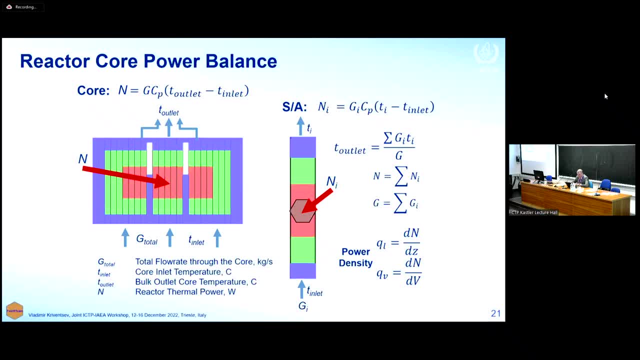 We consider how to remove this heat from the reactor core. So for this you need very simple. If the reactor core is N, its total power is Watt. So total flow rate, heat capacity of the coolant gives you the difference between inlet and outlet temperature. 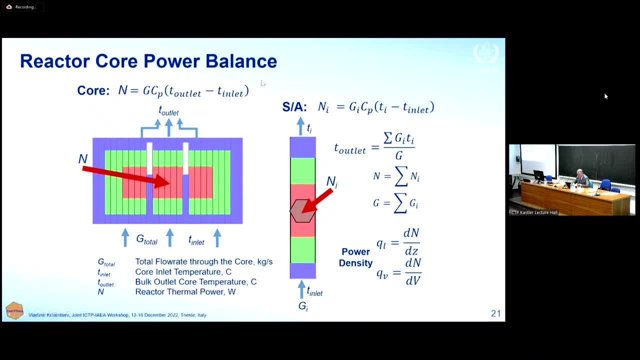 This is simply balance and energy balances here. This is valid for the whole reactor core When you consider the bulk inlet and outlet temperature of the coolant, but it's also valid for the every sub-assembly as well. So if you provide the flow rate inside the sub-assembly, 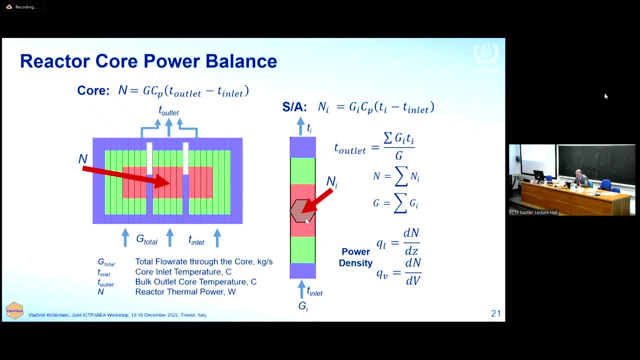 and you have inlet temperature and you know how much energy is released. so we know the power of this sub-assembly. you can calculate very simply the outlet temperature of this particular sub-assembly. For the power we can consider also the total power of the reactor or sub-assembly. 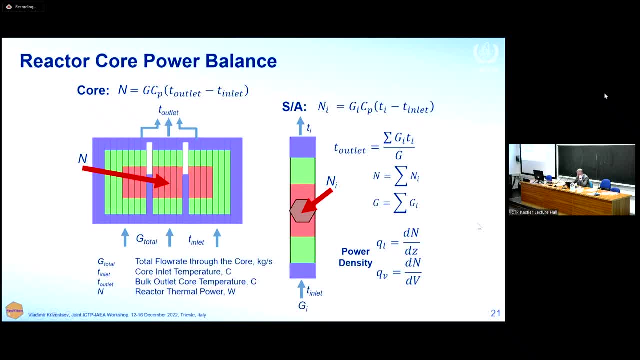 and I. I is the number of sub-assembly And also we can consider the power density. If we QL is the linear power, which is how many power is released per the one meter of the axial length of the sub-assembly. 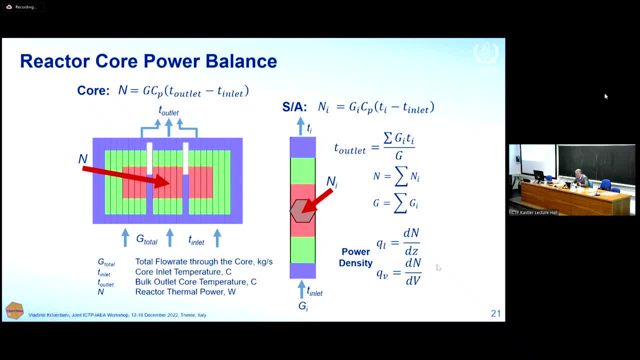 or of the fuel pin, Or if you have volumetric power, or if you have volumetric power, or if you have volumetric power, so you can also calculate how many is released during the work. This is simply balance equation, What we can use to first, to do with the exercise. 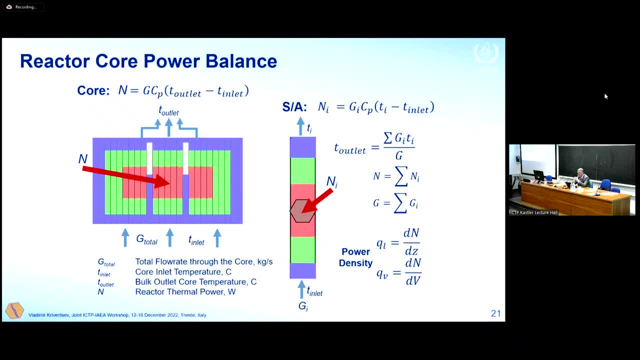 Once you have the power district, total power, you can automatically, of course, calculate the outlet temperature. okay, Then you calculate this cosine distribution of the power, of the linear power, in the axial directions. Then you can split your fuel pin in several blocks, like say 10,, 20, I don't know. 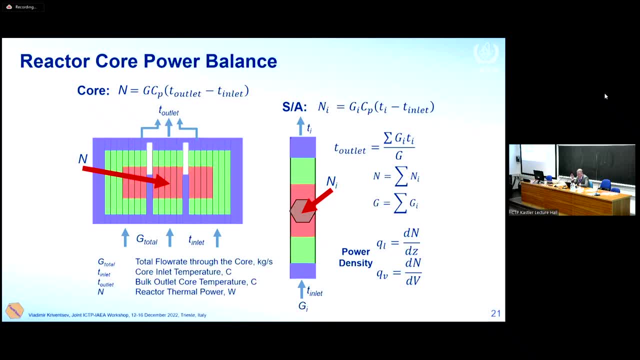 Then you can split your fuel pin in several blocks, like say 10,, 20, I don't know, We say. and assuming that linear power in every delta Z you can calculate with this delta T for every block, So finally you will have the again. 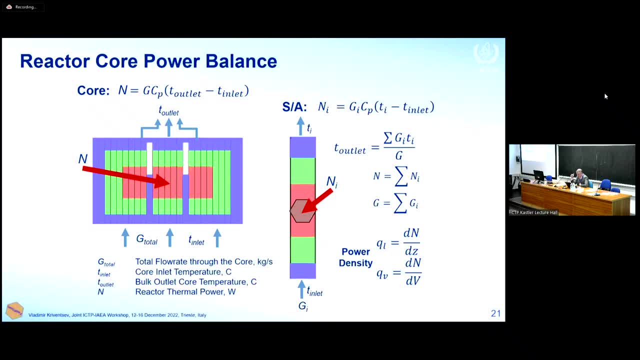 but going through this, all, all this, this mesh, I would say, is absolute direction, You will receive the outlet temperature, which should simply coincide with the outlet temperature which you can calculate from the power balance from this particular sub assembly. Okay, this is clear. 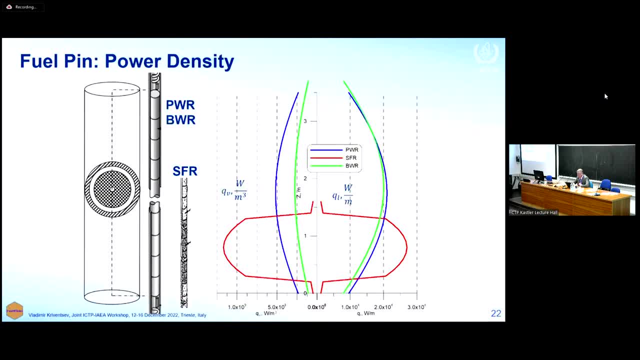 Just let me make it sure this is clear, okay, And let us compare now. So we were talking about the cosine distribution. Cosine is an approximation, So we approximate, like cosine, in the axial direction And basic function is the radial direction. 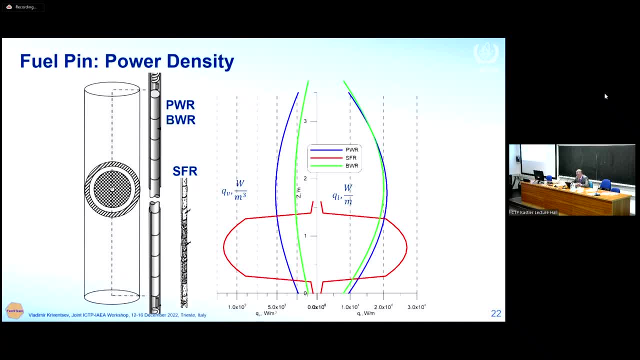 But again, this is an ideal approximation, which is of course depends on the position of the contour road or so on. But first let's say, uh, iteration, or first initial guess it's it's a power distribution, is cosine, Usually what we know from the nitronic simulations. 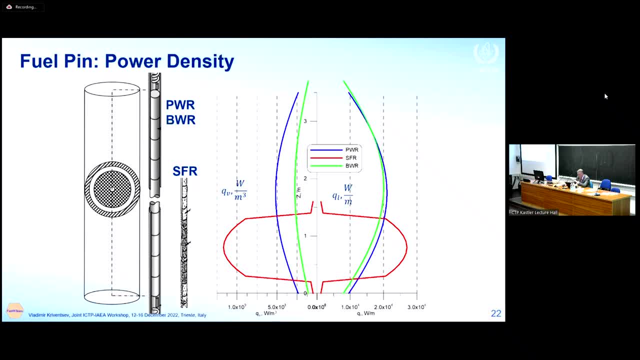 so power distribution is simulated by nitronics code, like Monte Carlo or different codes. But so for the thermal hydraulics we already receive this power distribution as an input, And usually they give a simplified simulations or the designer give you the picking factor. 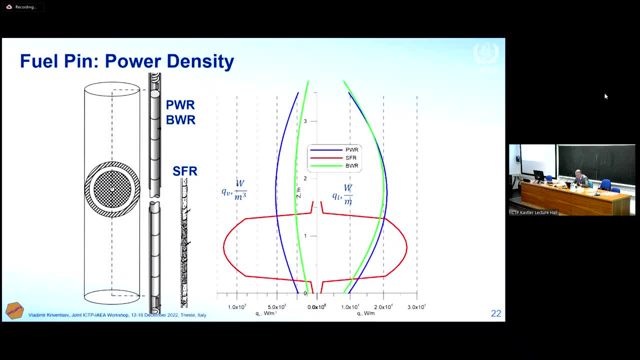 So the coefficient which makes you it's a maximum power divided by the average power, What also I give you yesterday. So let's compare, compare this power distribution here, volumetric per watt per cubic meter and also linear power of the pin. 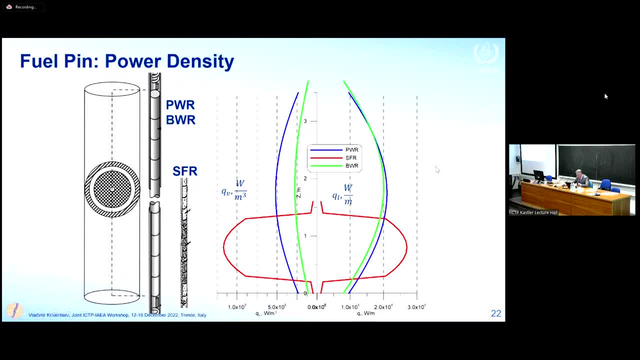 For it's maybe- I know I'm not sure it's supposed to be now, but probably for the pin. uh, compare with boiling water reactors, PWRs and uh, this um sodium cooled fast reactor- Sodium cooled fast reactor pin is smaller in diameter and also short. 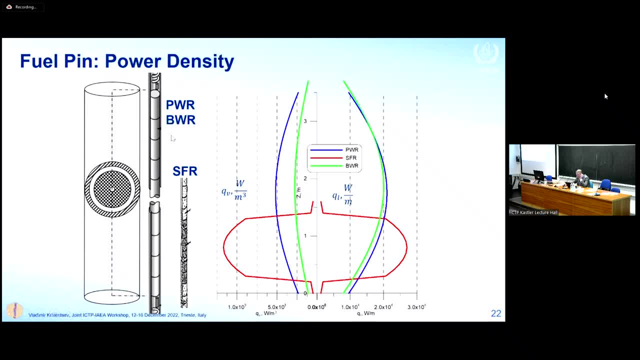 much shorter than compared. If you have here like three meters, probably for the, for the SFRs is a. it's about the active, what we say fissile core length is about one meter, So it's three times less. So green is the power density for the volumetric here for 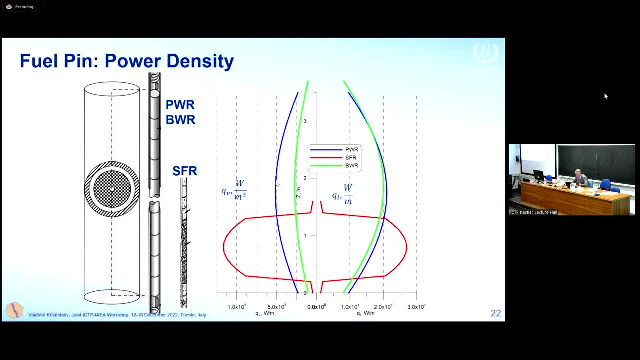 for the boiling water reactor, Blue is for the PWR and this is for power density for the sodium cooled fast reactor. You see that it's much higher power density And that also linear power density in pin is much higher. So, and this has become a problem in this case. 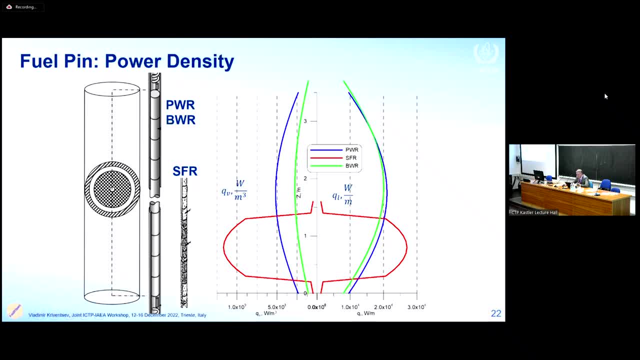 I will show you the Phoenix Phoenix reactor, which is traditional and typical, let's say SFR prototype that and you can see that power density, linear power density, is double for for the sodium cooled fast reactor compared to almost double compared to them. 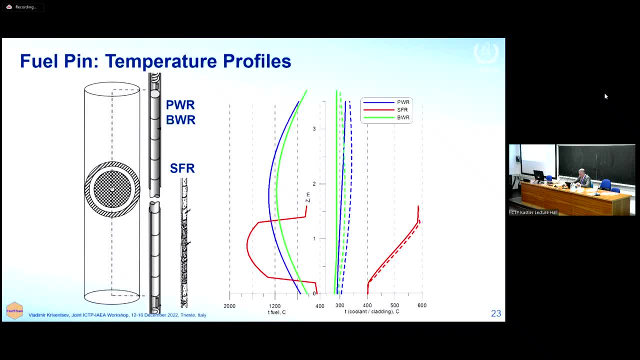 Uh, what The cool tractors. Uh, if you look all now, it's a temperature profiles. This is on this: on the right hand side you see the coolant temperature profile and on the left hand side here is the fuel maximum fuel temperature. 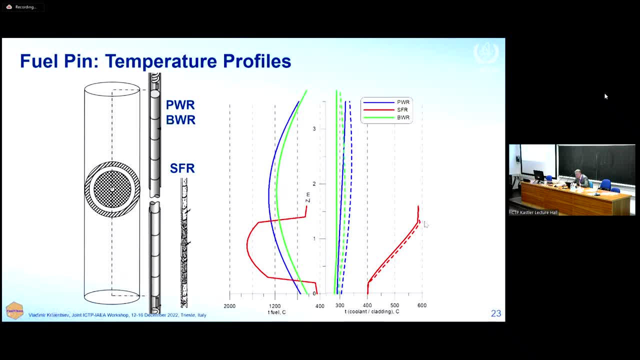 So okay, For the coolant it's a heating. The difference between inlet and outlet temperatures is about 200 degrees C for soil. Now it's it's less, So now we want to have it, not more than one: 50 in many cases is 120, something like that, smaller. 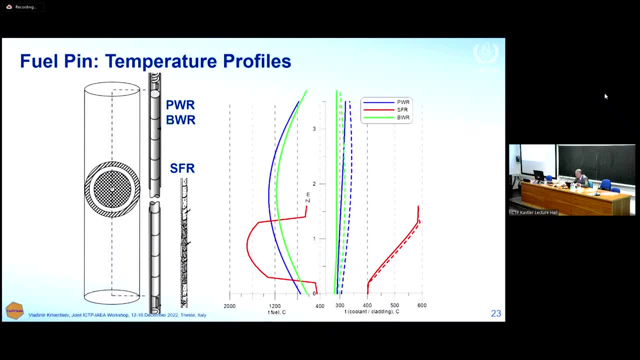 So just designers don't want to to this high power density for for, for the, for the liquid metal cool fast reactors now, but it used to be typically like this. That makes it's a challenge to to to remove the heat from the reactor. 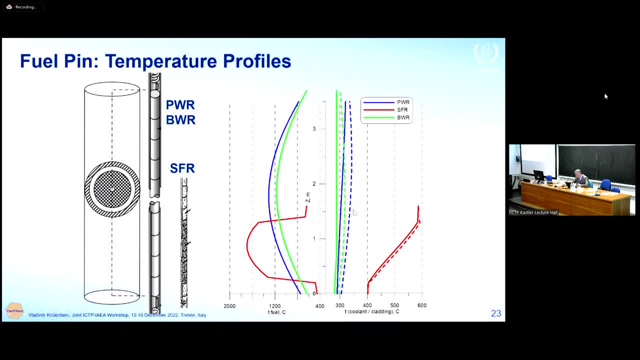 You see that. And temperatures, if you look here, it's much, much higher than for the water reactors. obviously Okay, And that is a benefit of fast reactors. Also, with higher temperatures, the efficiency of generation of electricity is also higher. 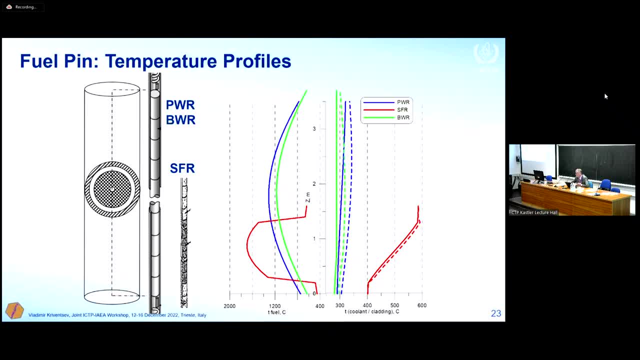 If for the water reactor is 30,, 32%, for the sodium cool fast reactor you can reach 40,, 45 probably. like this, So much better efficiency. You don't lose this energy which raised in the reactor Today. you don't waste it to the environment. 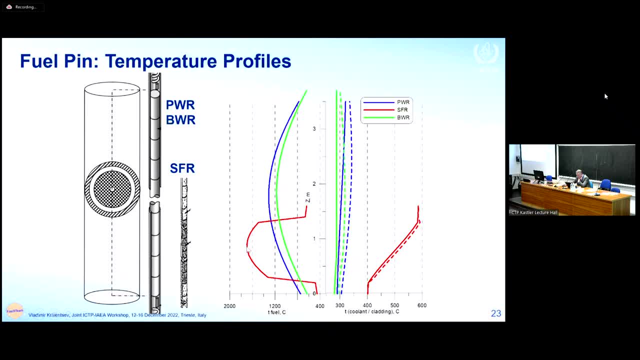 I would say if you look at the maximum fuel temperature, it's also higher for the sodium cold fast reactors. even for the same few fuel like uranium oxide or mox fuel, you see that the temperatures is much higher, which is challenge also because 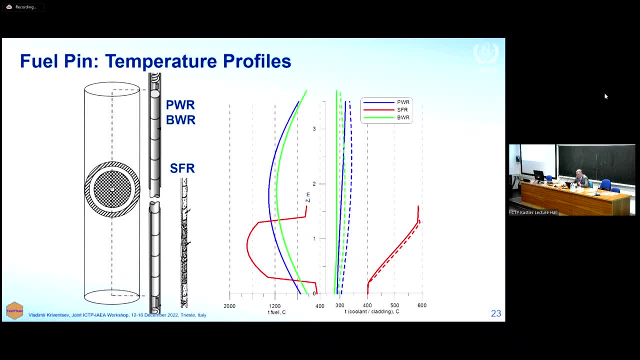 uh and also taking the burn up. So neutral, neutral. So amount of neutrons which uh, at least in in the per volume of the fuel in this sector for the fast reactor is much higher than for the light water reactors. 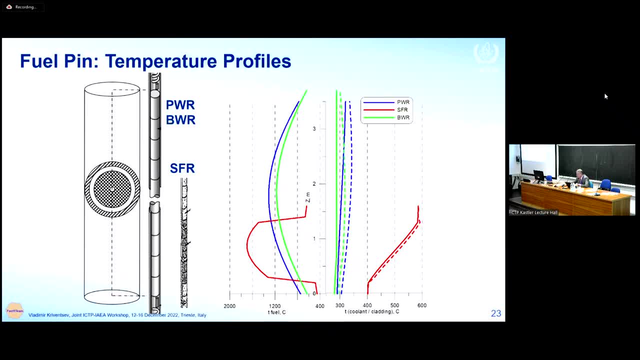 So we call it burn up, and total energy released per per kilogram of the heavy metals are much higher in the sodium cool fast reactor. with this high temperature, It's it's it's makes a challenge for the, for the fuel designer. 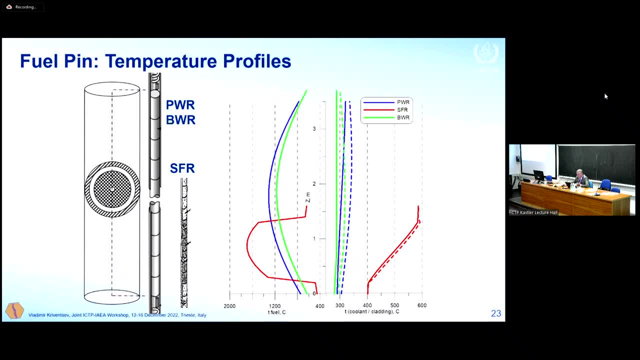 That's why, of course, uh, from the one side you want to, to, to, to reduce the burn up, but also from this, it depends how much, uh, how much of new fuel you can produce as a breeding, in the breeding materials, from the breeding material. 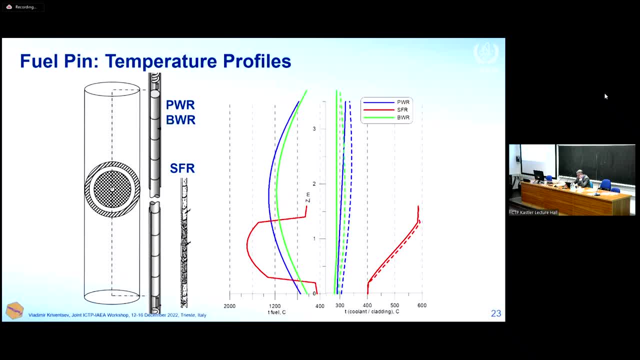 how much plutonium to three nine, which is for sale material we can produce from the uranium to three eight. This is also depends on the burnout, of course, not for the of the temperature but from the burner. but to have temperature lower. 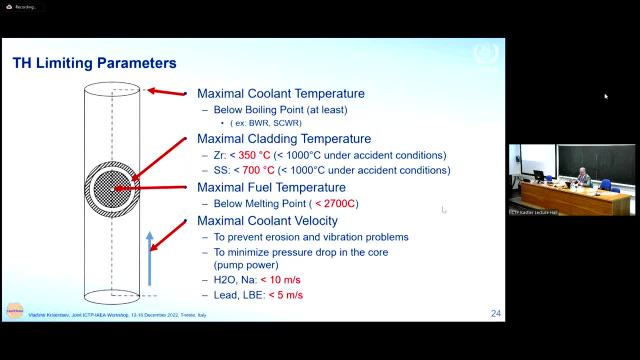 it's better In this case, please, Okay, And generally speaking, the uh. the limiting parameters for the designer, if you have a fuel pin simplified in this way, will be the maximum coolant temperature. It should be at least below the boiling point. 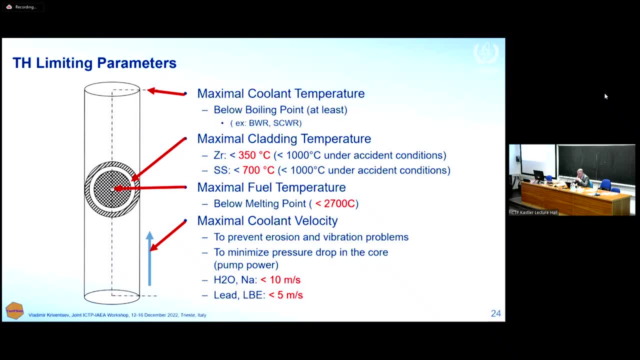 Okay, But of course, if you look at the BWR, it should exceed- I mean it's just reaches the boiling point because it's a water evaporate there. If you look at this, the supercritical water reactor- there is no such as a boiling point for the supercritical materials. 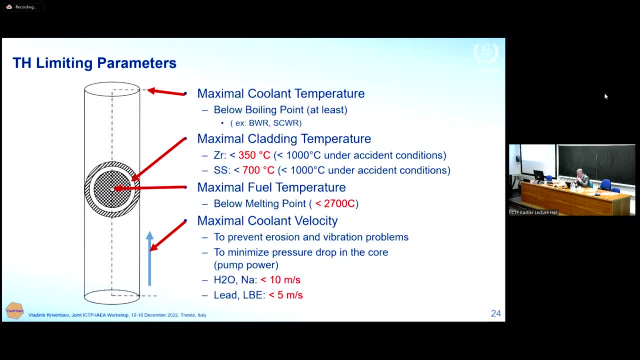 So it's. it's an exception of this rule, but in generally it should be below boiling point And I would say well below the boiling point. So you have the some uh margin to to to this condition. Consider also that not the pins in the reactors core. 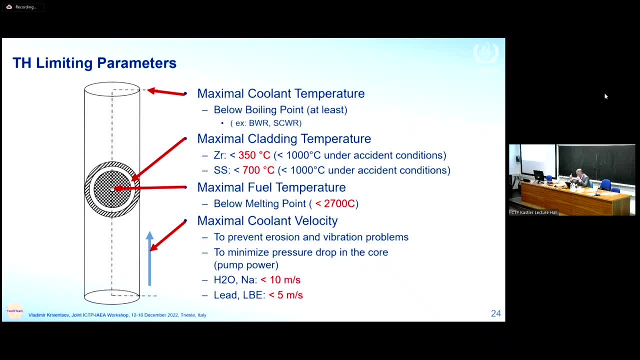 they are not in the same condition. Some pins are due to the power distribution. They can be more loaded- I mean higher power- and some pins are lower power. So in this case we should consider the maximum power pin and at the same time with the lowest velocity of the coolant, because the outlet temperature depends also on the velocity of the coolant. 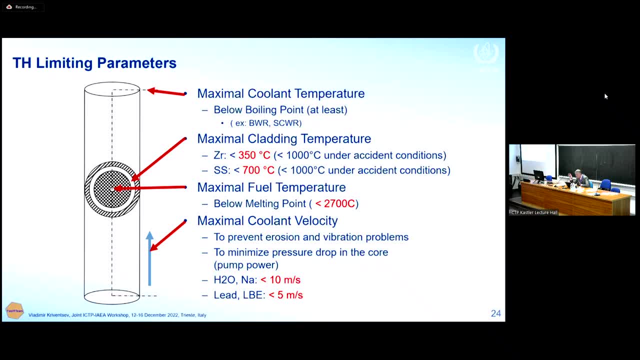 Lower the velocity of the coolant, proportionally you have higher outlet temperature. Temperature difference is exactly. it depends on the velocity of the coolant. Okay, Another um limits in temperature is a maximum closing temperature. Let's say, if you talk about zirconium for the water reactors. 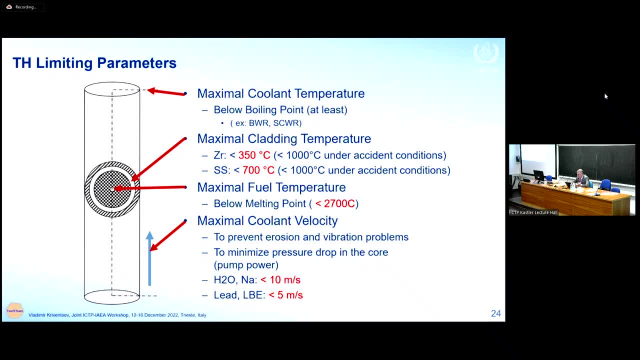 it should uh be lower than 350 degrees C, I think it's, frankly it's also should not exceed boiling point, for example, And uh, just for good. So the bulk, the bulk temperature of the coolant, of course, is lower than the temperature of the cladding, is high, because you have the heat transfer between coolant and and clad in the wall of the pin. 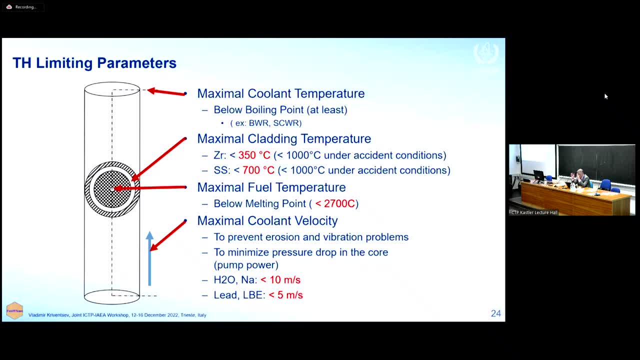 This is defined by no sick number and this is difference. Actually, it's perfect heat transfer for the sodium cold fast reactor, but for the water reactor this temperature difference is much higher, Can be 30, 50 degrees C, while for the typical for the sodium cool fast reactor. 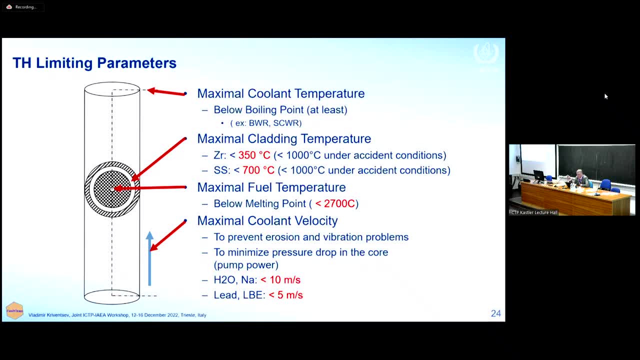 it could be seven, 10 degrees C, only difference. So it's very small and that is a benefit, benefit of sodium. So just to understand the, of course the volt temperature is higher than coolant temperature in the same XL location. Okay, And this is a limited parameter, that for stainless steel, as a designer say, it should be lower than 700 degrees C. 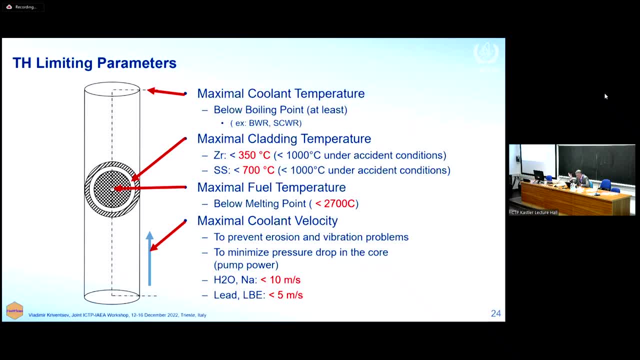 And this is a maximum limit which still can survive and also should be lower than 1000 degrees C on the exponential conditions. Another parameter: Then you have a gap, potential gap between fuel pellet and wall from the stainless steel wall or cladding in this gap because it's a gas gap. 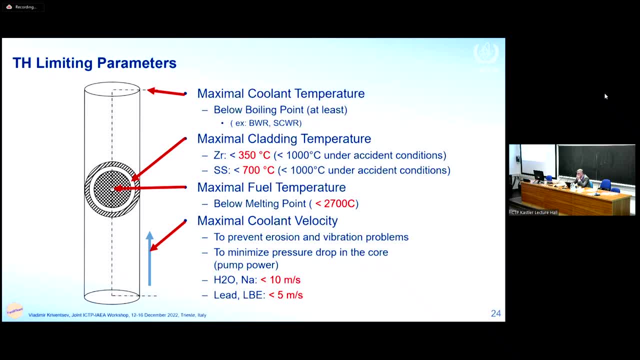 You have additional, maybe 50 degrees C, only one. Okay, One hundred degrees C, depending on the gap side and heat transfer coefficient is a gap. You have additional delta T, additional increase of the temperature, So the outer surface of the fuel pellet is higher temperature than in the surface of the cladding and then you can reach the maximum temperature, of course in the middle of the fuel pellet. that should not exceed melting point. 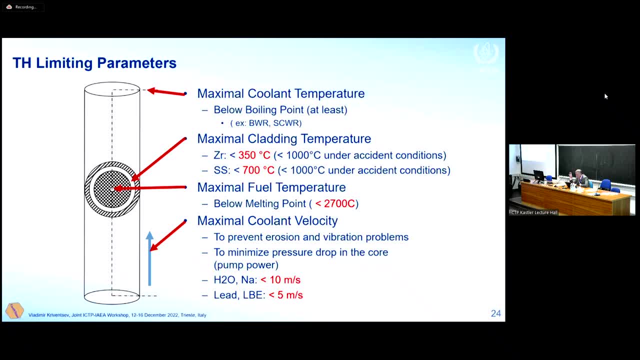 Never exceed, should never exceed, melting point. But of course you, you, you want to have the margin and take into account that there are trends that can do some trends and some accidental conditions. It should not exceed this in this temperature, melting, melting temperature and just and also consider that the power- again, power has a distribution and the maximum 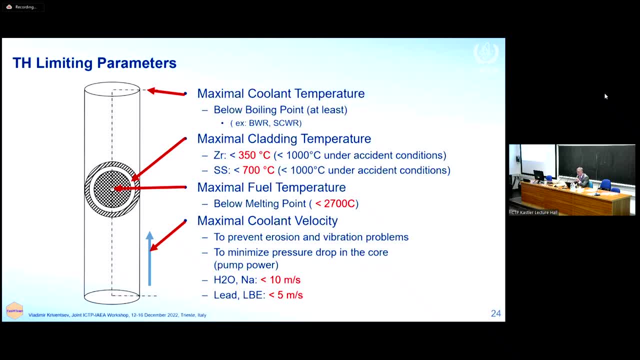 temperature Of the Fuel is reached nearly in the actual center of the quarter. For coolant temperature is maximum temperature is in the in the outlet of the Fuel assembly. For the cladding, in case of water reactor This is shifted so the maximum cladding temperature not in the outlet but little bit below. for sodium cold reactor: because of the sodium 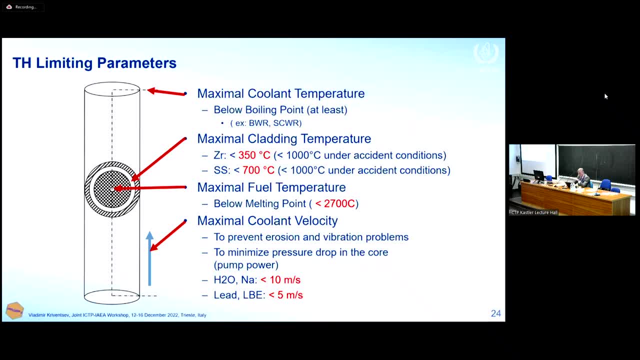 Thermal conductivity high. it's Just below. I mean it's actually the same as the out the temperature of the coolant, Maybe two millimeters slower, If to be precise, but you can consider it the same, Okay, and another, And Limiting parameters and maximum coolant velocity you can afford for the water and sodium is should be less than 10 meters per second. 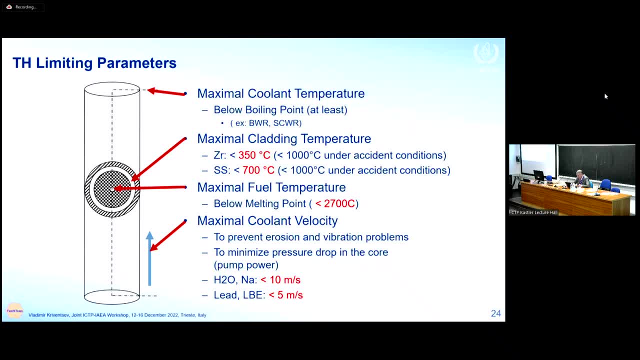 But usually it's seven or five meters per second is allowed in the typical design reactor designs for lead and lead. this month it should be less than five meters per second. but now the new, for example for the breast, is the reactor. the limiting parameter is two meters per second. that why we also trying to calculate the, the dependence maximum temperatures versus velocity of the coolant, and this exercise which we distributed yesterday. okay, 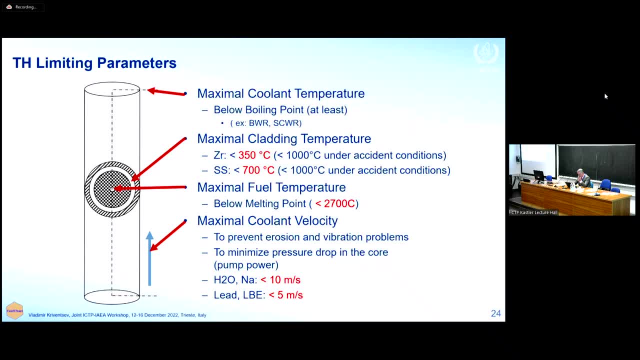 So When you do this from hydraulic calculations, you should make sure that this temperatures are not exceeded. or vice versa, if you know this limited temperature, you Should calculate the power that guarantees that you not exceed these temperatures. or you have given power the pin, you can calculate the temperatures, maximum temperatures, or if you know the limits, you can calculate. 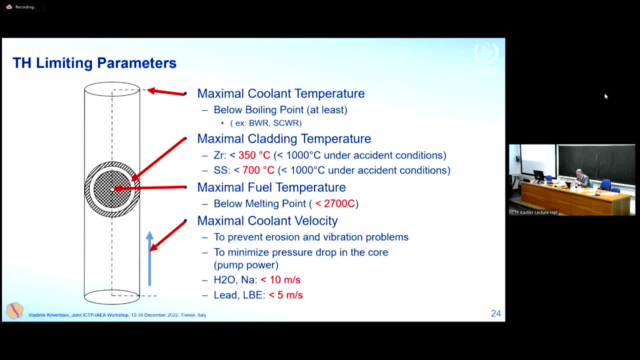 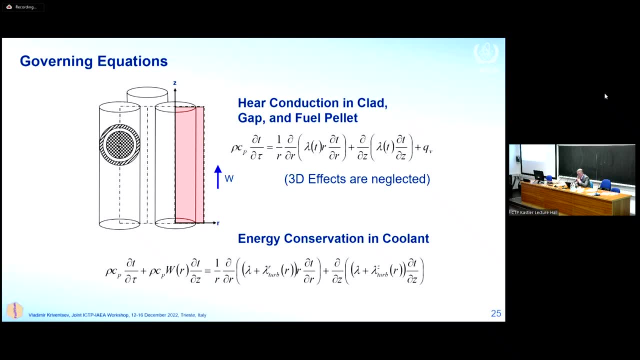 The maximum power of the pin that can be applied to this. Okay, how to calculate it? so maybe, of course, we we can have this very simplified calculations, but typically you have to solve the energy. okay, now, yes, talks or you know, it's in the region of your stock equations to to get the velocity profile and then, once you have it, you can. 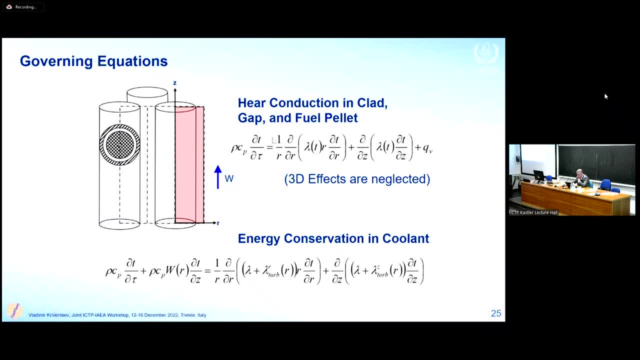 Calculate Temperatures in the solid, in the solid structures like fuel being and cladding. you can calculate solving this energy equation for the thermal conductivity It shows simply two dimensional and transit equation and time and distribution in our direction, in the direction depending on the volumetric heat in this material. here we affect. 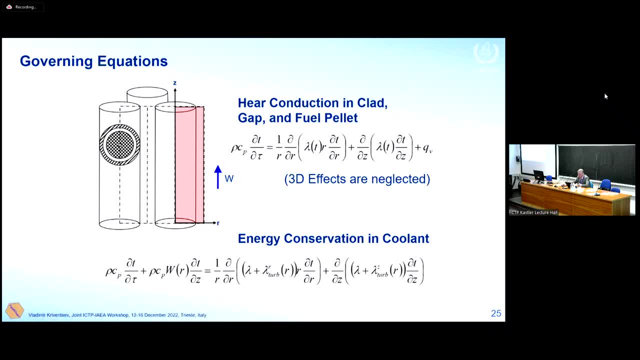 3D. We neglect 3D effects For the case. of course we can also add this As a motor direction as well, but in this case we neglected, especially for the Close, with good coolants, conductive coolants such like sodium, so- but for the coolant this equation becomes more complicated, and this is already. 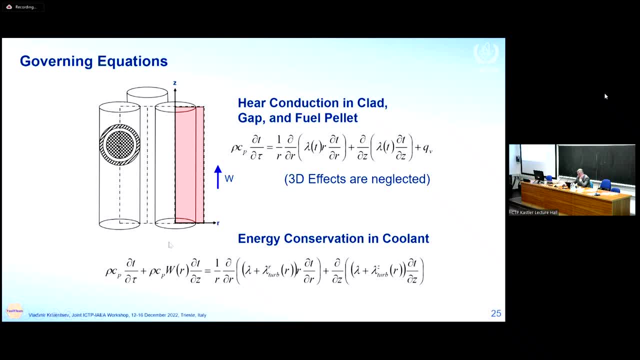 Not severe agent, and we're stocks equation, which includes this velocity distribution, If you know it, for the in the radial direction, again neglecting the effects of the azimuthal distribution, and in addition to the coolant conductivity, we have to add this term, so-called turbulent conductivity of the coolant, which is a result of the Reynolds. every region of the 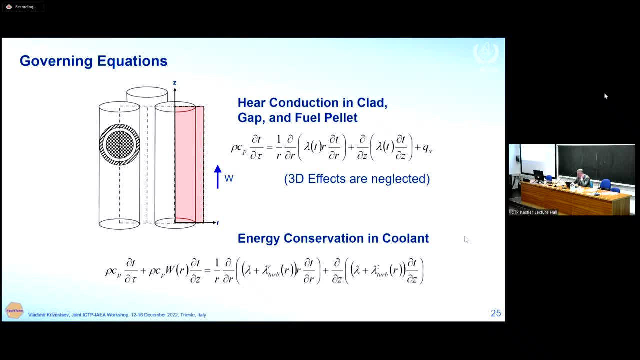 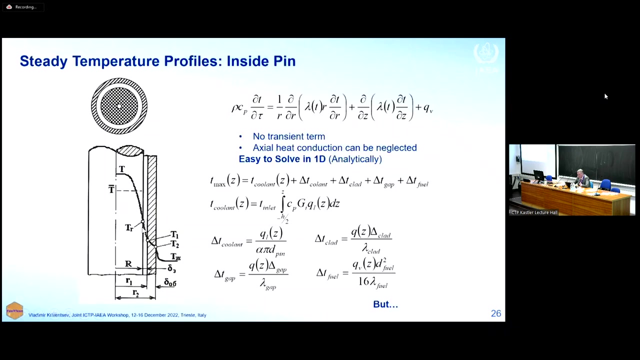 Yes, energy, in this case is energy equations, both in and in the radial direction and Axial directions. that because it could. it's not a neither any of the tropics, so it could lead to the additional effects. Okay, so to calculate the temperature distribution in these channels, both inside the fuel being and cladding and inside the flow area, you need to solve this to the creation. 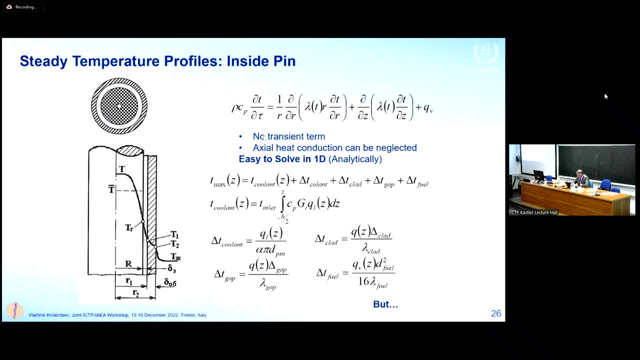 And again, if you, if you neglect- I think it's Here- If we neglect this, If we neglect this, If we neglect this transit effect, for example, for the steady state. it's very simple, it's a copy. So if you have coolant temperature- here this is, using the heat transfer coefficient and lucid number- you can calculate outside temperature of the wall. then, using conductivity equation, you can collate inside temperature of the cladding. 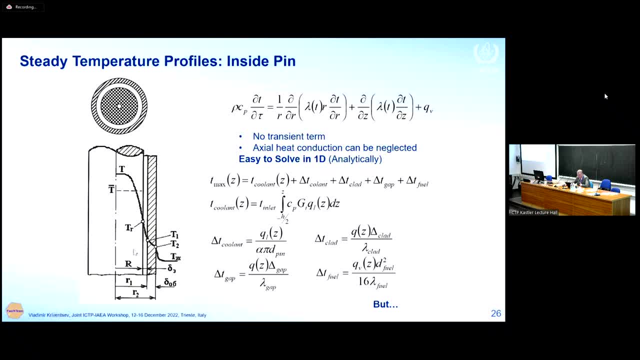 Call inside, which Is the one here- then if you know the gas and, for example, you know the properties of the gas and also it's not linear effects, because it's also could be radiation, you can calculate external temperature of the fuel pellet. finally, you can calculate. 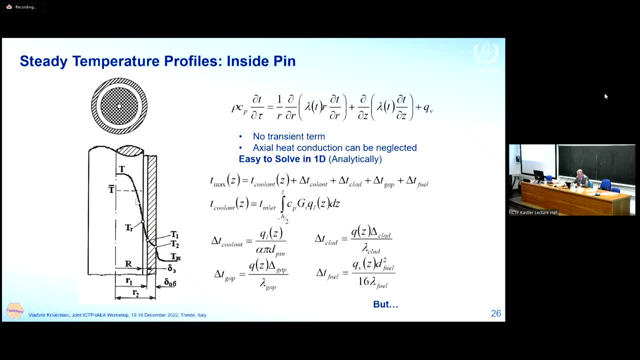 If you know the conductivity and dependence of conductivity versus temperature, you can play the maximum temperature which is supposed to be in the center of the Pellet. Okay, it's in case if there is no, So Of all, It just happens in the pellet, but the central hole is more or less the same. 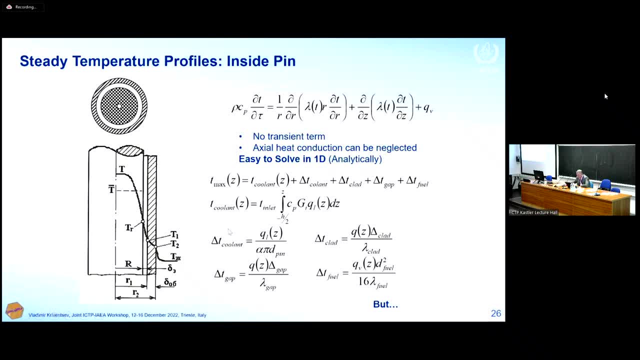 So for this you need to calculate this equation and very simplified you. you have deltate in culant, you have deltate in cladding, define it like that. He depends on the alpha. is heat transfer coefficient here Lambda. here, instead of K, we use lambda for the thermal conductivity of cladding of fuel and or also of the 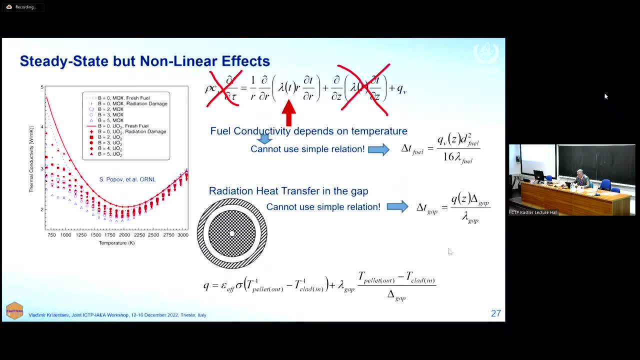 gap. it's very simple, looks very simple, but there are complications because the conductivity, for example, of the field depends on the temperature. so I mean, here you can solve. if we have this constant, you can solve this analytically and receive very quick solution. but since, for example, the conductivity of 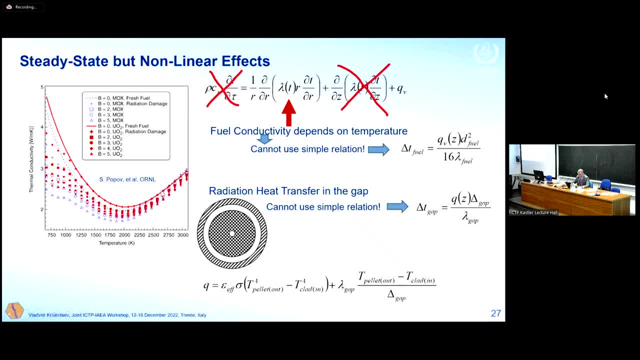 fuel. thermal conductivity of the field depends on the temperature. okay, that means this function of temperature as well and these equations that cannot be solved analytically. but of course you can solve it iteratively. but then you have to allocate mesh and do something. do some the numerical tricks also to 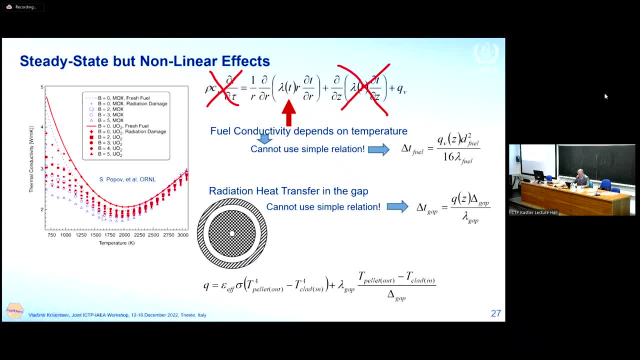 solve it. and and it changed significantly from to what per, metaphorically Kelvin, up to three, depending, and for the low temperatures even. it's like all four point five and even five. okay, so this change in the thermal conductivity of fuel should be taken into account in, in, in, usually in the calculation. 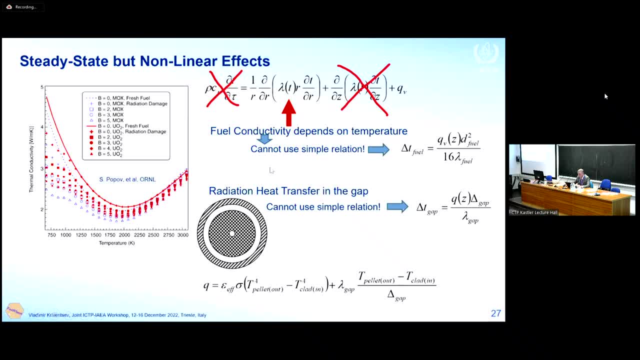 otherwise, you, we don't know what is the real temperature of the, what is the maximum temperature of the fuel and which is the limb which is the limiter parameter here. so instead of this simple relation, we should make some numerical tricks and simulate it numerically also. the 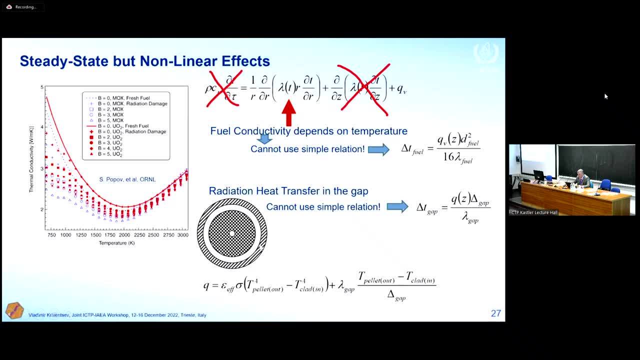 conductivity here in the gap is not only because it's a high temperatures and transparent gas. so you have to take into account the effect of radiation if radiation heat transfer in the gap, which is nonlinear effect, also can be solved analytically here, and so we should need some numerical tricks. 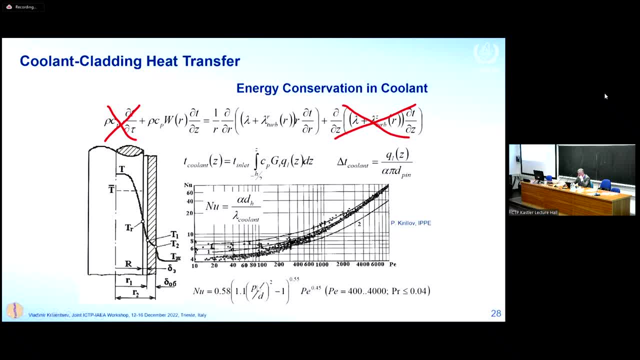 finally, of course, the most- uh, i know not most- challenges, but the thing that doesn't allow you to solve it all analytically. then if you have to use the empirical correlations for the nusselt number, for example, one of like this which depends on the peclet and the p2d, there are many several. 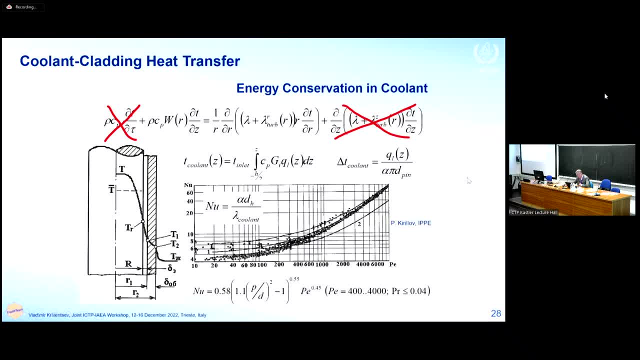 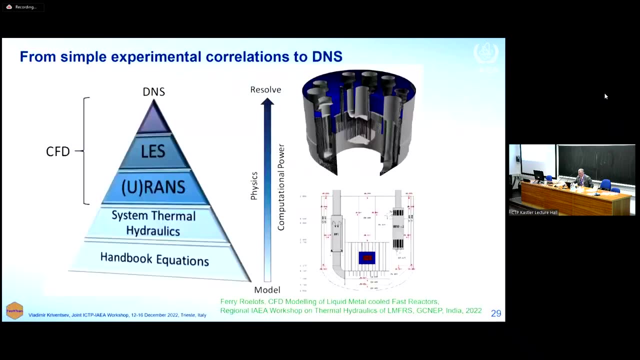 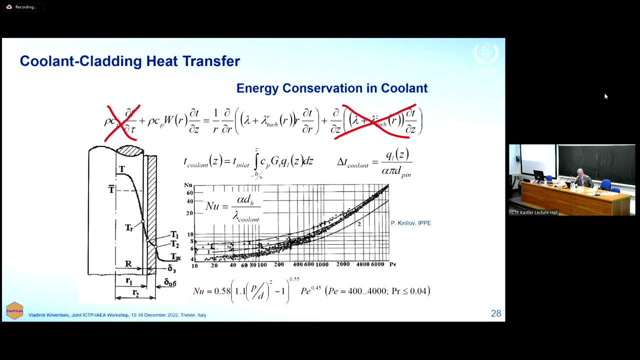 experiments for the nusselt number and for the heat transfer coefficients, so it's not accurate. but this does not allow you to solve it automatically for the any configuration, because the empirical correlations are given for the particular particular configurations also. okay, that was the difficulties and now i i hope you understand better how to go through. please, please. 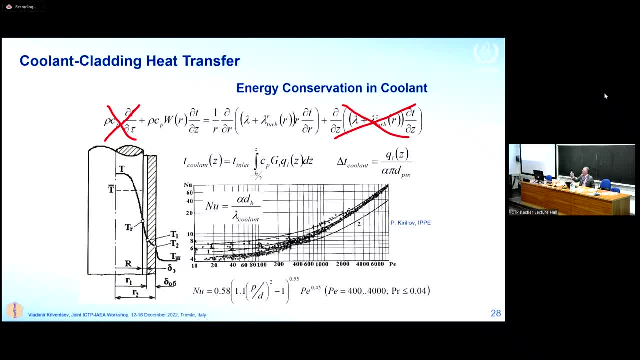 but, but you should please use the microphone. so, because we have the online dimension, please. um, it's just a question about the the gap thickness. here we have, uh, the fuel pin diameter is 9.7, the cladding thickness 0.5 and the fuel pellet is 8.7, so it's like there's no, no, no gap. 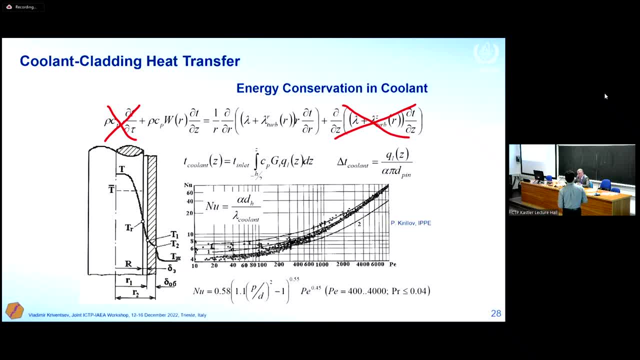 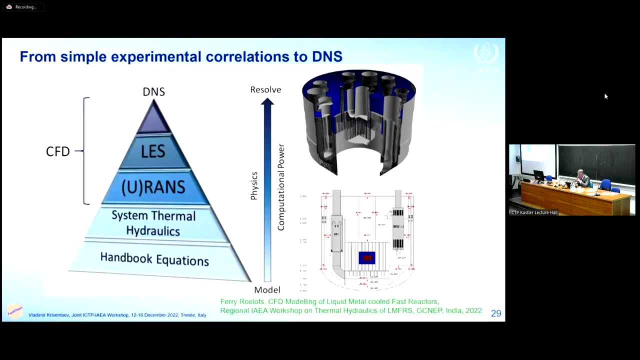 in this axis and that exercise, we decided to neglect the gap, so it's zero. so, to make life easy, for the gaps, no, but for other things, yes. okay, that is a simple equations. and what people say. how do we calculate this? basically, principle, using, let's say, handbook equation. that is very accurate. 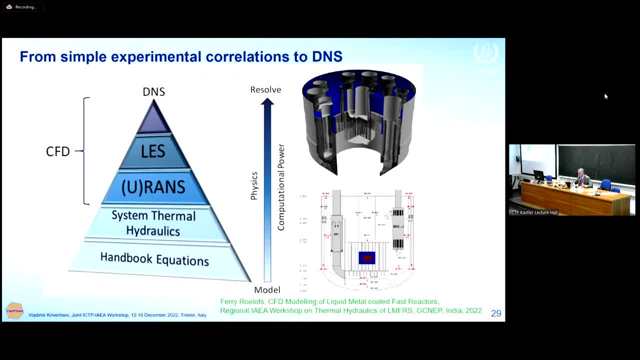 method, also because it's basically from the balance of energy and nothing else. uh, but since it's, let's say, first initial estimation for the first iteration of calculation, because the system itself, including the reactor, core, reactor vessel, and there are many flow passes, you cannot calculate simply using these empirical coefficients and you can have some. 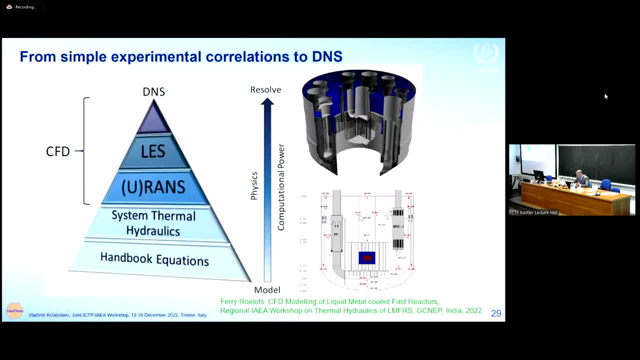 approximations or evaluations, how much you can have outlet temperature. but you should know how does it mix, how do you receive these functions. so it's a very simple calculation. so let's say this total what? because it's three-dimensional structure. also, you should know what would be the inlet temperature for the heat exchanger and 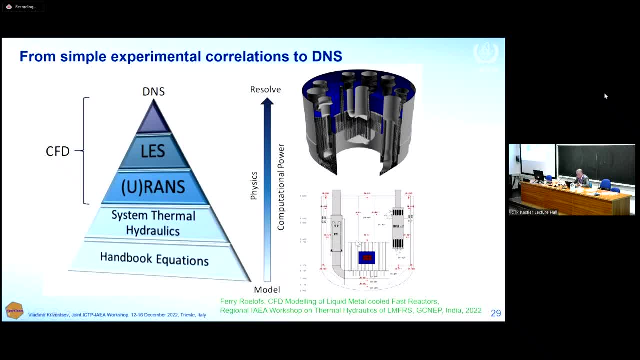 outlet temperature, how the slope paths go, how these jets of the coolant when they release it from the fuel assemblies, how do they mix, and there are many, many effects that you cannot simulate manually, let's say with handbook equations. the this slides I took from the presentation by the expert in CFD: 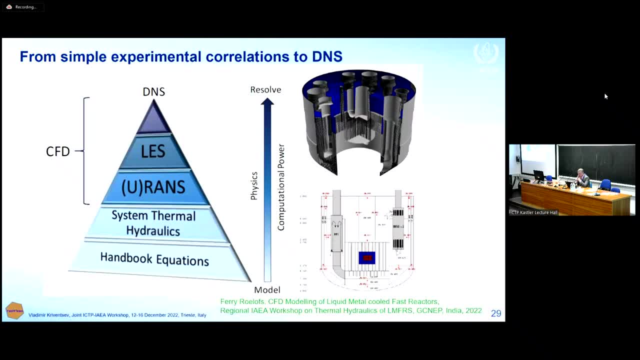 fairy rose on the in the regional workshop on the thermal hydraulics of liquid metal cooled fast reactors in India two weeks ago. so he calculates. you see the split, this, this, let's say the levels of the calculation handbook equations at what we consider, then systems on hydraulics and then CFD. 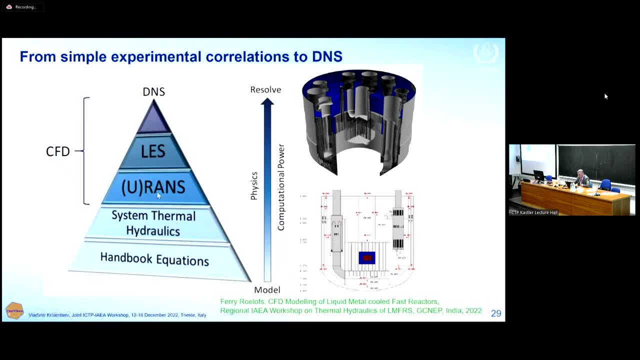 approach which we talked about them a little bit later. it is this all CFD and in more details, require more and more CPU time. let's say now cannot be applied for the whole reactor, Even runs cannot be applied for up, applied to the whole reactor core, including, I mean, flow inside the small. 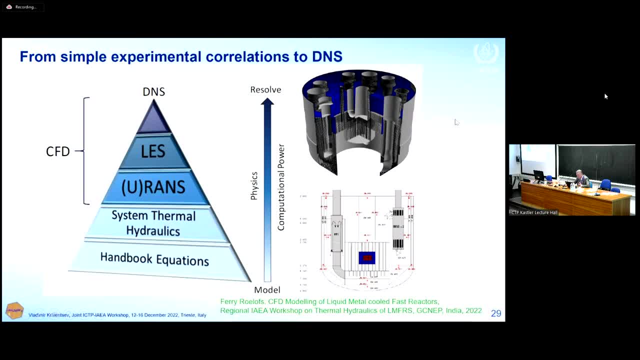 thing. this is too complicated. we need billions of mesh to resolve. is the necessary completely impossible now, very, I mean, and will be impossible, I believe, in at least 100 years more, because it's still required too many measures to simulate. if you want to simulate the whole reactor core, all reactor vessel. 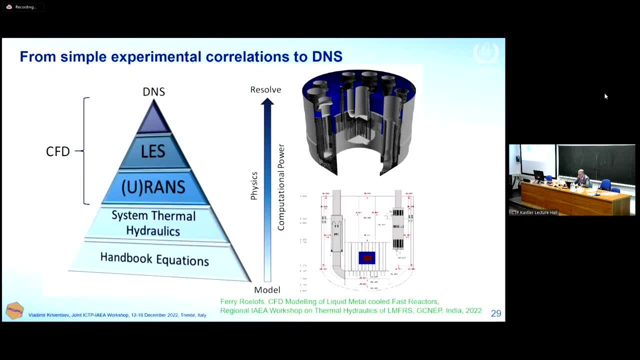 is even the core only business is request too many computational power, but it resolves the physics and gives you more details and more curate. okay, but we have to stop something at some point. and here's a very actually no systems. is a system through my doors or relative raised operation in between, in between. 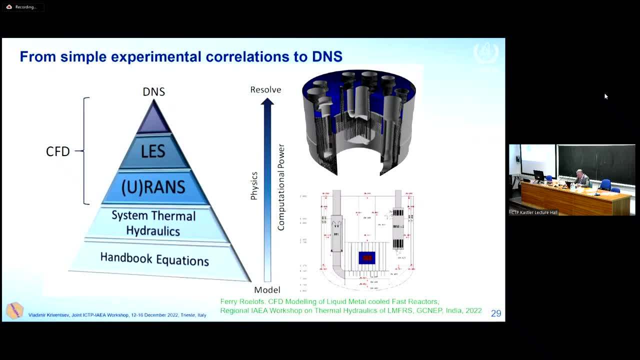 you have so-called sub channel analysis, which we'll talk a little bit later. so again, and systems from my doors: you calculate, simplify, it's more or less one-dimensional simulations, all. when you sit up, this, your measuring system: along the flow path, flow passes in your core. 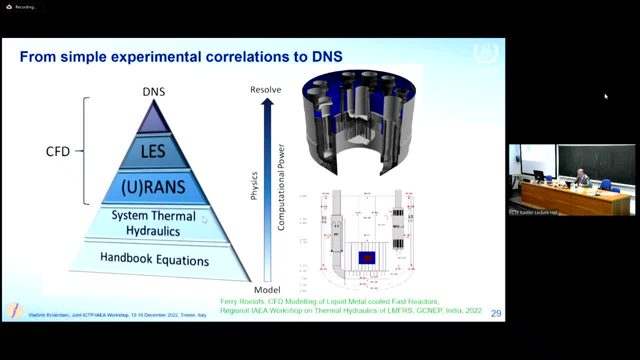 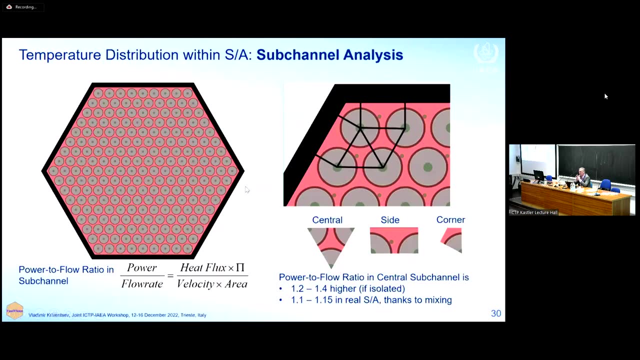 sometimes using as a quarter, as a parallel systems, and okay. and then you apply CFD, which is also difficult, very difficult to apply to them. then we have the system, but one first step it's to apply sub channel analysis for the core. if you look at this, 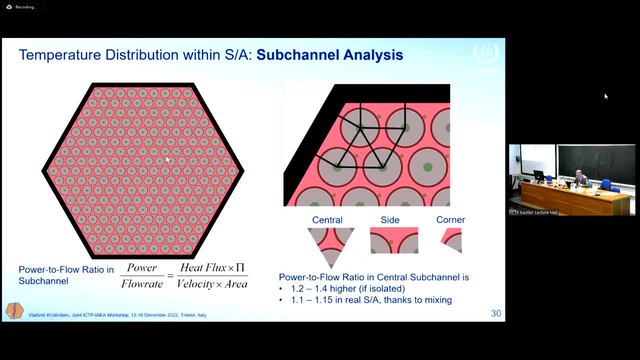 geometry of the fuel assembly. you see that this is not in infinitive array of the triangle, allocate pins allocated in triangle array because it has walls as convulsed. and if you look at the so-called sub channels, here you have a central sub channel, standard sub channels which we are simulating. 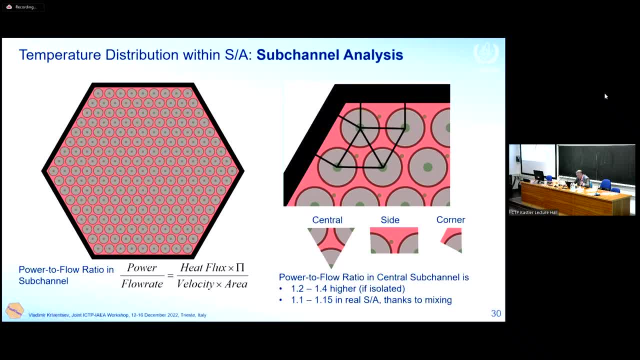 choosing for simulation in our task exercise yesterday. but we also have the side sub channel and corner sub channel which are smaller separately flow passes for the side sub channel area is much compared to the perimeter of the red, perimeter of the walls is much higher and it is itself much higher than area. 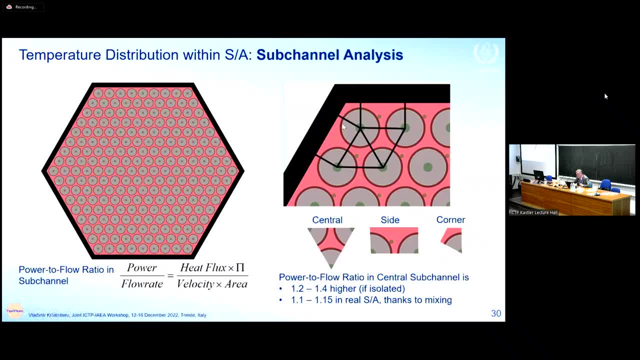 of the central sub channel, but power- it's half of the pin- is also released to this area. it means that higher area and because of the bigger hydraulic diameter it has also high velocity. so in there and in general in the sub channel, in this side sub channel you have higher flow rate and the same 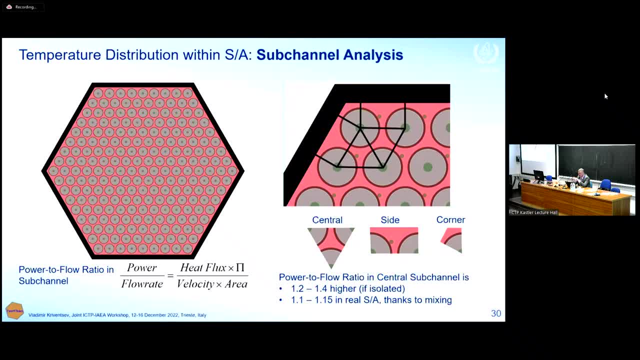 power is released from the half of the pin to this area. that means you have cooler coolant temperature of air. you apply staircase of M 12 and somehow have to apply to these twoatz holes. here temperature of the coolant is lower than in the central sub channel. 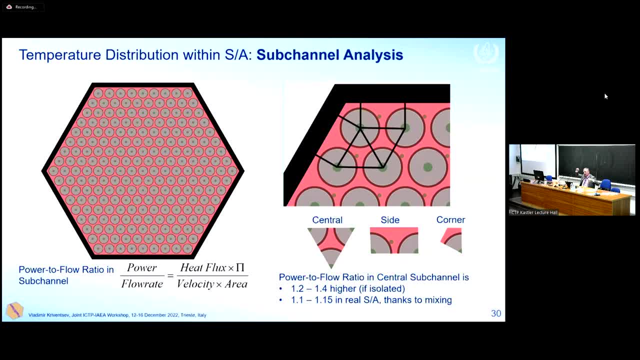 In this case you have like low temperature at the side and high temperature on the other side, on the other side with uh, so-called corner sub channel, this small one you can see. this is also different. I would say it has once one six on the pin. 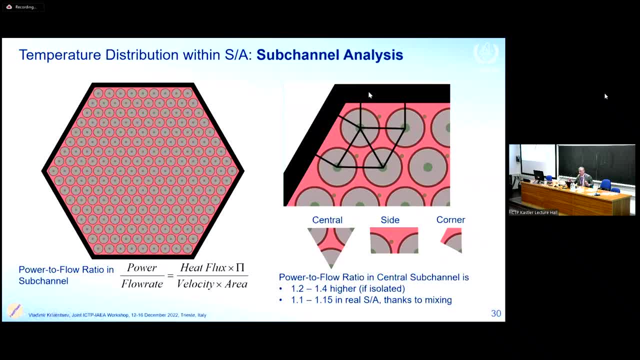 but also much smaller area, depending on configuration It can be, the relation between flow rate and power could be different, but the generally in the side you have lower temperatures, Fortunately, or I know, uh, you have this wire and you have a mix. Also, if we're mixing between the central 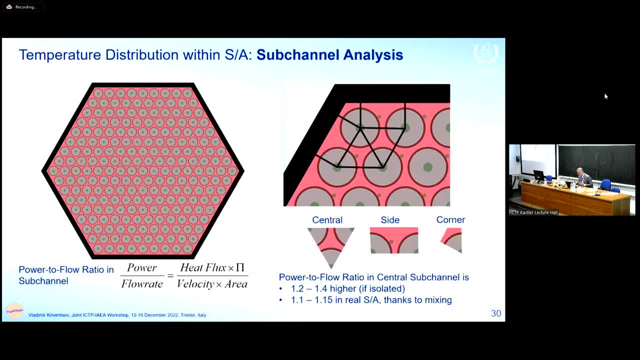 so the, actually the temperature difference between central and peripheral sub channels are not that much. but you need to calculate. you cannot assume something. If you assume something with balance equation, you you will have very low temperature, actually much lower than in the reality in. 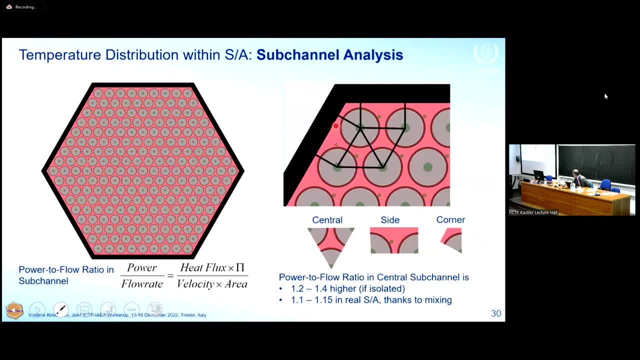 the much lower temperature in the peripheral side sub channel than in the center. So to calculate this you have to use this. uh again, see you calculate it. You can in principle now calculate with CFD, with Reynolds, over age or Navier. 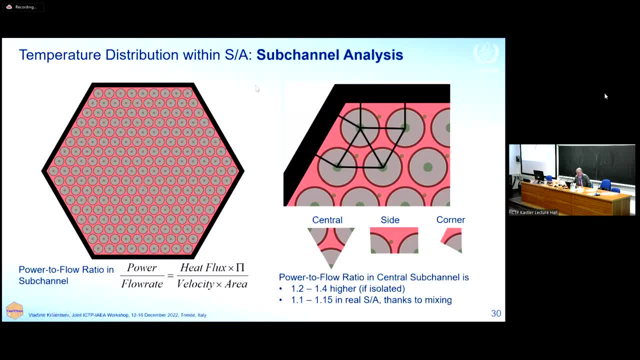 stocks equation. but there is a more easy method, which require less computational power and rely on the exact experimental data obtained for this kind of sub assemblies is vertical sub channel analysis, In this case the energy equations integrated over the sub channel area, and then you solve. 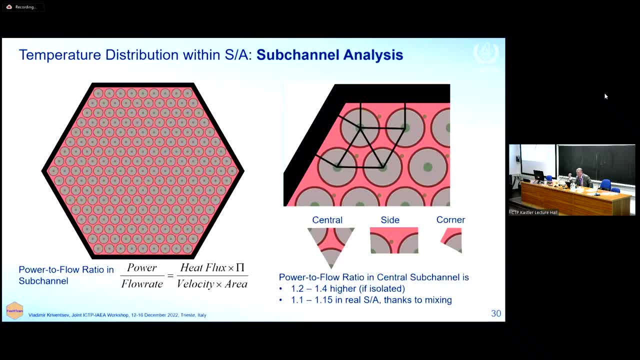 this and using an experimental data for heat transfer coefficients And mixing factors between these two as a- uh, let's say, boundary conditions. it's like transport coefficient between this to between this adjusted sub channels. Okay, This is one way And it's already. 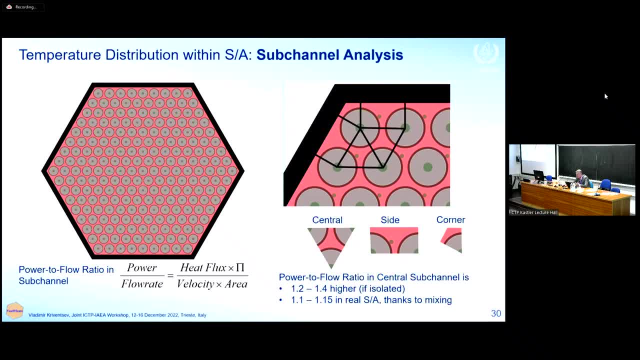 it was done 30 years ago and it worked well and now it's improved. But again now, in principle, CFD allows to simulate all this In some, with some approximations, of course, all this subassembly. but from the other side, sub channel analysis now allows to simulate all the core. 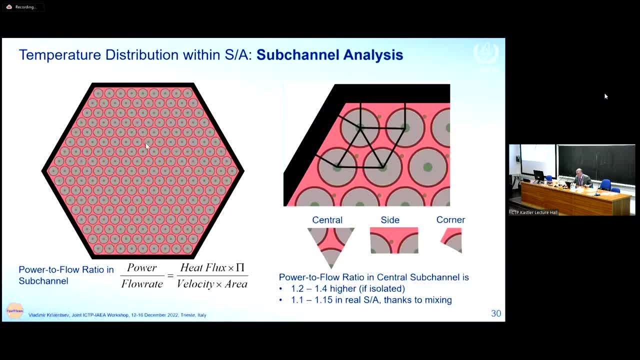 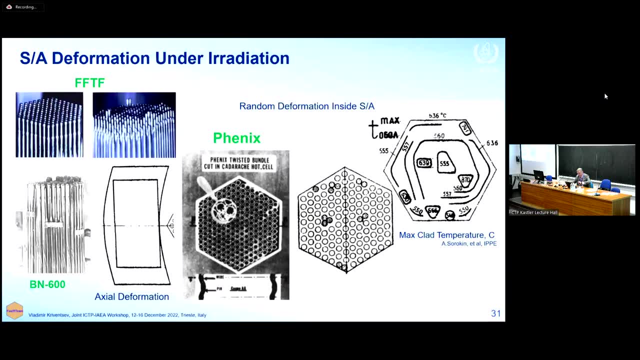 all subassemblies in the core of the sub channel analysis, while CFD is impossible to do this and include this in peripherals, and look what is complications here also. Actually, if you have this pins after irradiation, this is for the fast flux tech facility in the US. 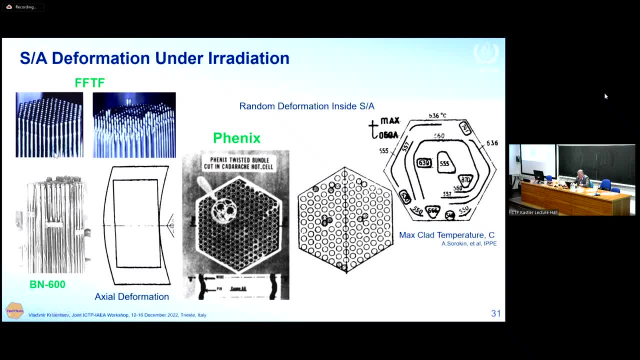 This is the photo of the fuel assembly pins before irradiation and this is after they swell. they change the sizes and dimensions and like randomly. you know, it's not, we don't know why. By the way, these two here, a couple of here, a couple of here, some of this uh, 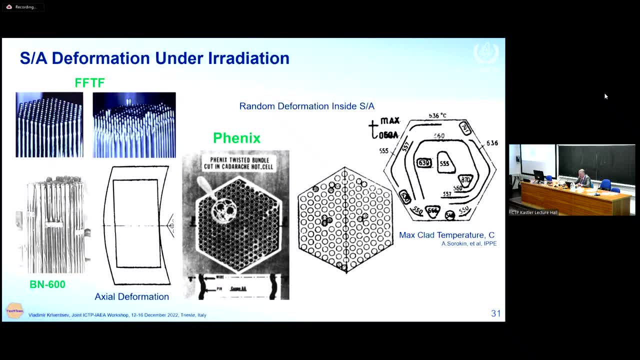 they were extended in size such random, maybe because they have some tools, non uniformity in temperature or like this to touch. We don't know, but randomly we have this change. So this is not ideal. The angle array of of of pins. 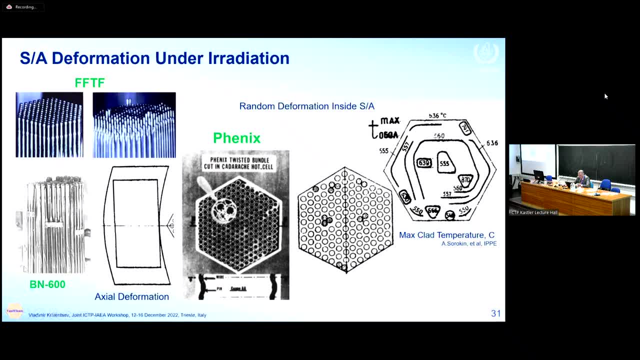 but in reality it could be different. This experiment shows similar photo for the BN 600. you see there are several pins which are get out from this And also uh due to the temperature, uh differences because we have also different power distribution. 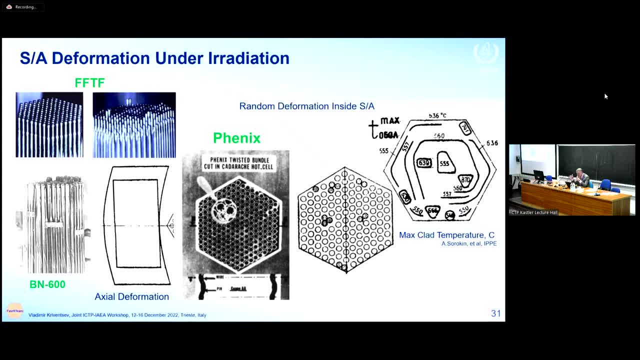 then then we have the different temperatures for even within the sub assembly. This actual sub assembly can change if temperature here is higher than here. So you can change in this location. So all structure of the sub channels can change and also can change as a geometry. 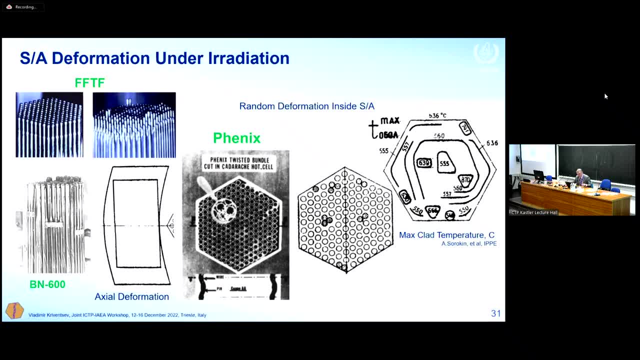 and can change The flow and temperature distribution, For example. you see, here you have very huge opening and gap means you will have much lower temperatures here, Even with mixing, you can change it. It's a photo from Phoenix reactor and that means it may even increase the differences. and also from Phoenix. 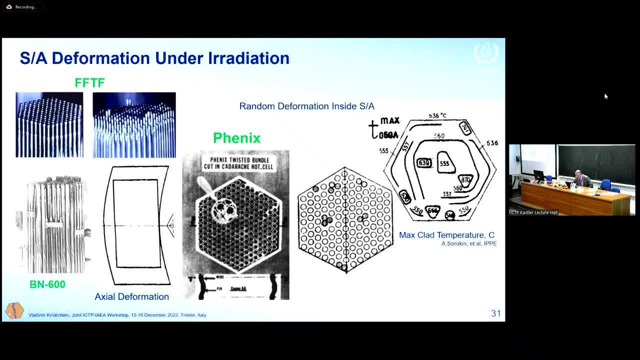 You might see that some pins touched each other. I don't So. so why I didn't? didn't serve Its purpose to to split to to distance fuel pins between them for whatever reasons, because of in case of radiation, So you can have picking temperatures for this. 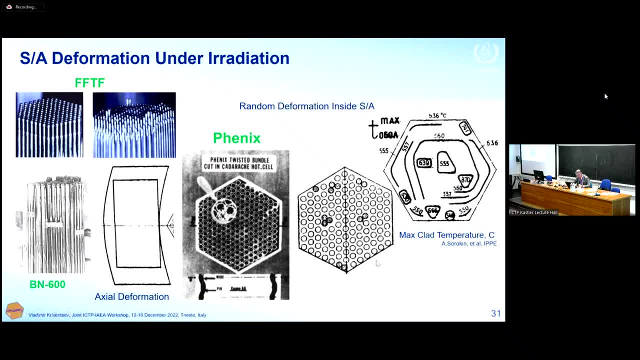 You need very complicated simulation, is a, with sub channel analysis probably, but it's it's also the only first approximation, but maybe also in this CFD in particular areas. So here you have the touches, So we will have high temperature. 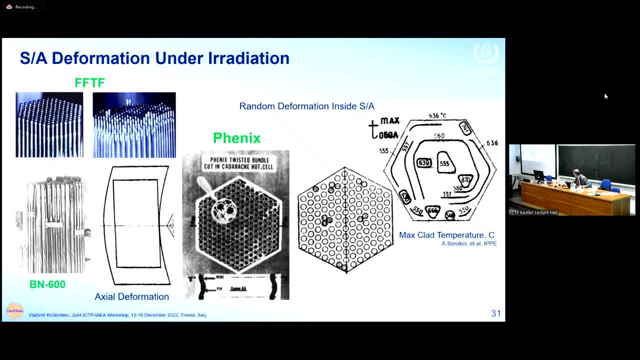 temperatures, very high temperatures. you see, if a woman, I think, is very high temperatures here and lower temperatures here, that is kind of distribution calculated with sub channel analysis. you might see the maximum temperatures here. I believe it was this sub assembly was 870 degrees Celsius and that could be. 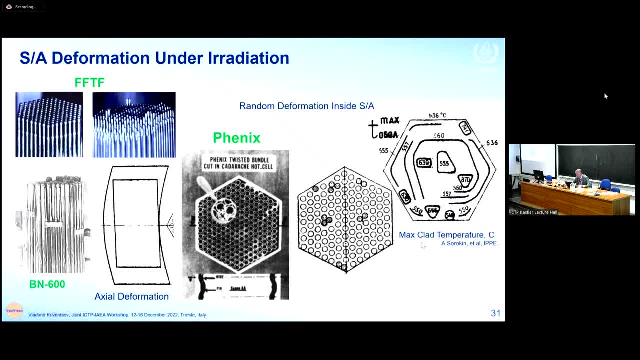 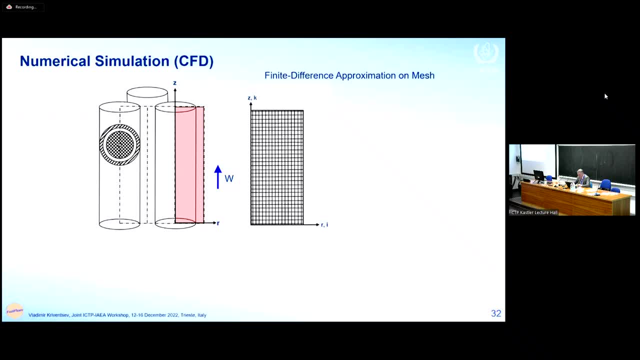 the reason why they can expand differently in different locations. that requires more calculations. okay, now let's let's see how can we do this numerical simulation of the same sub channel. we already discussed it in this triangle pinery. so we can split. so to do numerically, we split in the mesh, we 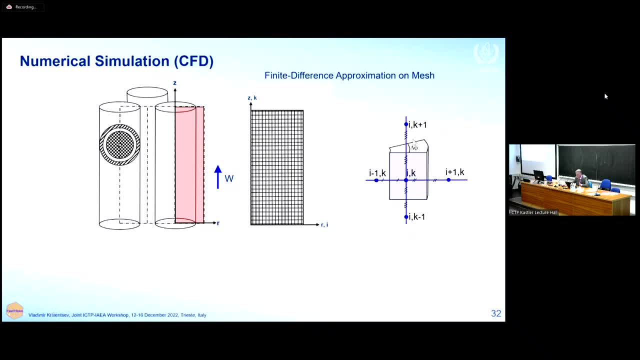 select the so-called, so-called control volume or the small minimal measure sizes like this one, and we apply energy equation, now I'm- and also Navier Navier stocks, or let's say, momentum conservation equation, to this small volume of of solid material or small volume of liquid. okay, once we apply this equation to this small volume, 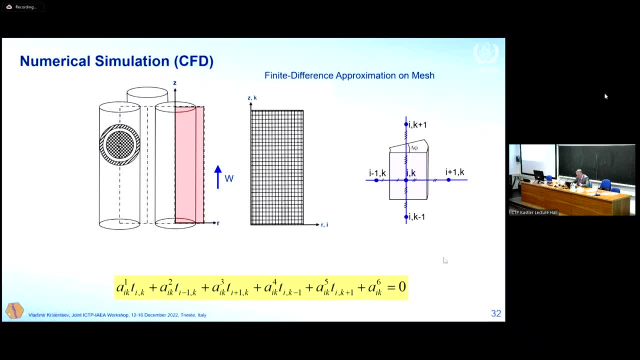 you can obtain the so called algebraic equation for the discretization of this so, which reflects the initial transport equation in partial derivation. so once you have this algebraic equation, you can solve it numerically. again, not analytically but numerically, because the Gaussian's matrices to huge商ierry. 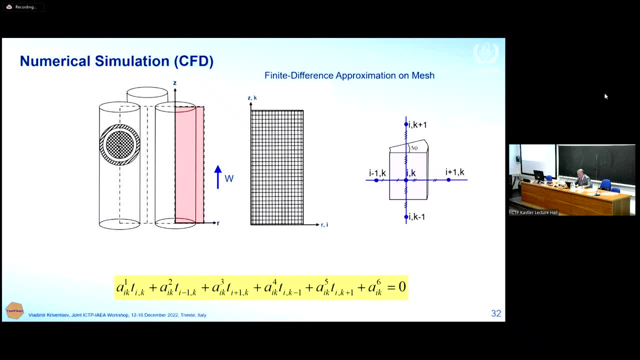 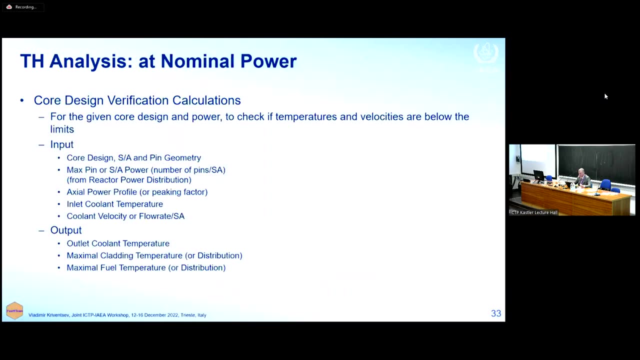 hypothetically, I would say you can solve it also analytically, but usually we use numerical method, iterative numerical methods to solve. then, once you solve it, you have distribution of velocities and temperature in this small control volume. and this is how CFD it's, just maybe it's, I know it's for introduction- the 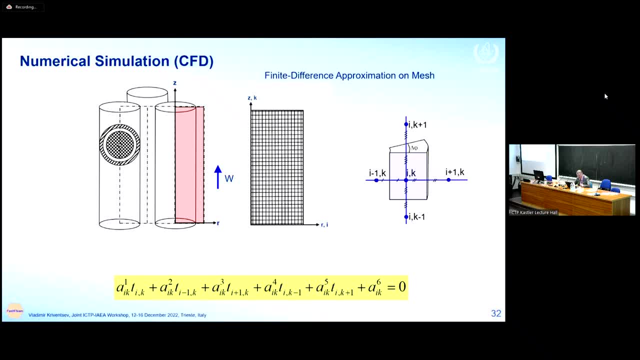 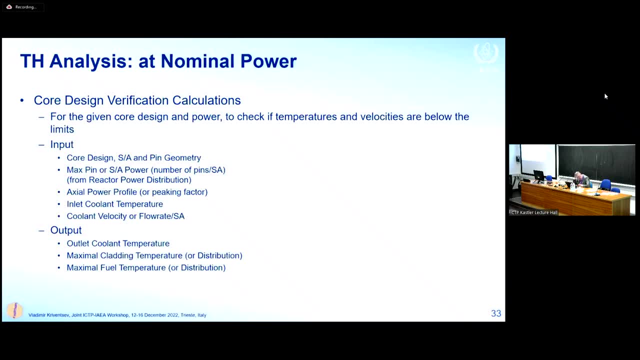 numerical methods to explain how is CFD works. but of course it's more complicated and requires long. you know, course, of the lectures on how to simulate this. okay, maybe already notice it yesterday that we can simulate conduct the thermohydraulic analysis as a nominal power. so for the given core, 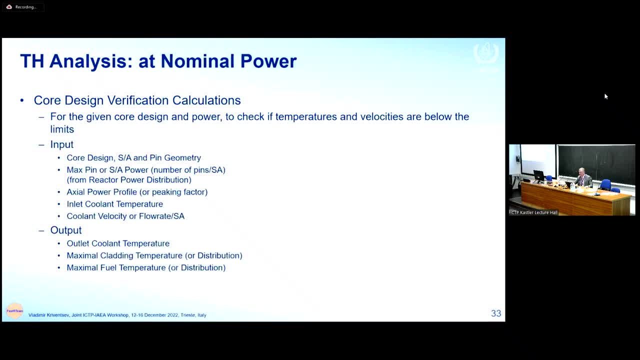 design for the given power, as designed and provided we. the purpose is. objective of this analysis is to check if temporary temperatures and velocities not exceeding the given limits. so for this you have input of the design of the core and geometry and the core and pin geometry. you need number of the pins and number of subassembly in the reactor. 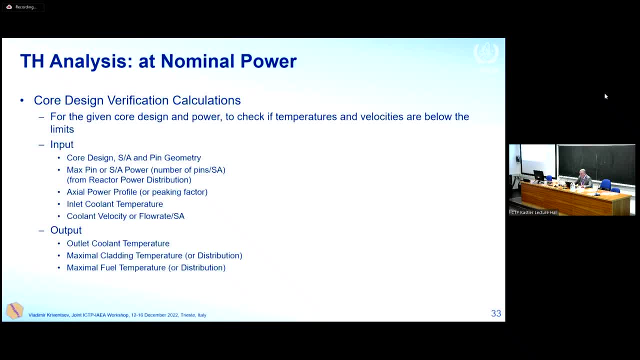 core. you need to know the axial power profile or picking factor- at least you also need to have this inlet column temperature and also you you need know the cool velocity or distribution of the cool velocity and flow rates through the sub assemblies. as output, you calculate out at cool temperature maximum. 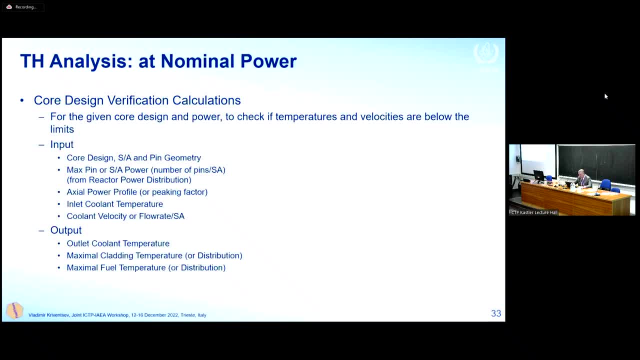 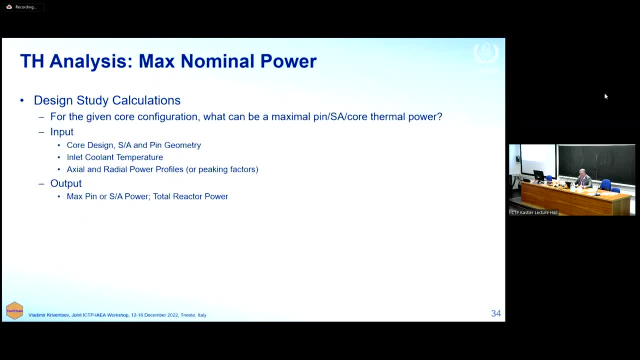 closing temperature or distribution of the temperatures and maximum field temperature or its distribution, okay, and if you want to conduct the study of the design, how much for your career can survive, you can. it's. there is other opposite calculations. when you again have the core configurations, you should. 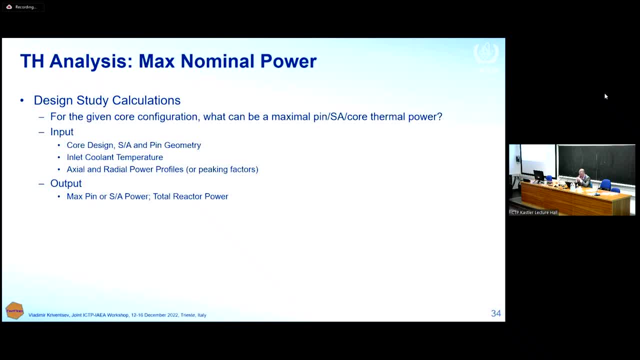 define the maximum reactor power, which on which the temperatures and velocities will not exceed the maximum values as well. this is kind of test. of course. this is not like core designers invent the design and then give you please check. this is like iterative process, of course it's know the temperatures and they decide. okay, should we reduce the? 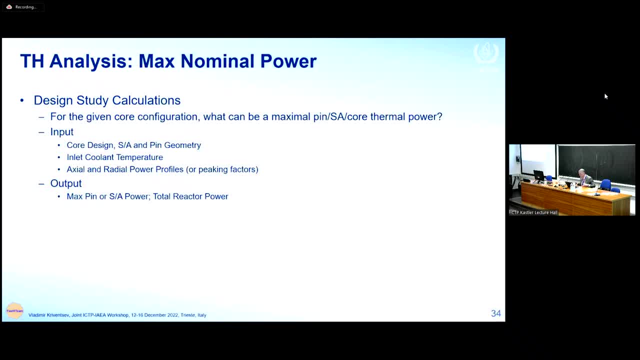 diameter of the pin, or should we expand the diameter of the pin? so this is kind of iteration process and let's say the part of it is thermal hydraulic analysis, but of course it also includes the other calculations. power distribution it's given by the initial neutron simulations, but since the materials properties also 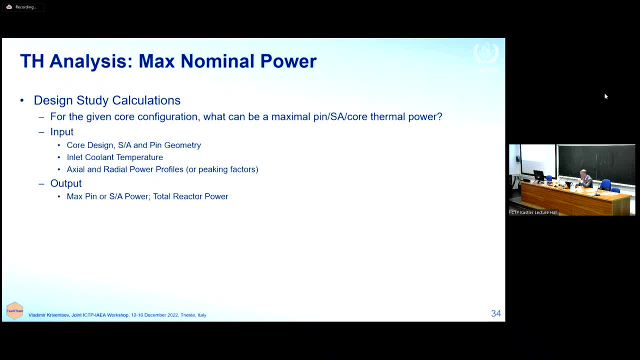 depends on the temperature and the reactivity depend on the temperature. Once you have temperature distributions you give it back to the neutronic analysis and neutronic analysis simulation codes will recalculate the power which can be now adjusted in some hydraulics and so on. 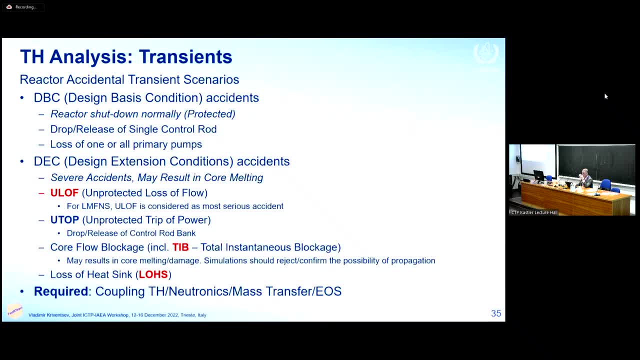 And from structural material changes in geometry. expansion of the pins, for example, also could be calculated depending on temperature, and then with expanded new dimensions you have to recalculate neutronics as well. This is one part, but when we are talking about steady state analysis, 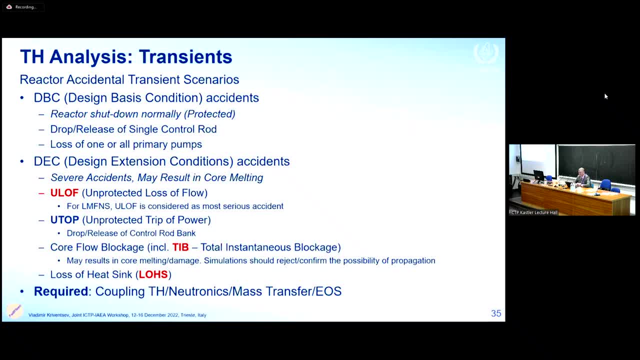 But an important part of the thermohydraulic calculations is the transient, because the steady state is more or less given. You even can calculate the steady state parameters without using any CFD, only using the basic or, like Ferry says, handbook equations to calculate this. 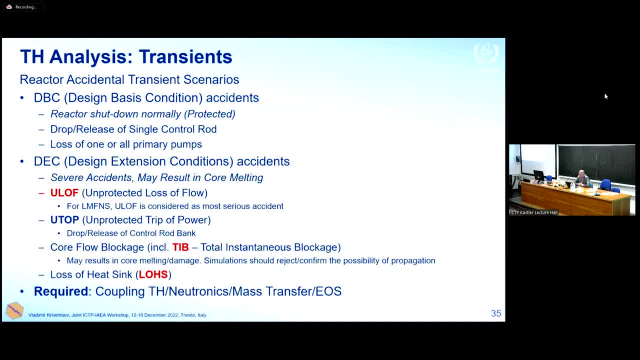 But to calculate potential transient, which can be standard transient, reactor shutdown or heat up, you also should, during this transient in the standard condition, you should make sure that the temperature gradients and temperature increase will not exceed certain limits, like, say, 10 degrees Celsius per. 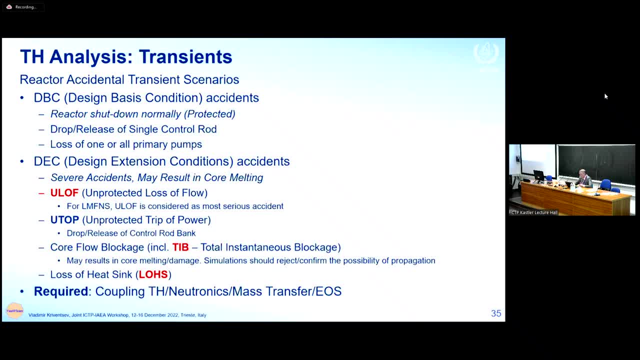 hour or whatever something. So to start the reactor, for example BN800, from zero power to nominal power, you need at least two days. two days to do this and to make sure there is no temperature gradients to smooth. This is, of course, over, you know, maybe, or it's very conservative approach to do this. 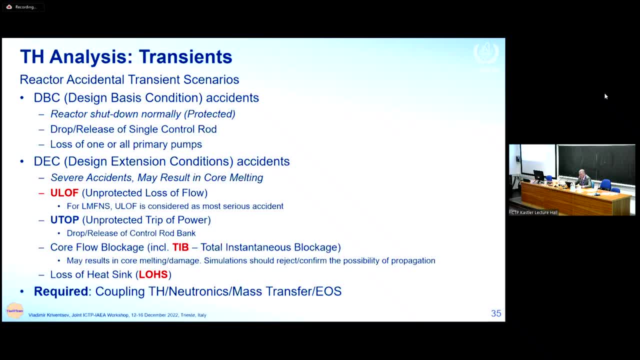 but for this you should calculate thermohydraulics during the transient. This is what you do, But there are other transient. this is a list of the possible transient which subject to thermohydraulic analysis. There are several very important transients. 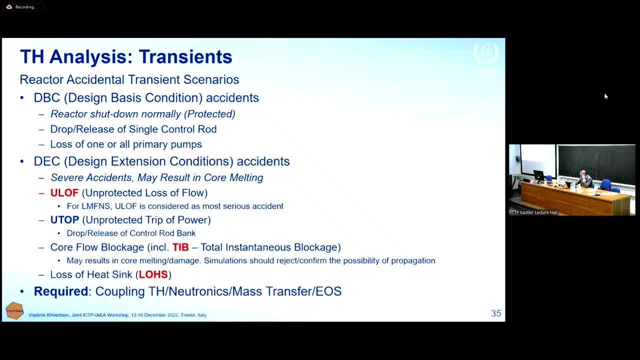 which are not as transient and accidents are not proposed by the design, For example, unprotected loss of flow, which means you, for whatever reasons, your pump stop working and also your safety system doesn't work. So reactor is not shut down by control road safety, control road. 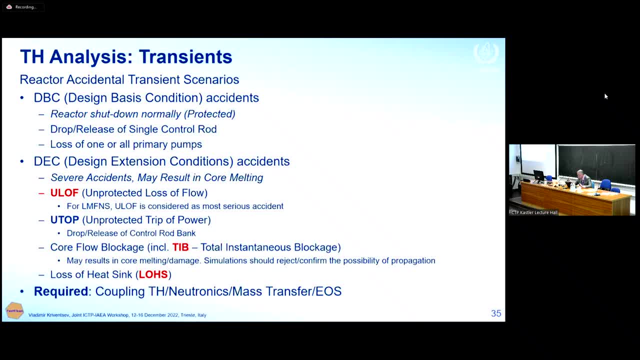 insertion to the reactor. For whatever reasons, it could happen- potentially never happened before, but could happen- And it's this so-called unprotected loss of flow is considered, for example, one of the most important and serious accidents. There are other types of the transient which can, which requires this thermohydraulic analysis. 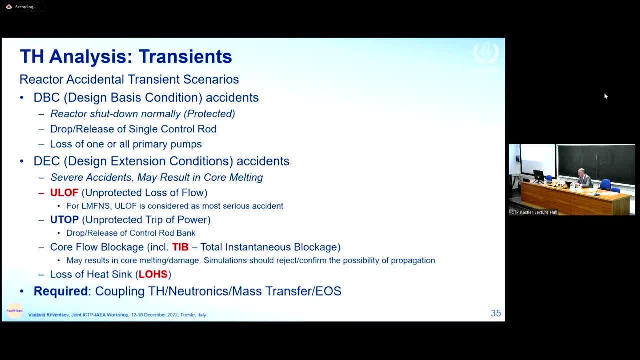 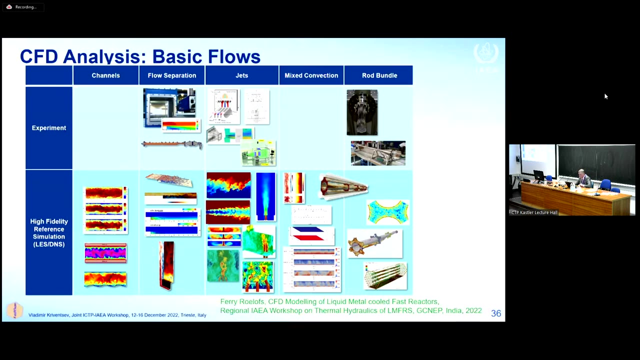 and we have to do this to understand- And this of course cannot be simulated by hands or by handbook equations. You need software And simulation costs both system analysis, sub-channel analysis and CFD to calculate this. Again, I took it from the Ferris presentation but I will skip. what kind of flows? 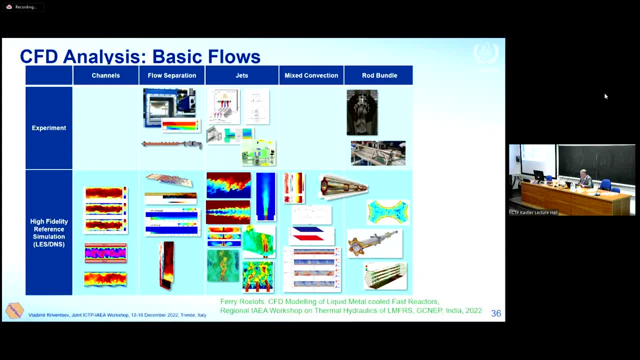 and what is experience we have. We also need to validate your simulation costs. You need experimental data. Of course you cannot do experiments on the whole reactor, especially you love transient. It's impossible. But you can separate effects and you can study experimentally several effects. 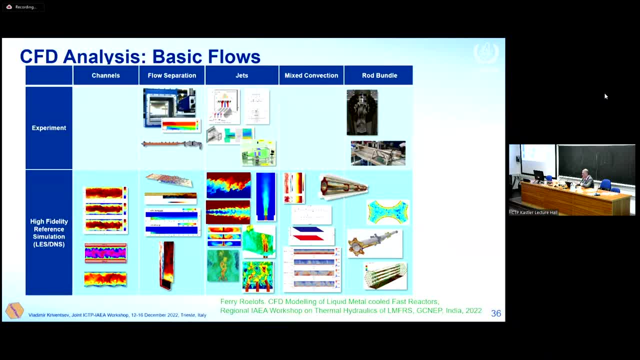 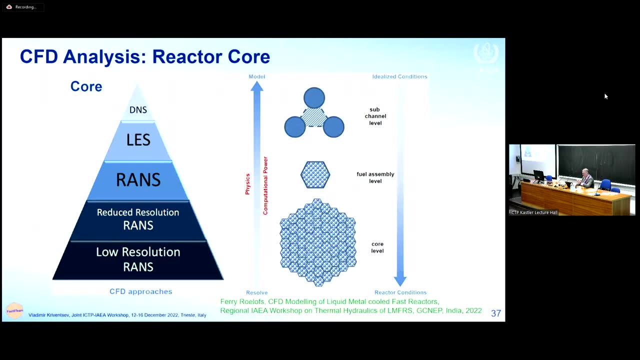 how does it certifications many, many other physical effects and then try to simulate with your computer code and see if the results are matching. This is called validation of the computer code versus experimental data. Again, this shows also the details of the CFD analysis of the reactor core. 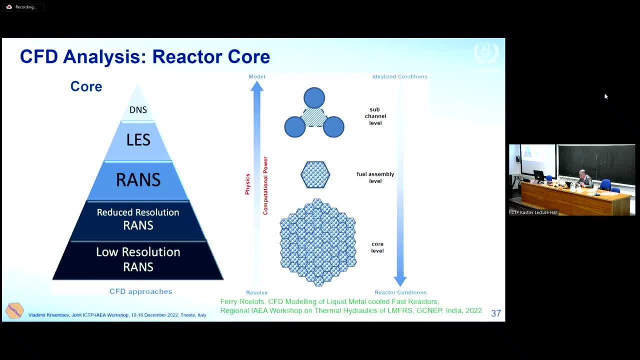 with CFD, pure CFD method. Now we're not talking about the sub-channel analysis and simplified system codes. But so again, DNS is not possible And low resolution Reynolds average are still possible for the whole core, But if you go to the reduced. so for instance, 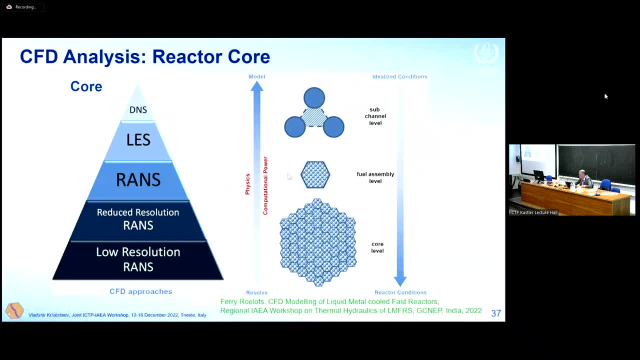 the full Reynolds average you can simulate. probably It will take weeks or months to simulate. But if you want to simulate DNS, you can only simulate this small sub-channel like here, Because otherwise the modern CPU power is not enough And I believe it's now will be not enough. 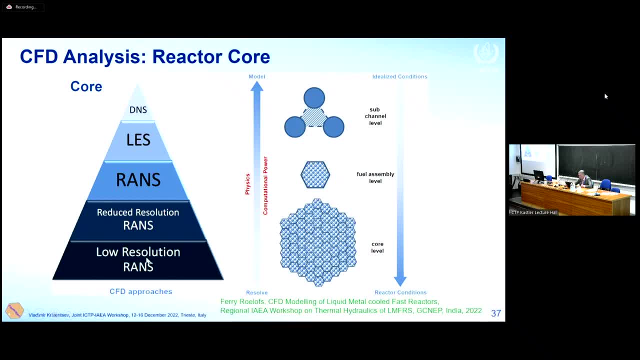 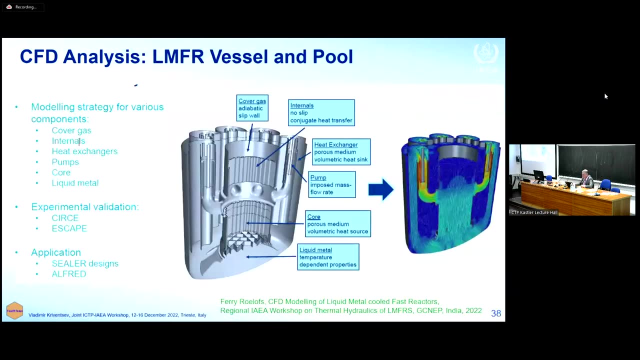 But with low resolution Reynolds average you can simulate your core again at all, But it's low resolution. runs are similar to sub-channel analysis because it's porous media on some. OK, now I have to go, probably to complete Again. there are several types, not only the important simulations in the core. 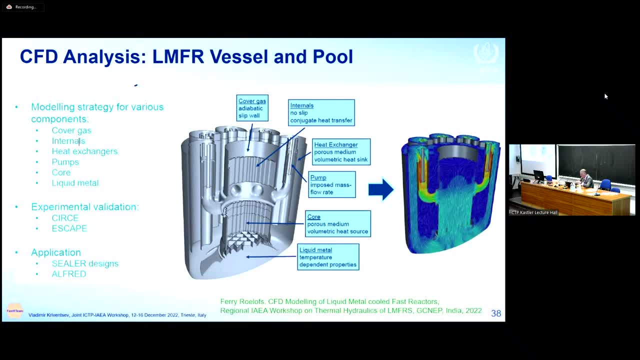 but the effects in the reactor vessel And we have a big pool with several flow passes, which is entrance piping, And also we have many effects how they enter heat exchanger, how these jets are mixed And there are stratification effects when the hot temperature coolant are collected. 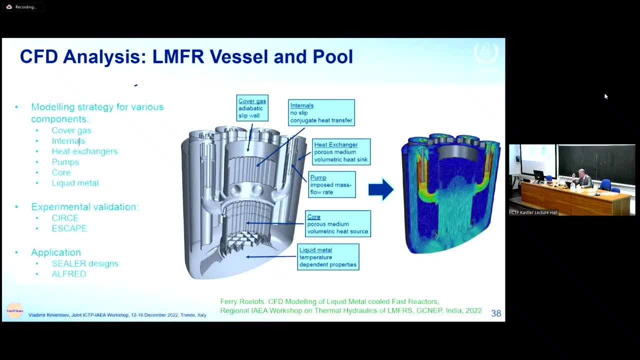 in the upper part, And these stratifications should be avoided because it also it could result in the temperature gradients and other undesired, let's say, effects. So we also can with this. you have to use CFD analysis to calculate this plenum. 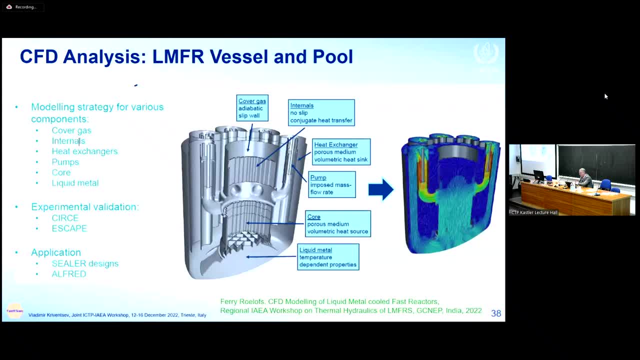 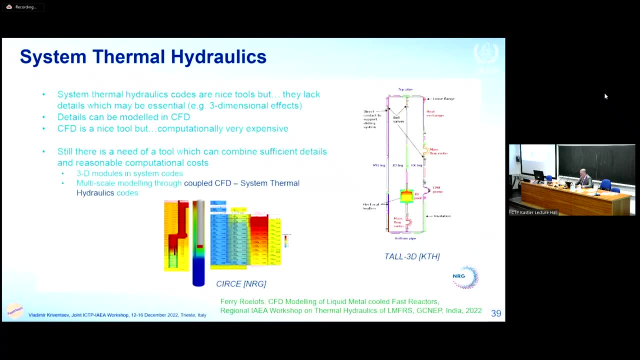 And this is potentially possible And done, But this doesn't. And how to calculate the core inside, it's another question. how to simplify Systems from It's very quick and also popular in many simulation course When you replace all these three-dimensional structures with one-dimensional, one-dimensional. 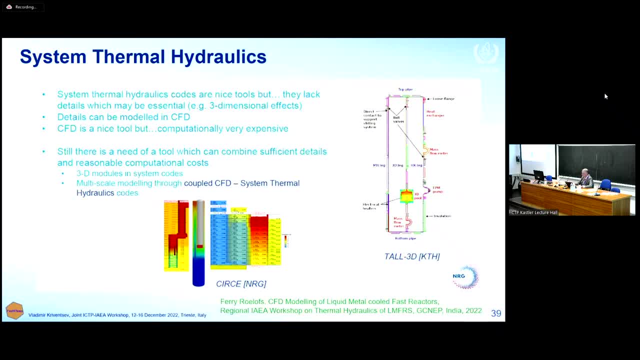 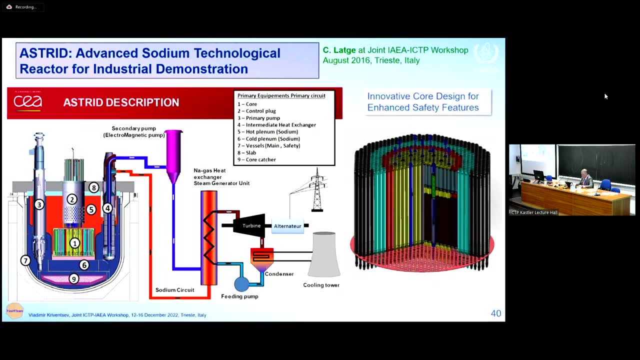 passes, for the main flow passes, and it can be also simulated, which of course is possible. I will skip. now Let me show you. This is the old Astrid code, which is now postponed. Postponed or canceled, I'm not sure. 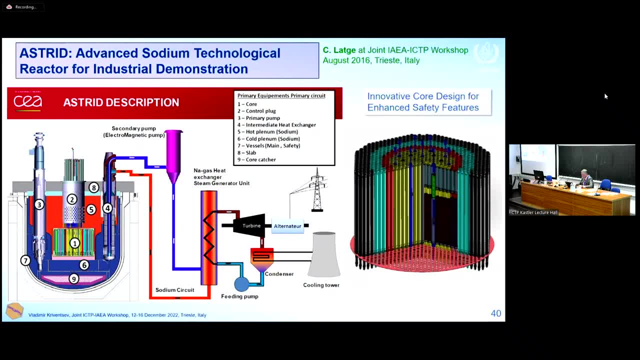 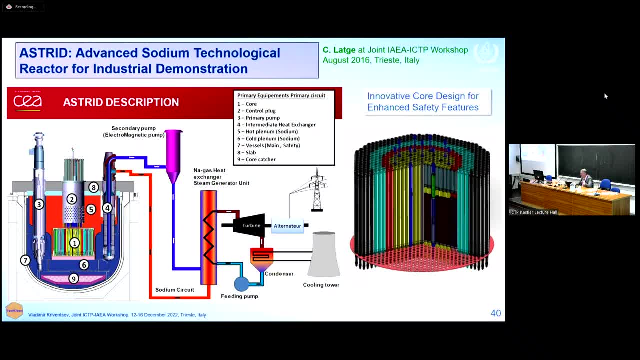 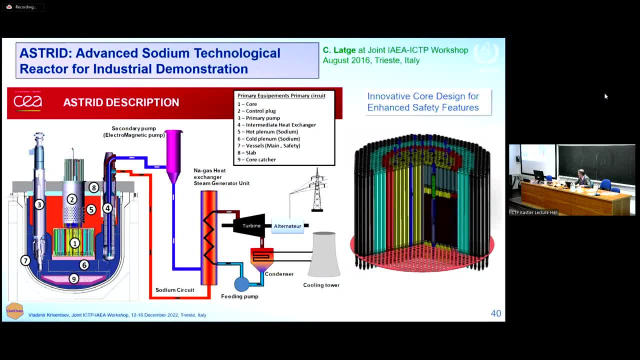 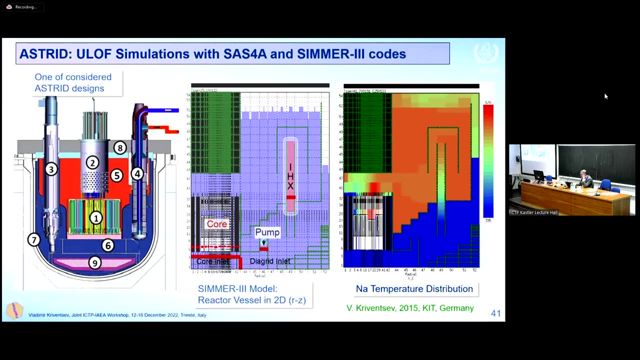 can learn more. I'm sorry also for the online participants. We explained: Okay, This is old Astrid code We can simulate. This is example of simulation of the ULOFT transit simulation: Unprotected Loss of Flow of the old Astrid design with similar code which is multi-physics and includes: 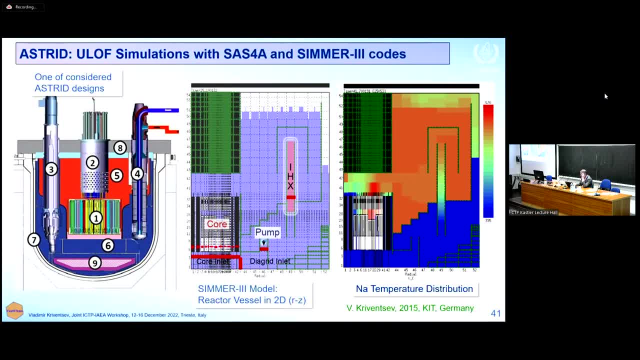 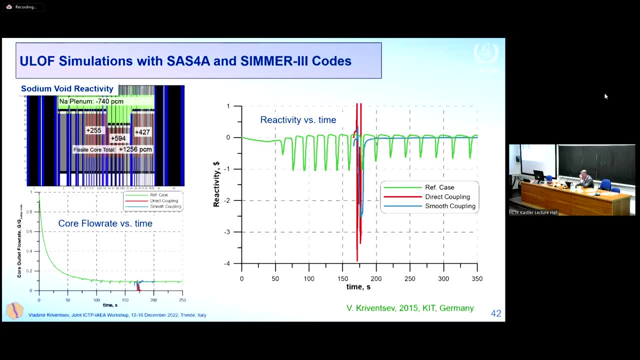 many things. multi-scale code shows you example how to simulate the courier and distribution of temperatures and velocities inside the courier. and since it's multi-physics code, it has also inside this calculations of neutronics so it can place neutron power distribution and neutronics and in this 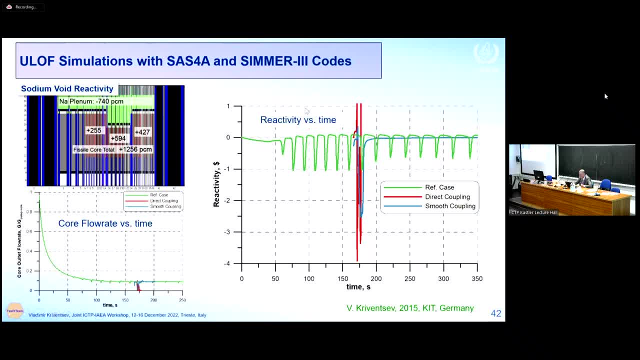 case of transient you can see the simulation again. so when sodium starts boring inside the courier, you have. it gives you a positive reactivity, because here the reactivity coefficient inside the courier is positive. so as a result the reactor power increases later still. we have a flow here because of the natural circulations and the 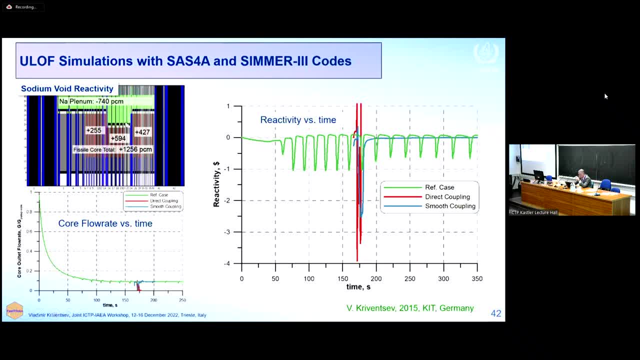 remaining passes from the pump. so when this sodium vapor moves to the upper part, to the upper plenum- because of this special design of the Astrid code they have so called upper sodium plenum here- the void reactivity effect is negative. then the reactor power decreases. when sodium vapor reaches the 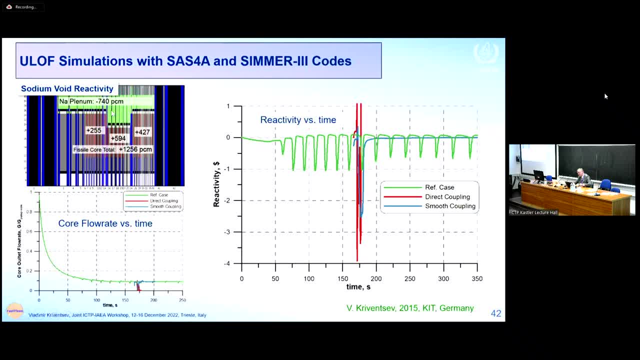 this world and once it decrease it and but does not stop, and that is effect results in this fluctuation of the reactivity and flotation of the power, which can also very uncertain, which can lead to the secondary prompt reactivity of the reactor and and immediate increase of power, several orderful 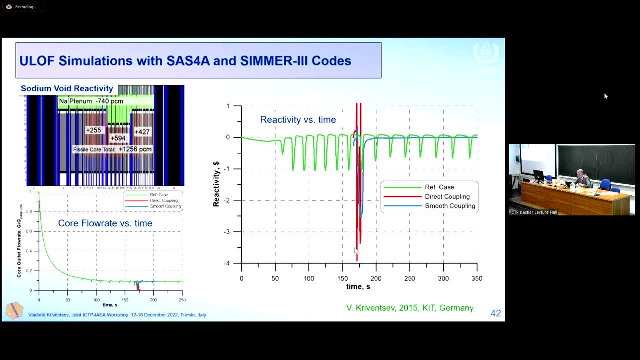 magnitude, which is shut down by Doppler effect then, but in outward stream current and so on. then Mosler algorithm is used here on just sort of standard way of so called constant flow rate and the ME probability which does not stop from the și of P, which is you have now a slice on each speed minus Mach i. 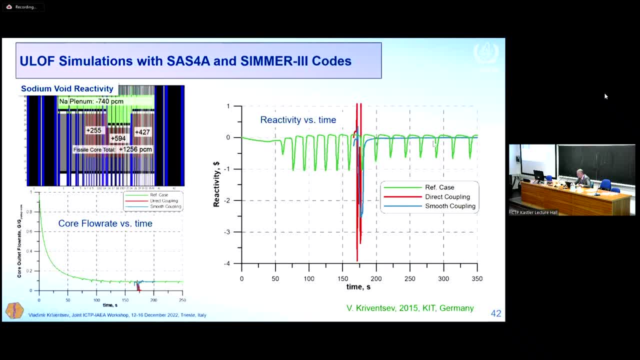 it will melt your core or, dependent on your modeling and simulation, the core can survive this effect also. Uh, this is happens during this. uh, already after 150 seconds of this transient. So means this reactor is a decay. heat is removed by the natural circulation. 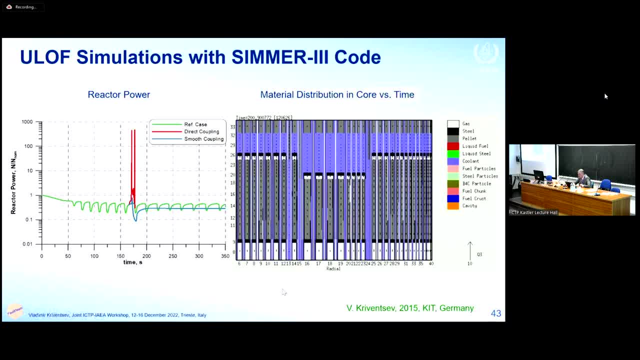 Okay, As I wanted to show you the figure, how- how it looks like. So this is the core. You start. it starts boiling in the in the upper part of the core and becomes a vector, becomes a power increases. But when it's moves here, the power decreases due to reactivity increase. 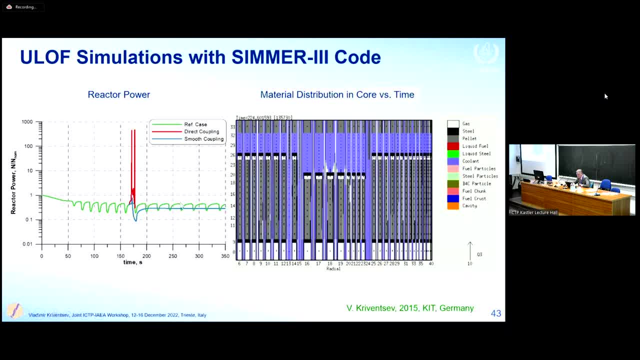 And this is like a periodical effect we can observe, which is, I know at least it does not lead finally to the CV accident. We score them all down. But in principle, if you change a little bit, let's say if you change the coupling of the systems, 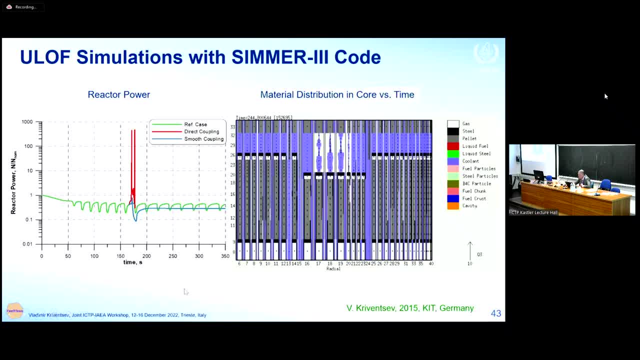 it is uncertain. It's also uncertain. It's not a great, not very precise simulations. If you change slightly something, it can happen that this fluctuations will lead to the also to the secondary trip of the power, and it could also melt. in principle, 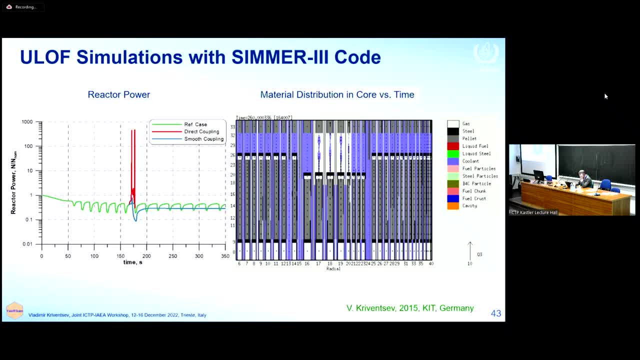 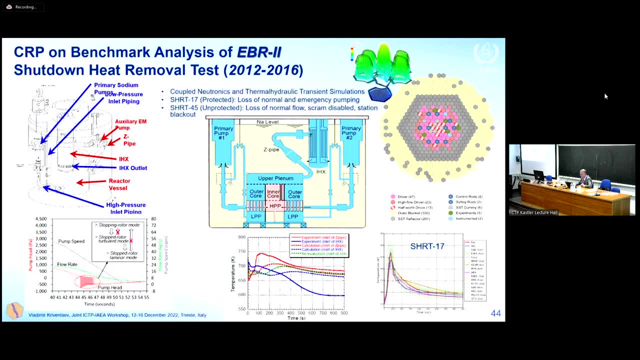 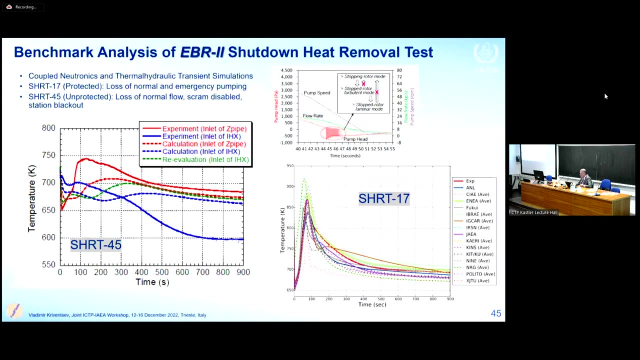 But if you don't provide, of course, the external heat removal for these systems. this is another example how to simulate the complicated areas which was conducted by the I in the IACRP that several participants, in this case we- in this therapy is to test the computer codes of the participants. 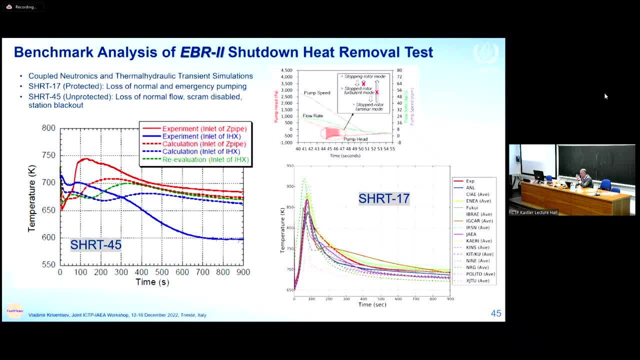 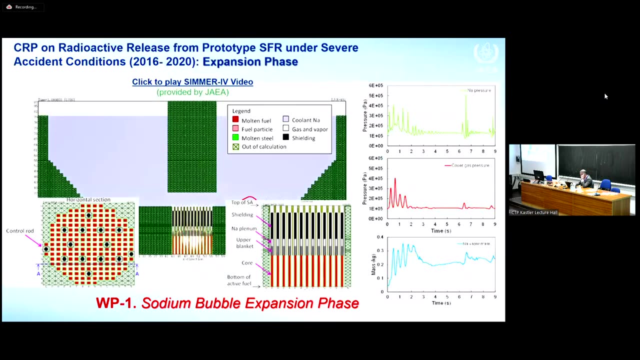 The experimental data were provided after the test, So they participate in blind- so-called blind- simulations and tried to validate the computer codes and simulation models on this experiment. This I showed you already, probably yesterday. It's another therapy which shows how the after the law. 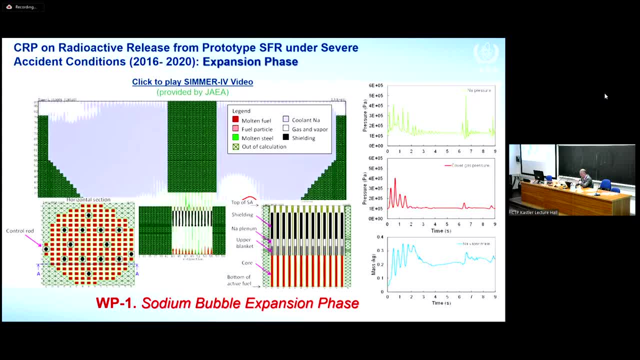 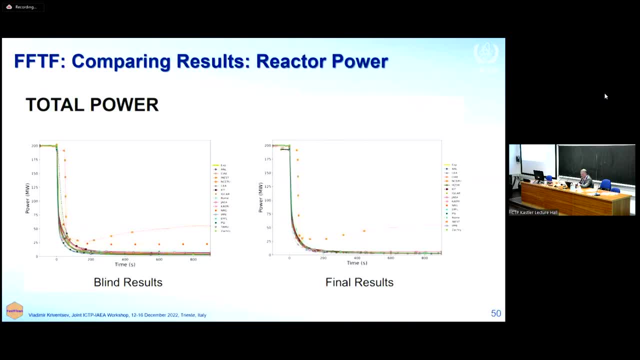 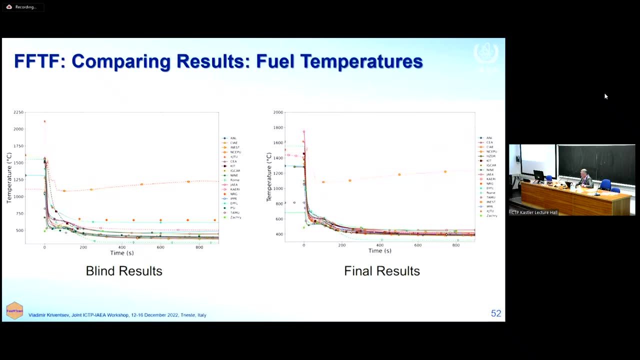 the behavior of the sodium evaporated and condensed in this score And the. okay, let me, I will skip this, but you will see the some results of the thromahydraulic simulations of the several benchmarks conducted by the IA recently. This is also, I show you, the sodium properties calculator, NAPRO. 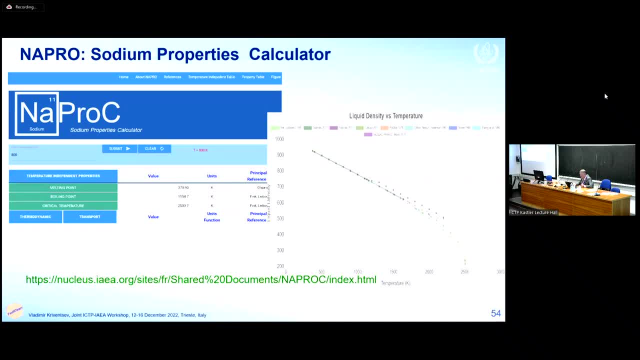 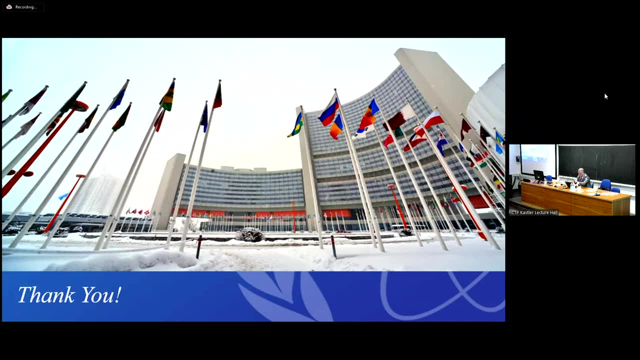 which is now released, and I invite you to try this. This tool, it's online tool. You can find it here. This presentation will be done there, And for this I'd like to thank you for your attention and complete my presentation. 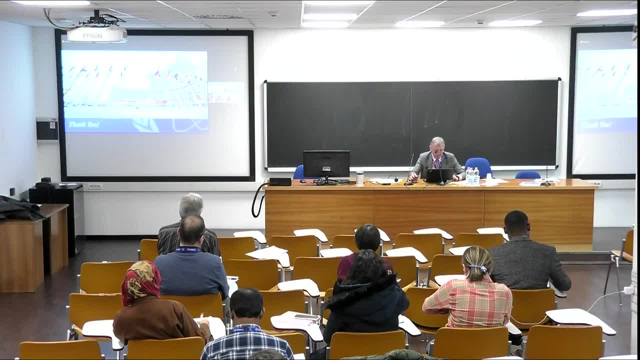 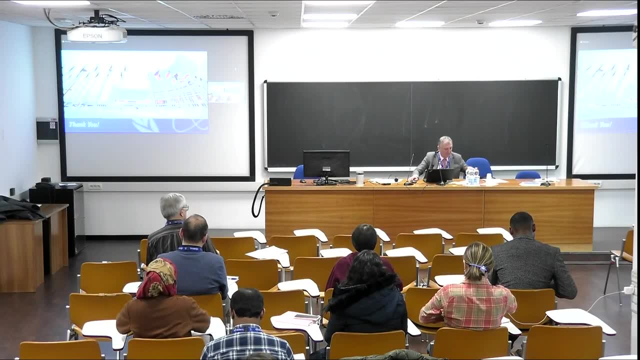 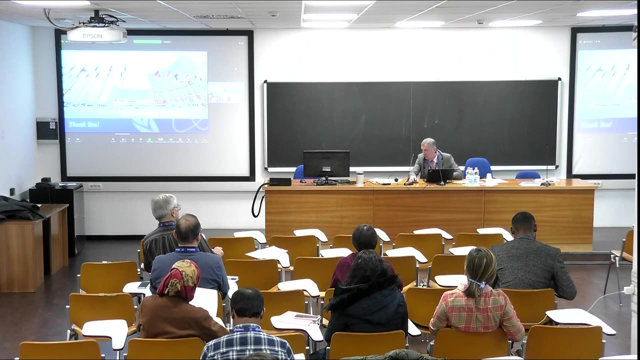 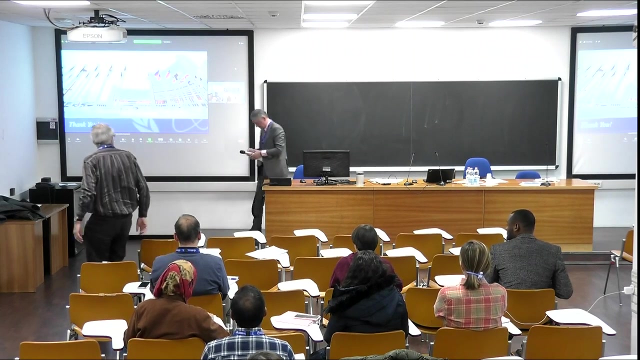 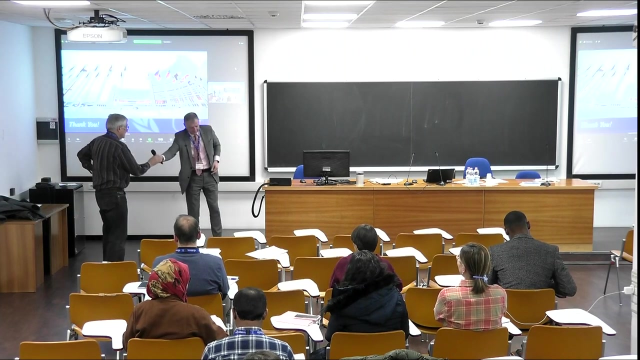 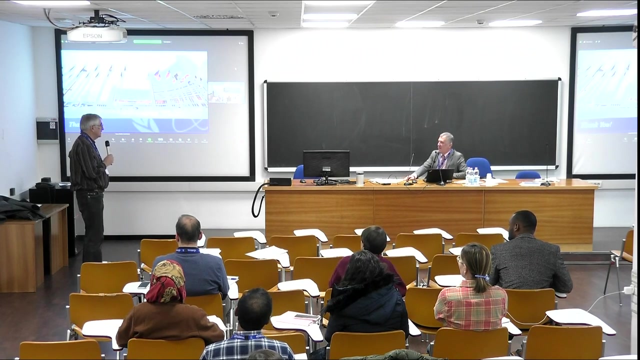 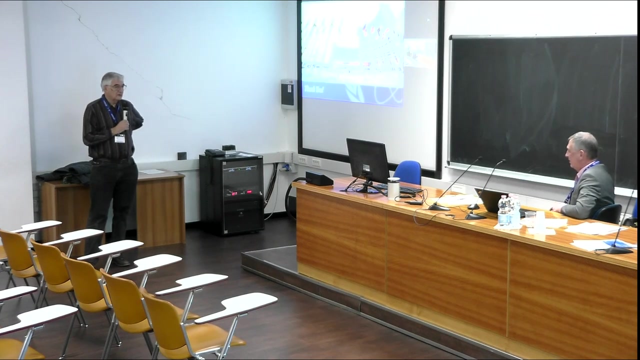 And if you have any questions or comments, I am happy to answer. Do we have online questions? Okay, please, please. Thank you, Vladimir. Just a comment about the velocities of sodium and lead. on one slide You have shown the velocity of sodium: less than 10 meters per second. 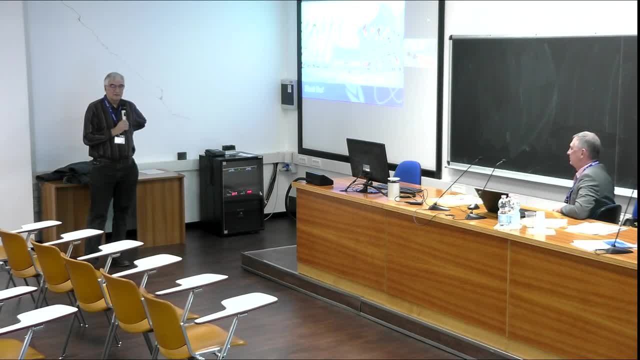 In fact, it's not related to directly outside some kind of physical properties. In fact it's due to the cavitation. cavitation, Uh, when you have a pump, you know that, as a function of the pressures, you can have cavitation. 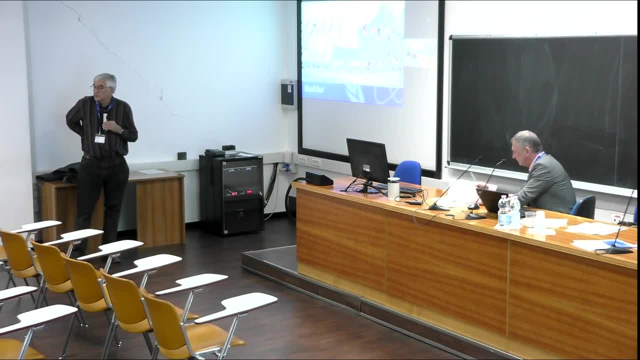 And so we have studied some cavitation and shown that it was uh. if you have a velocity less than 10 meters per second, it's uh. it's okay for sodium, But I have a question for uh, Vladimir, about the velocity of lead. 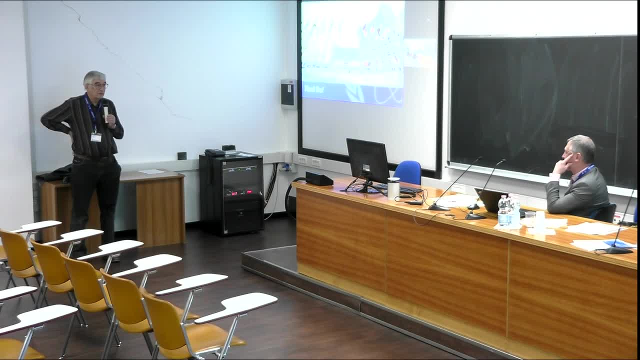 I have seen five meters per second. up to now, in several projects I have seen the limit at two meters per second. Uh, is it because there was some progress on materials, for example? or, uh, they said that it's possible to go up to five and the previous 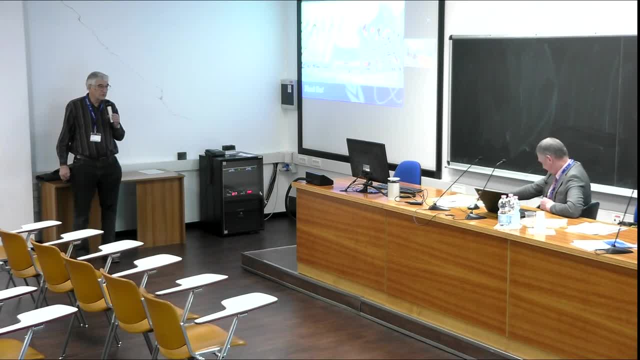 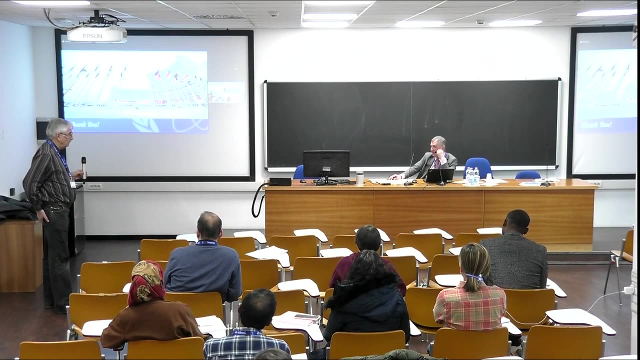 uh, two meters per second was too conservative. How do you? what do you think about that? Thank you for the question. This is, uh, actually opposite. The five meters per second was previous evaluations. Now they become- few years ago- I'm 10 years ago- more conservative and becomes. 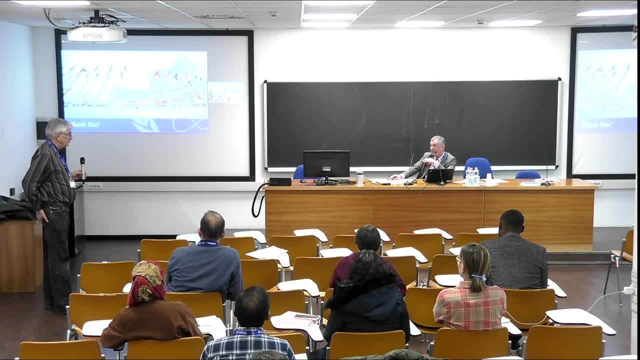 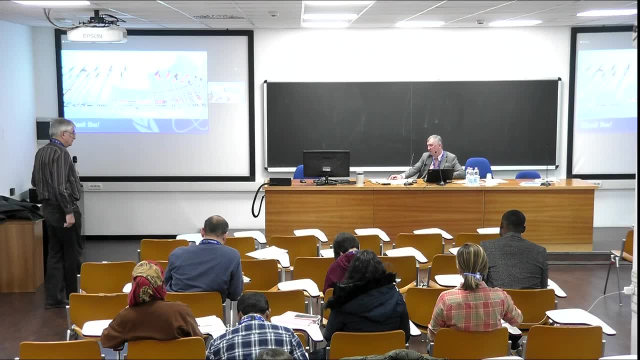 this limit decreases to two meters per second. Now it's two meters per second. for the breath, for example, It used to be- potentially from some evaluations- was five meters per second, but now it's two meters per second. Okay, Not because on the slide it was indicated five. 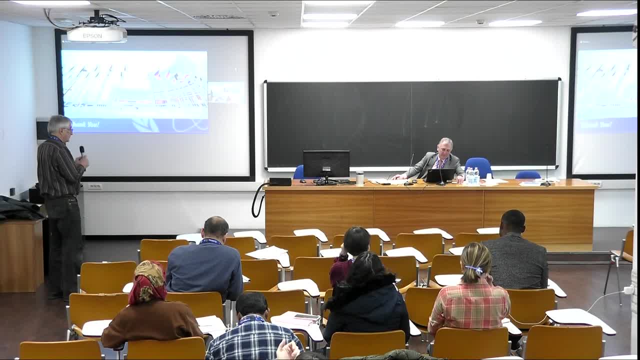 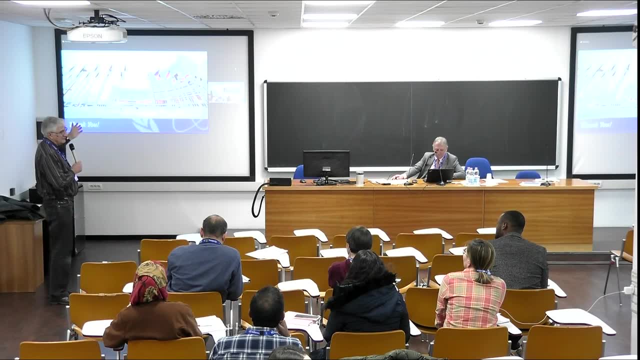 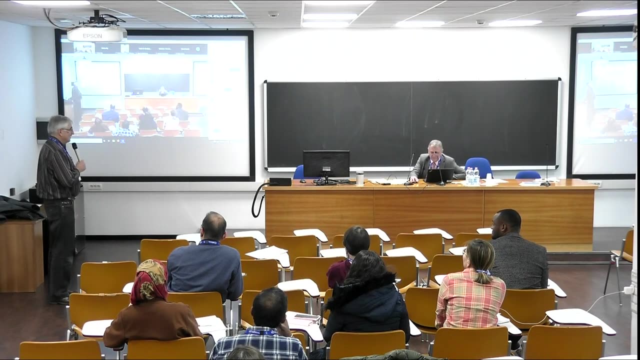 Maybe it's old, yeah, Okay, And a comment about sodium water reaction. There are two key. Effectively it was, I would say. for me it was maybe too positive for lead, And just a comment about the sodium water reaction. 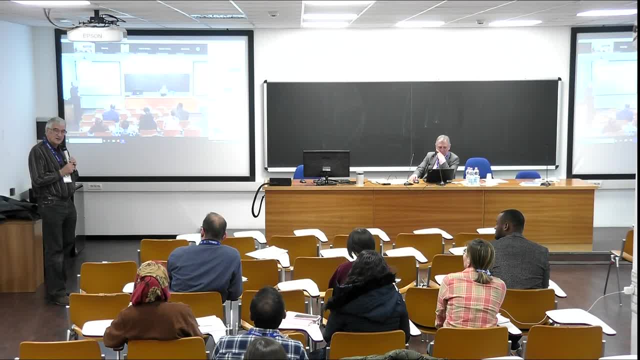 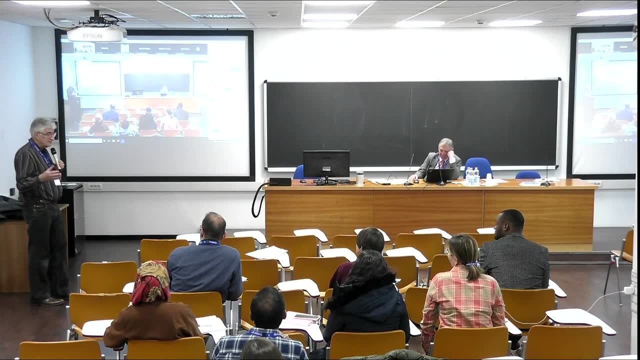 For sodium air interaction. it's clear that it's really a drawback for sodium for fires and so on. We have to take into account this reactivity and it's clear that it's necessary to address this point seriously. It was done in the past. 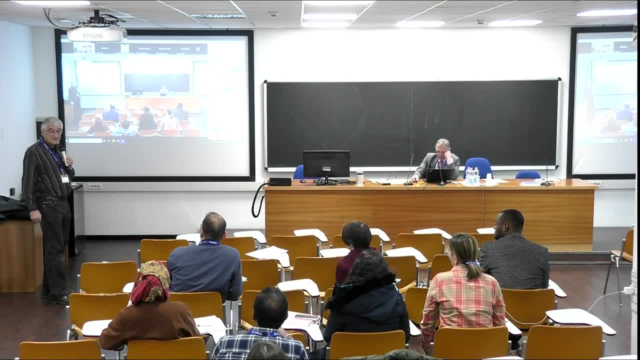 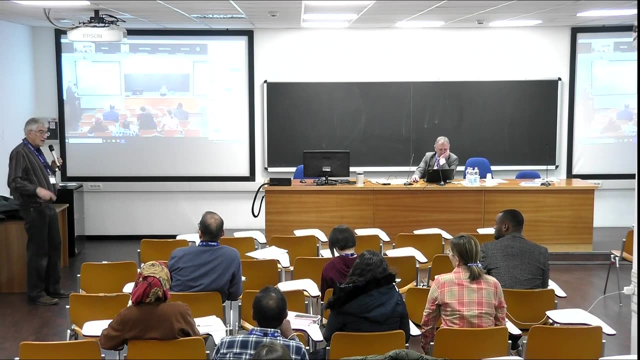 because you know that there were many sodium fast reactors in operation. But about the sodium water, I would say my personal feeling is not a so high drawback as it is often underlined. Why? Because we have effectively this potential interaction, but the feedback. 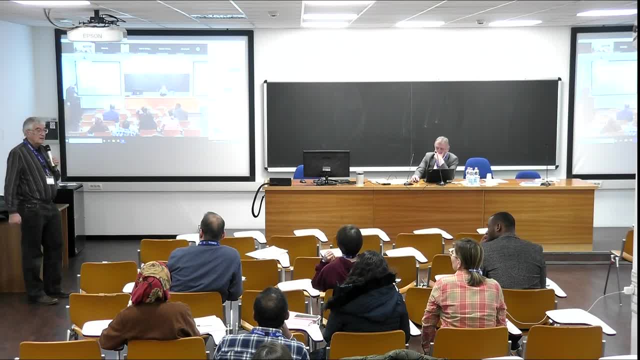 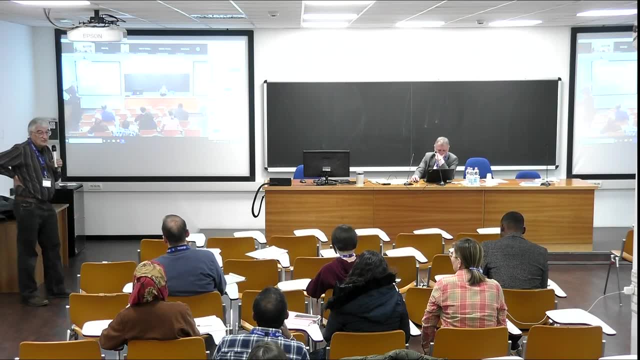 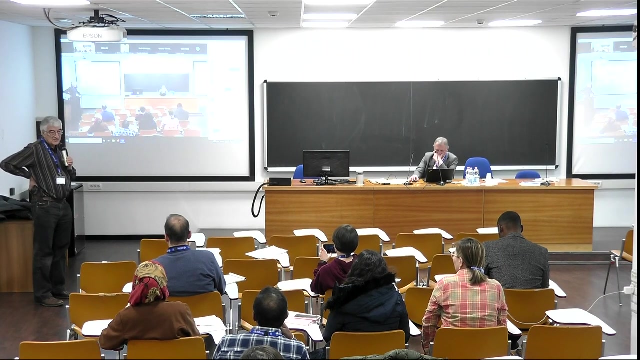 if you look in the feedback of steam generators, for example, except maybe in Russia, in Kazakhstan, BN 350, where there was a large sodium water interaction 50 years ago- maybe we have the possibility to have a sodium water interaction in the reactors without consequence. 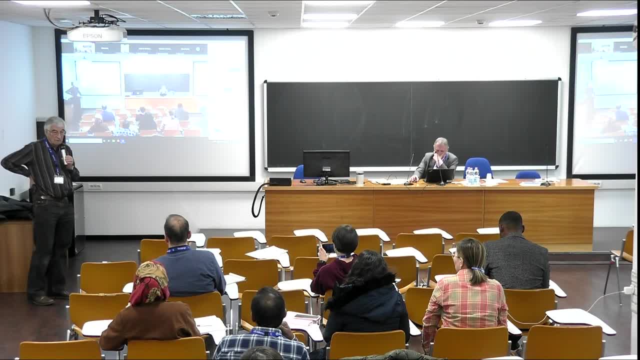 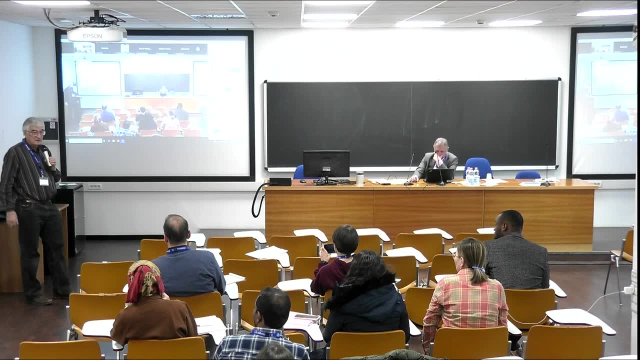 large consequences, Clearly in Phoenix, for example. but now by design provisions we can avoid weak points in the steam generators. This is the first point. Second point: we use the sodium water interaction in two main points for two main act process. 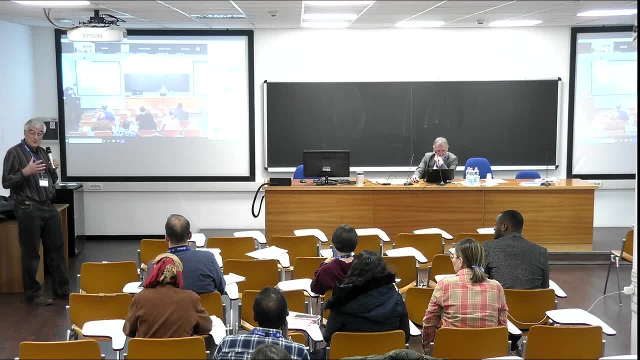 One is the cleaning of components, So it's easy to clean the components with moisture. It applied since many, many years, So it's a positive interaction. I would say This is not the case. This is not the case with lead. 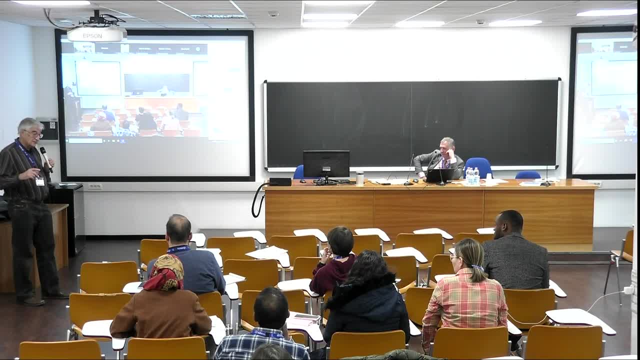 Second point, for the decommissioning, for example for Phoenix, the project is we convert sodium at the end into sodium hydroxide with a process we have developed called NOAA. We convert into soda and then we neutralize to produce water with a salt.